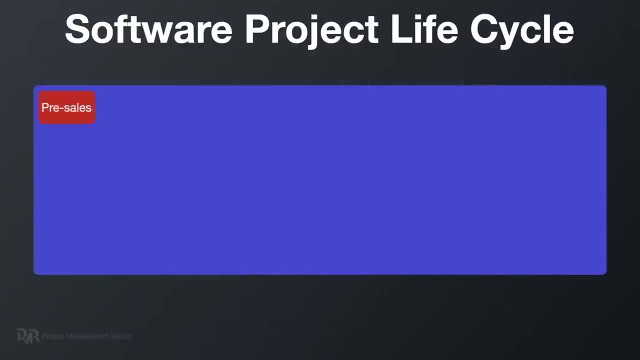 we may have the following phases: Pre-sales project initiation, concept development, prototyping, planning requirements, definition, UI design, development, integration, testing, deployment, hypercare, maintenance and hand-off. closure or support phases. For sure, it's a list of all possible phases. 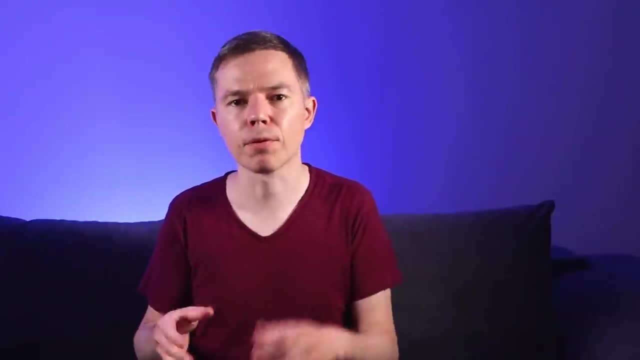 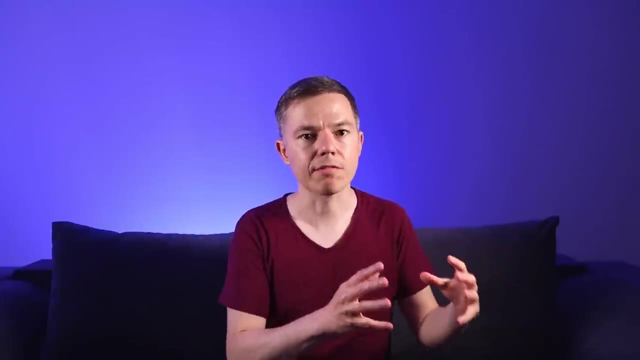 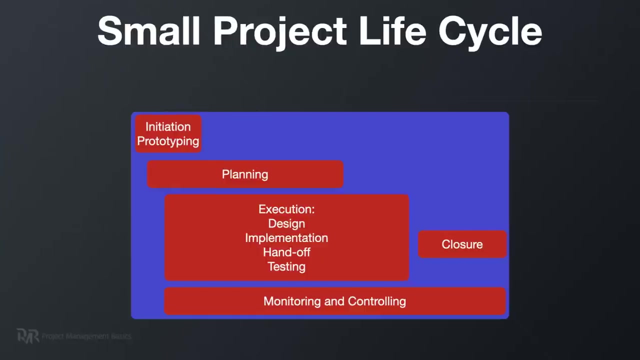 but you don't use them all in every single project you lead, But in any case, on a big project each phase may take several weeks to several months, So you can treat them as small sub-projects On a smaller project. these phases mix together. 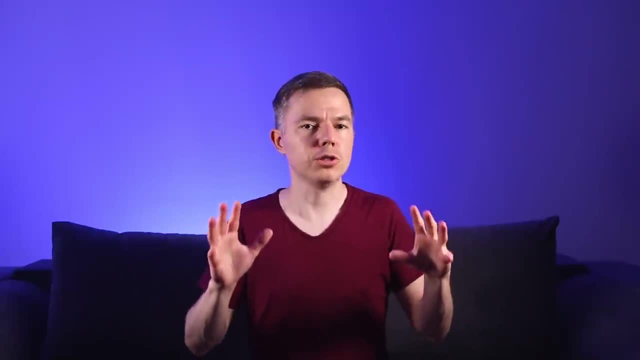 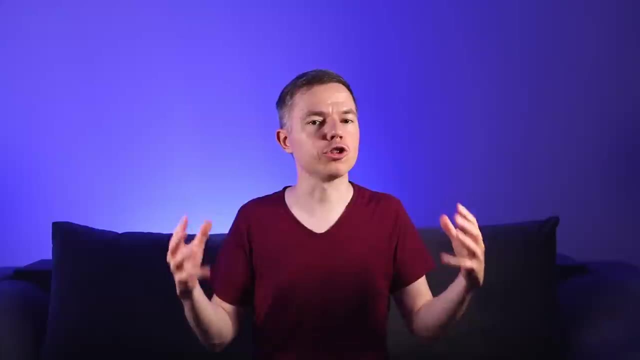 and it's hard to differentiate them. But here's what you need to understand: You can and should use different processes and tools, or even different project management approaches in each phase. For example, you'll use the Scrum framework to manage. For example, you'll use the Scrum framework to manage. 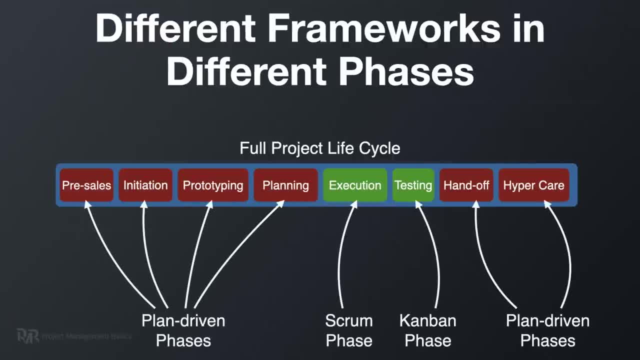 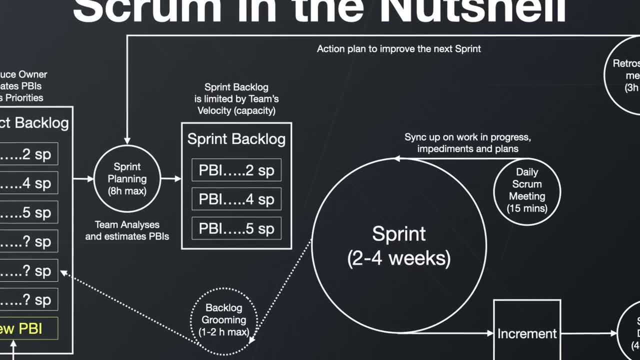 For example, you'll use the Scrum framework to manage the implementation phase of a software project. That's precisely how agile project management with Scrum or Kanban works, But you'll never use Scrum to manage UI design, creation or hand-off phases. 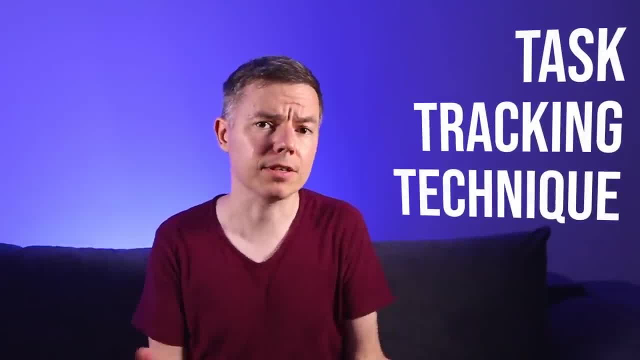 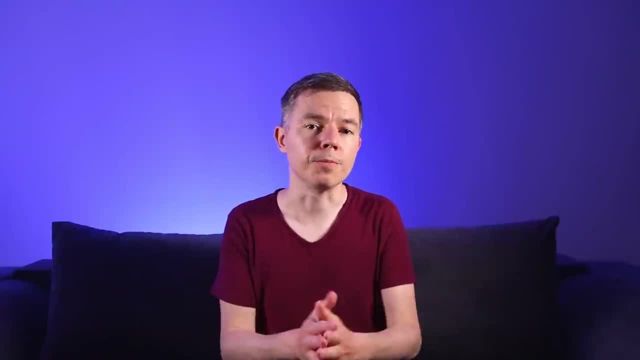 For those phases you'll use something simplistic. For example, you'll track tasks and their due dates. Okay, it sounds complicated, but here's great news for you: If you work in one industry for the most of your career, If you work in one industry for the most of your career, you need to learn no more than two or three typical project life cycles, All right. I want to pause here and stress out the importance of what you learn just now, especially if you are not a project manager yet. You see the industry and niche where you work. 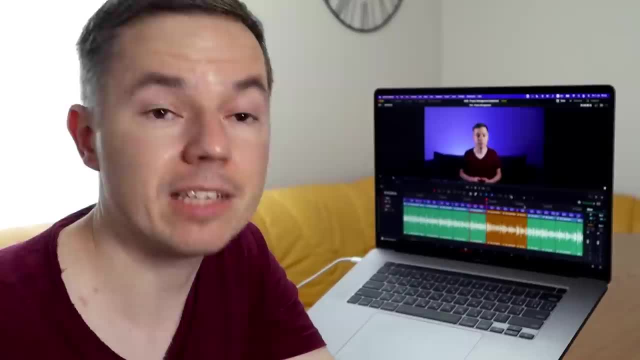 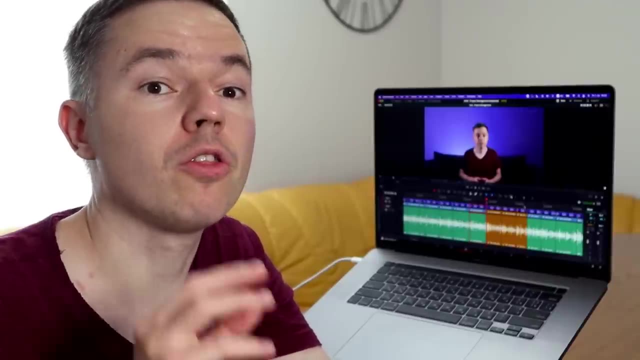 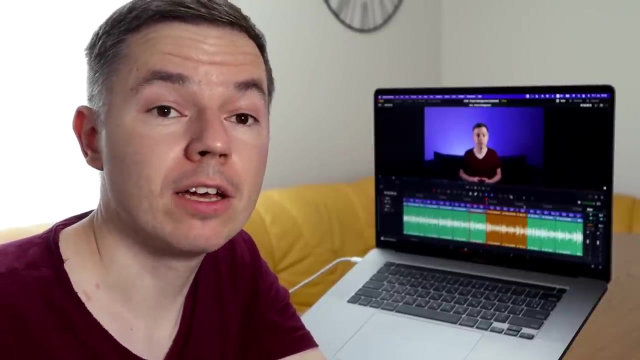 will dictate the available life cycles and project management approaches. So if you already know where you want to work, you need to focus your attention on project life cycles only. You don't need to learn the whole project management knowledge domain. But there is one more limiting factor of your choices. 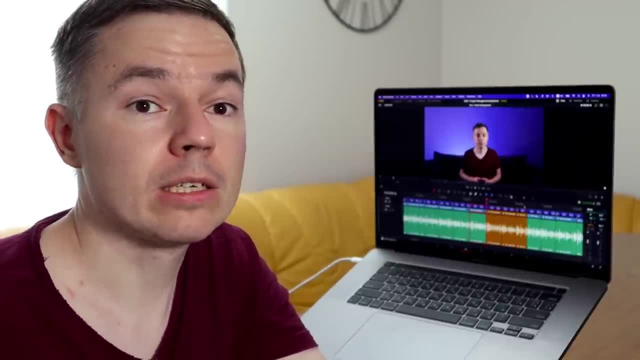 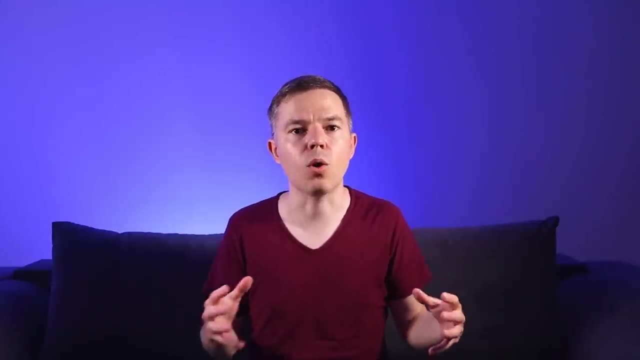 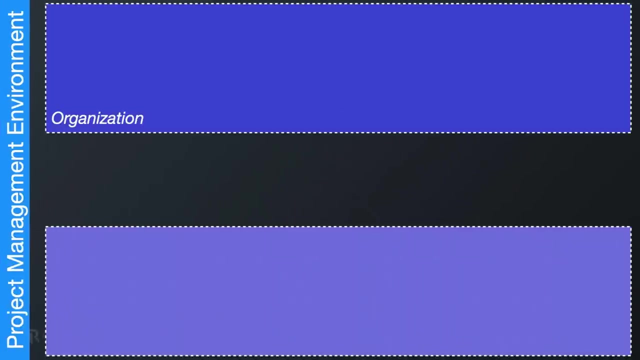 for processes, tools and techniques that you can use. So let's get back and pay close attention to this. You see, you don't run projects in a vacuum. You always lead projects inside environment of the organization where you work. As a result, you always have many custom processes. 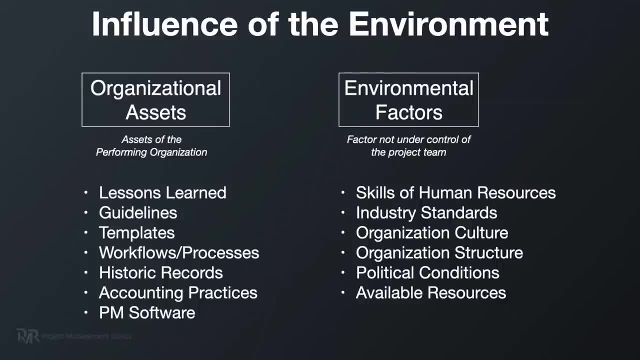 policies and tools. You don't run projects in a vacuum. You always lead projects inside the environment of the organization where you work. As a result, you always have many custom processes, policies and tools that emerge from the organization's business administration. 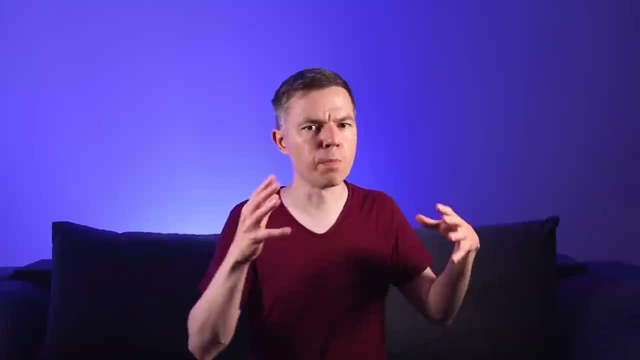 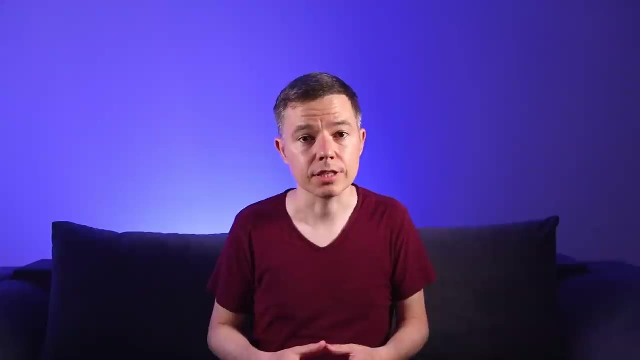 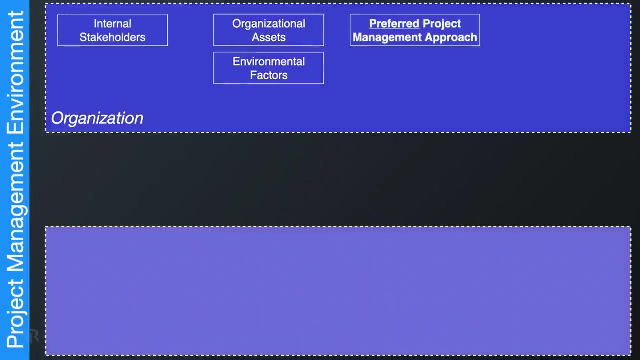 So you can't simply ignore the environment and do project management at your own discretion. It will produce too much friction and inefficiency. So instead you have to play along with the environment In the real world. each company develops its own project management approach based on its needs. 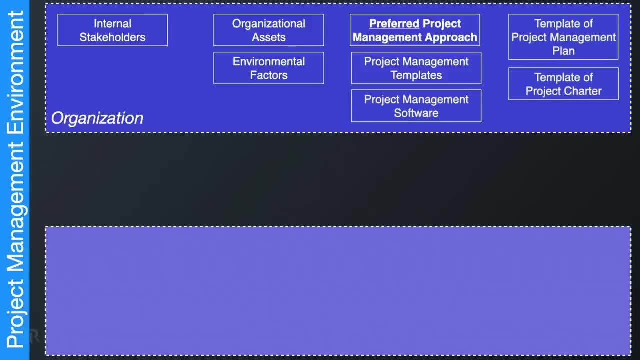 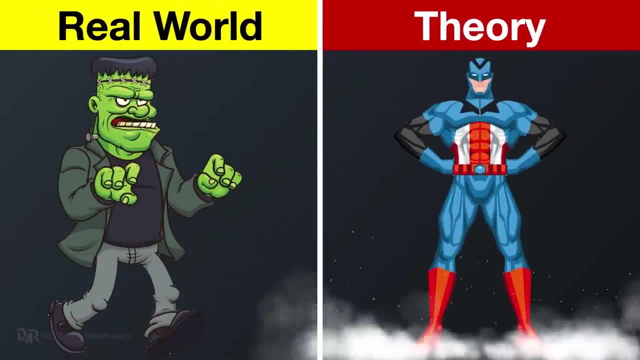 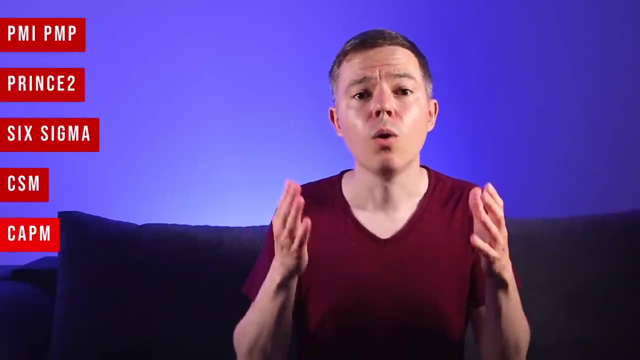 Therefore, there is no such thing as standard project management. That's why project management is more like Frankenstein's monster tailored in one piece, rather than a seamless Captain America. For the same reasons, popular project management certifications won't help you become a better project manager. 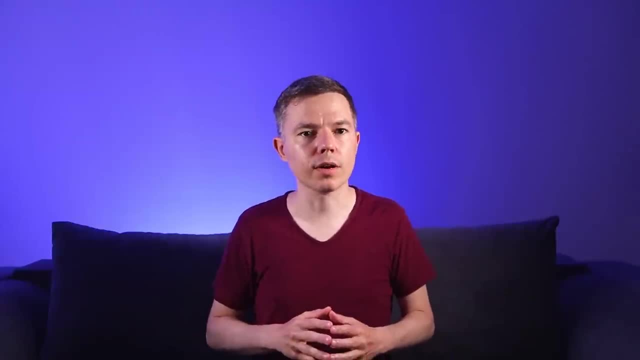 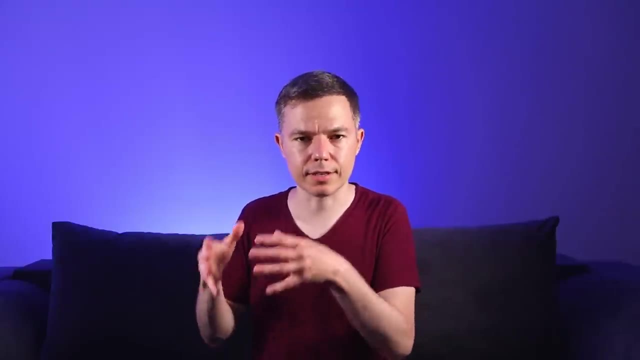 With this in mind, let's consider two cases. First, you work in an organization and you run a so-called in-house project. It's a project for the needs of the organization itself. In this case, you have only one environment to deal with. 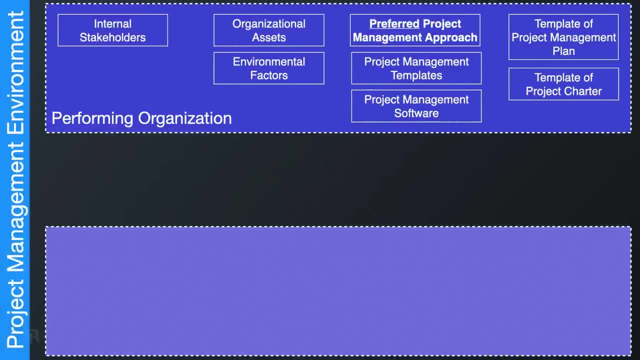 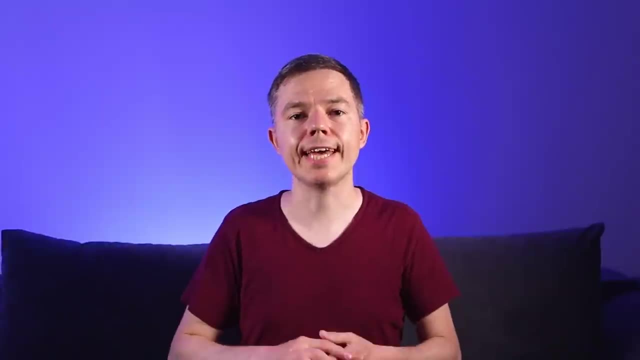 Second, you work in client-vendor relationships. You have your organization, a so-called performing organization, and you have a client's organization. They operate in completely different ways And that's a real-world challenge. You have to take into account the requirements. 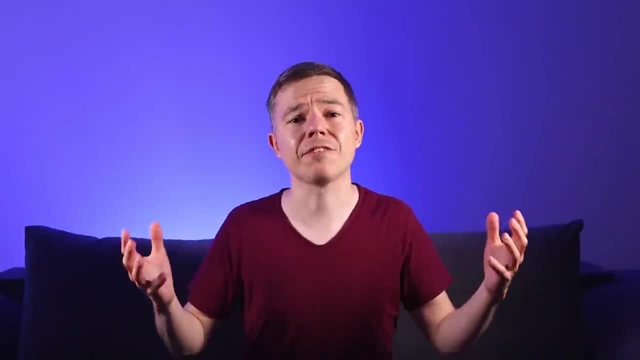 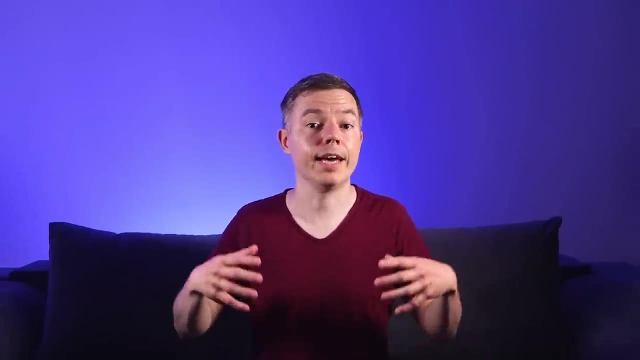 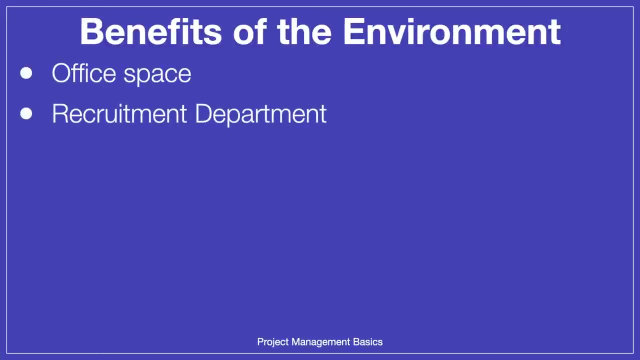 of both organizations to run a project and find common grounds. It includes lifecycle processes, tools, roles, responsibilities and approaches. On the bright side, your environment should provide you with office space, hiring department templates, project management software, lessons learned, best practices from other projects. 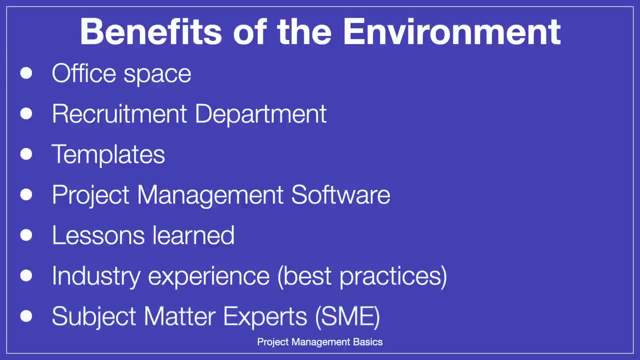 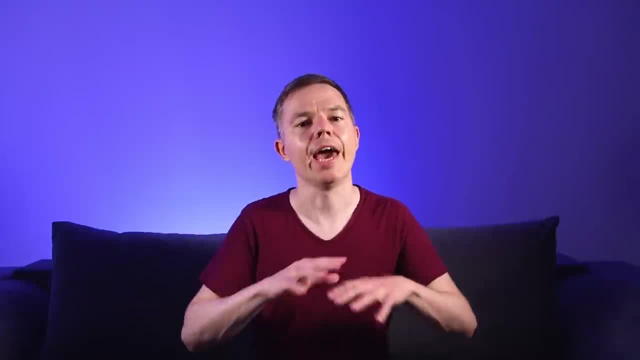 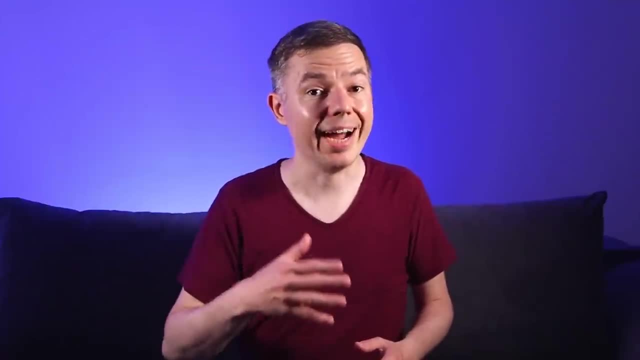 and access to subject matter experts. So in most cases your environment should help you run the project. Usually it takes off the burden of organizing every aspect of the workplace for your team so you can focus on your project work. So again, you should always align. 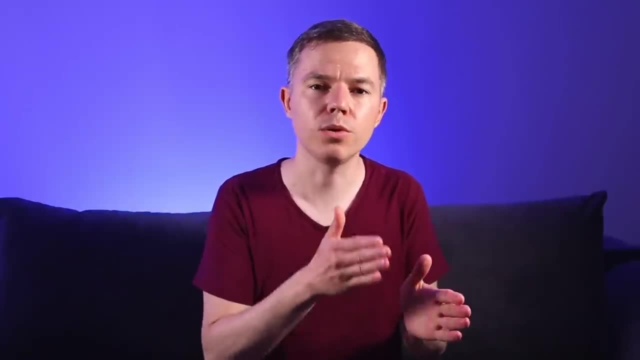 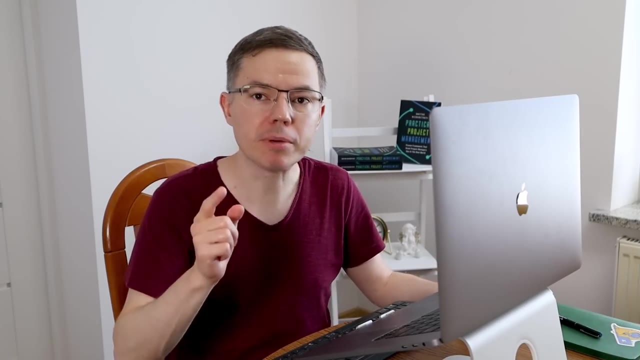 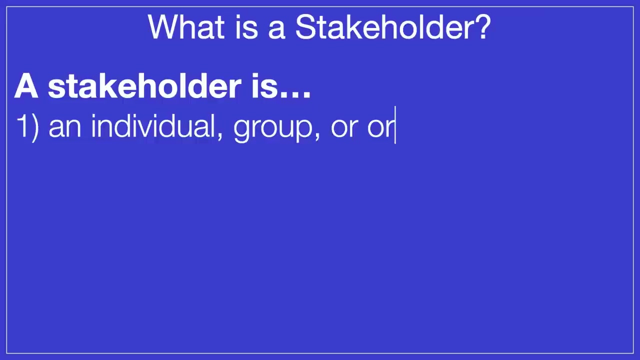 your project management approach. with the environment where you work, It should be like swimming with the current, not against it. And now is a great moment to start talking about project stakeholders. A stakeholder is an individual, group or organization that may affect, be affected by. 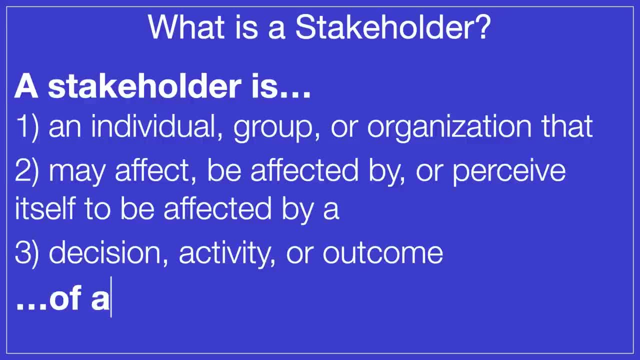 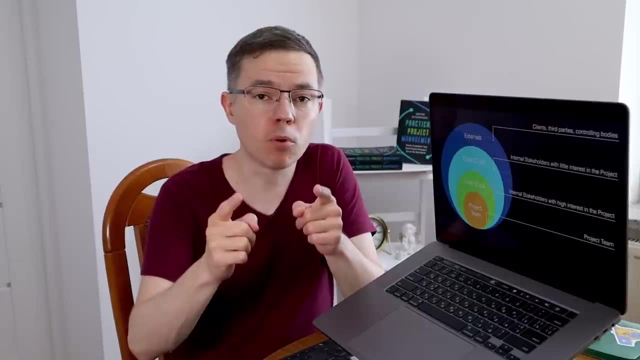 or even perceive itself to be affected by a decision, activity or outcome of a project, according to the definition from the PMI's PMBOK guide. So, in other words, your client, the project owners are your stakeholders, But likewise your boss, some team members. 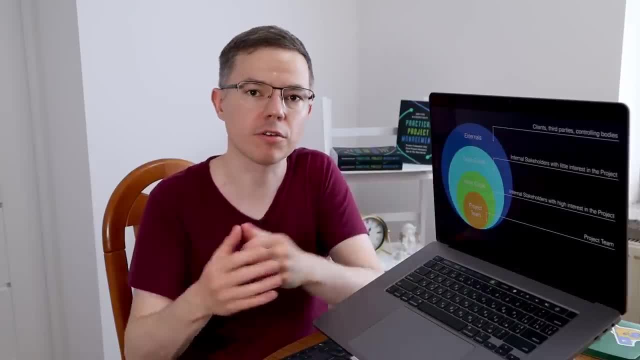 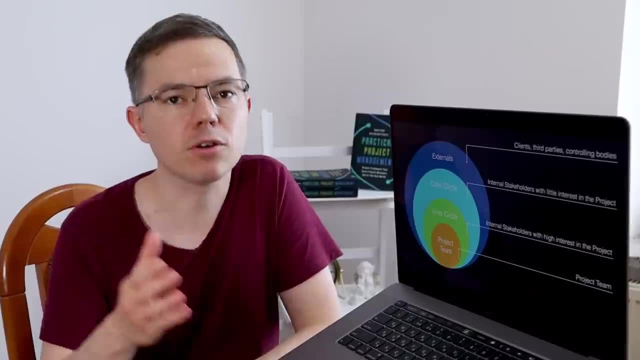 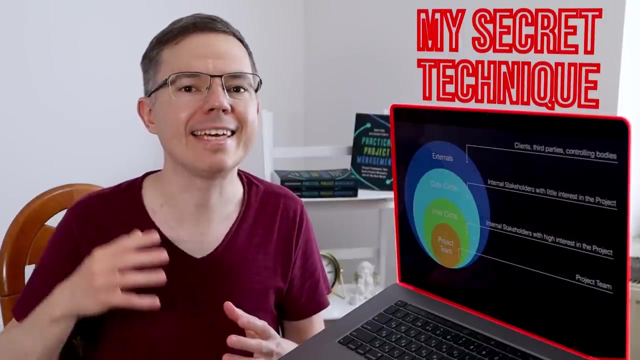 and subject matter experts are also stakeholders of the project. So stakeholders are all possible people and organizations who may gain or lose because of your project. There are many types of stakeholders and many reasons why they care about project, And that's why you need to identify them all. 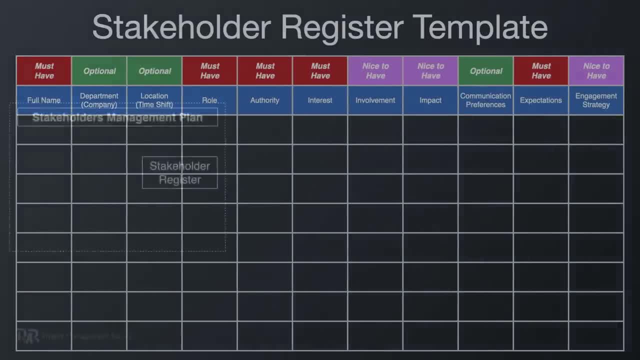 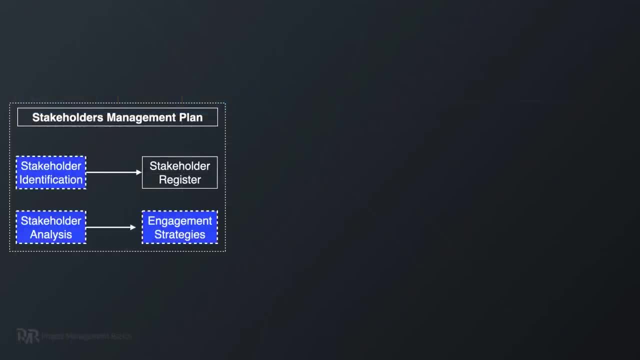 Here you start using a stakeholder register to capture all the information about stakeholders, And then you need to perform stakeholder analysis and decide how you want to interact with each of them. Here's what I want you to remember. Stakeholders provide the recording. 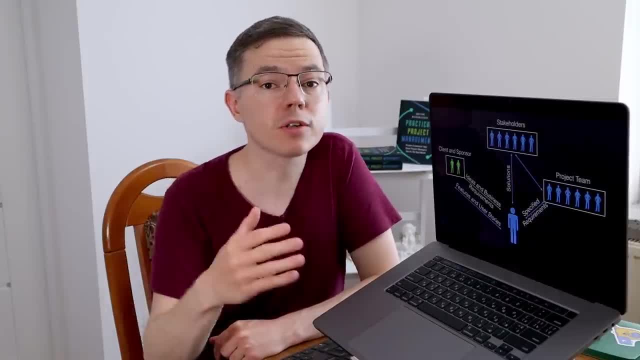 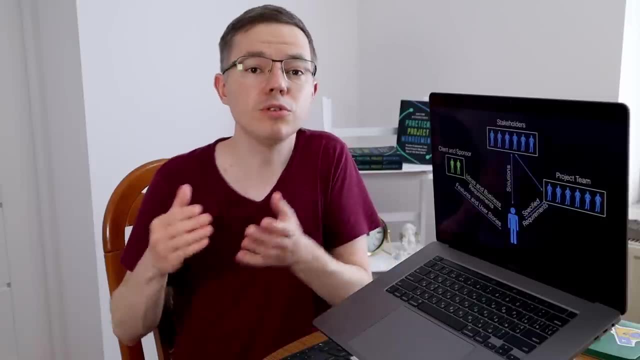 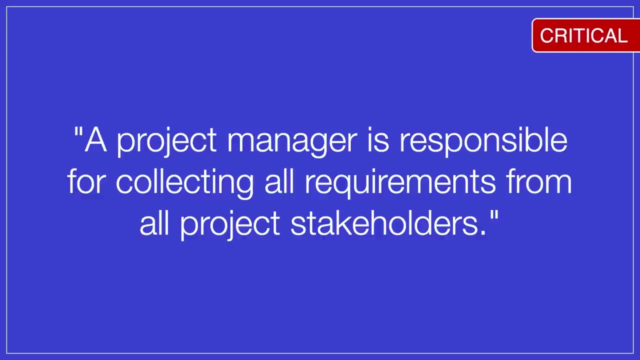 of the requirements. Some of them provide requirements towards the product or service you need to create. Others provide requirements towards your project management approach. they want you to use in their environment, And here's a critical part. It's your responsibility to collect all the requirements. 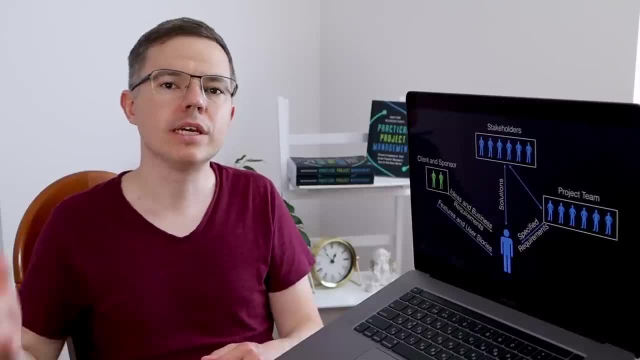 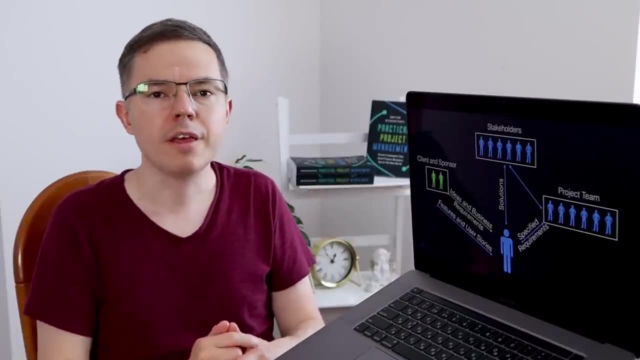 from all stakeholders for your project. In the real world, if you miss identifying important requirements from an important stakeholder, it will be your fault. In the worst case scenario, this stakeholder will use their authority to force you to include the requirements into the project. 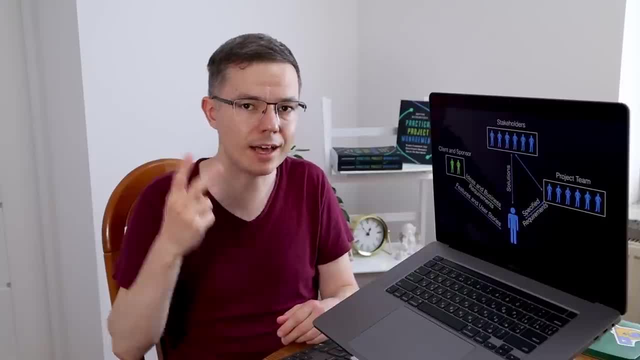 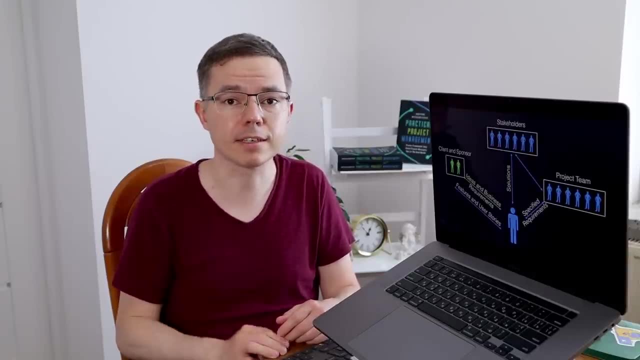 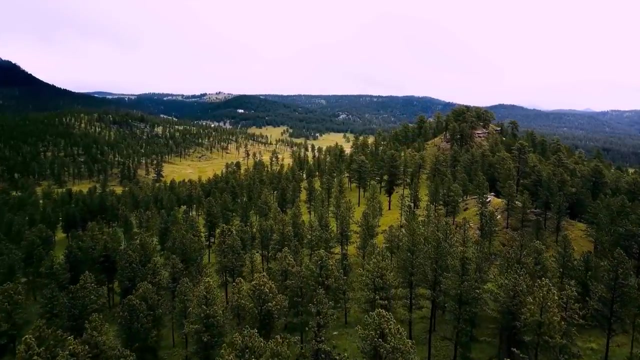 You'll have to change your project management plan, explain to other stakeholders how it could happen and maybe ask for additional budget and time, And usually it's an unpleasant conversation Or even it may put the whole project at risk of failure. So, for example, you have almost finished building. 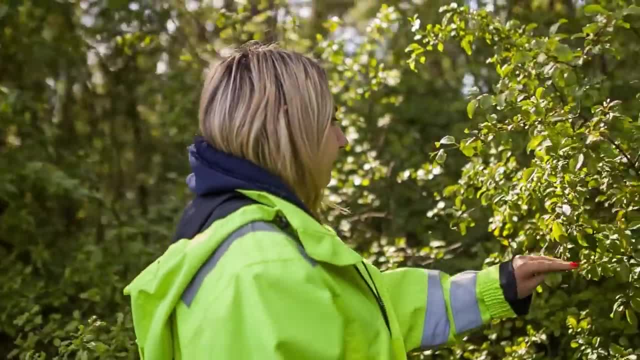 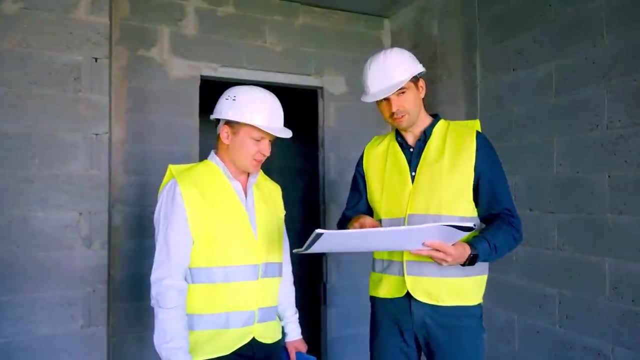 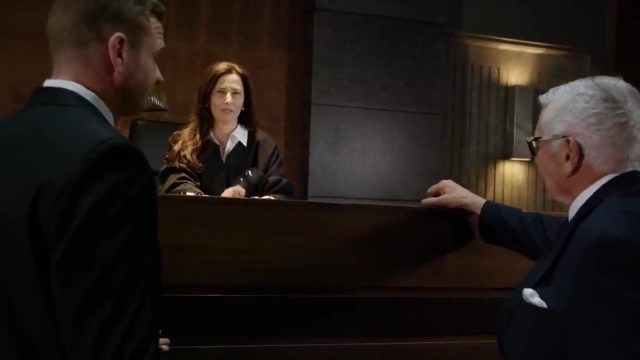 an expensive house in the woods, But somehow you failed to identify an environmental organization as a stakeholder. It appeared your house didn't comply with their environmental policies for this area, which you failed to identify at the start of the project. Now you have to pay a fine and change the heating system. 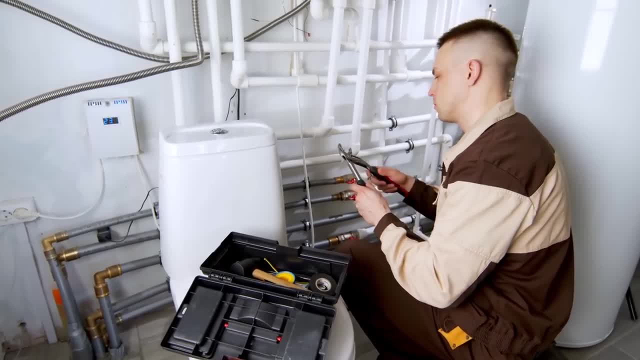 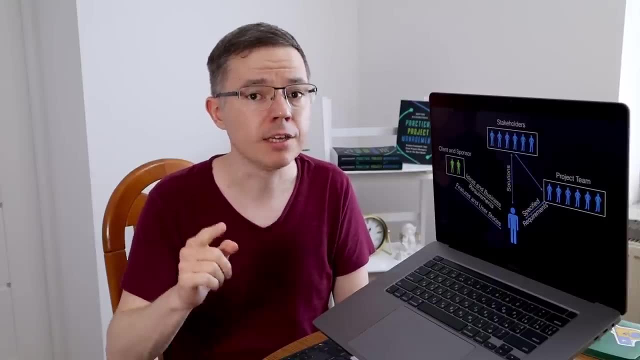 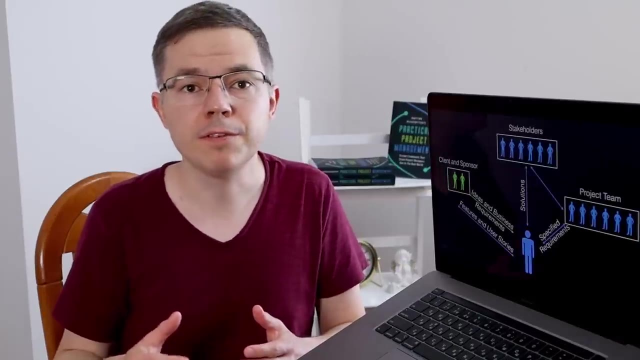 of your house, So it results in additional expenses and rework. You must identify key stakeholders early in the project, But likewise you should be on the lookout for other stakeholders throughout the project's lifetime. In the real world, if you work in a company for some time, 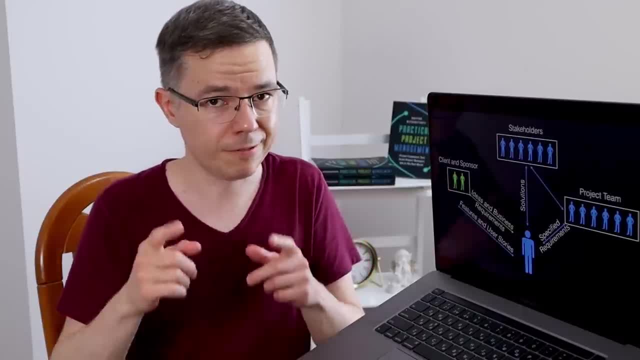 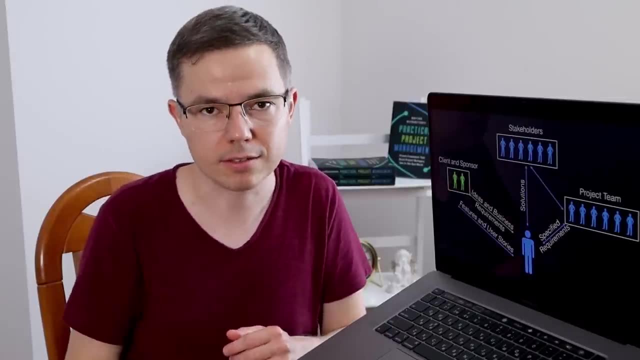 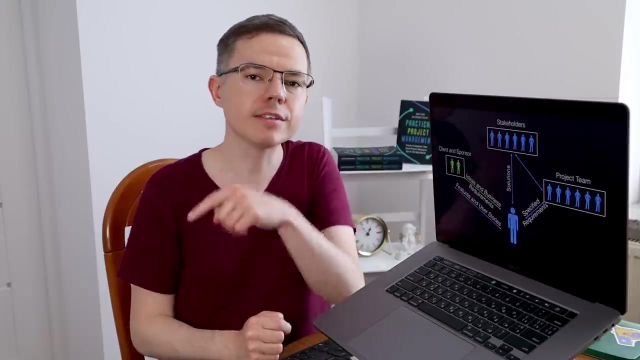 you should already know many internal stakeholders And in fact, you need to continuously build working relationships with them, not only when your project starts And after that. you need to identify external stakeholders from the client side and those from your industry or niche that may impact your project. 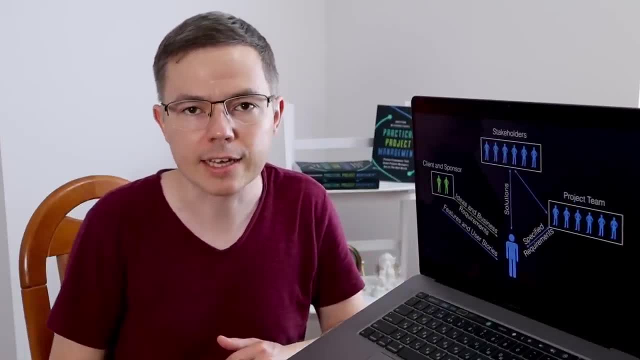 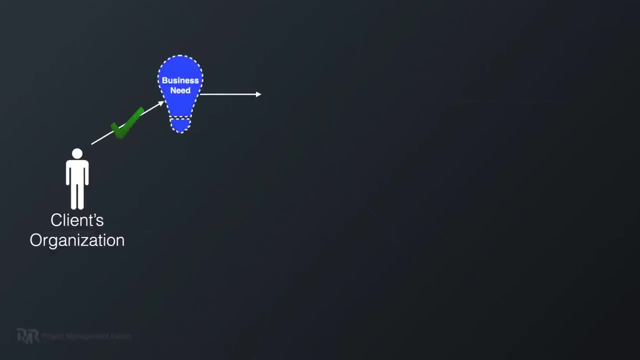 Now we have set the stage for a project to start, Let's get back into the lecture room. So imagine the client's organization. They have a business need to develop a product or service, but they don't have the expertise and human resources to do that. 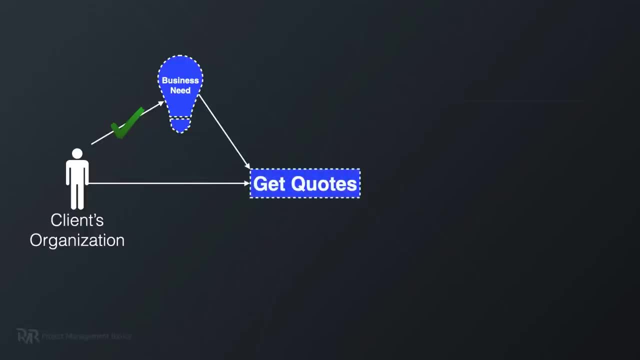 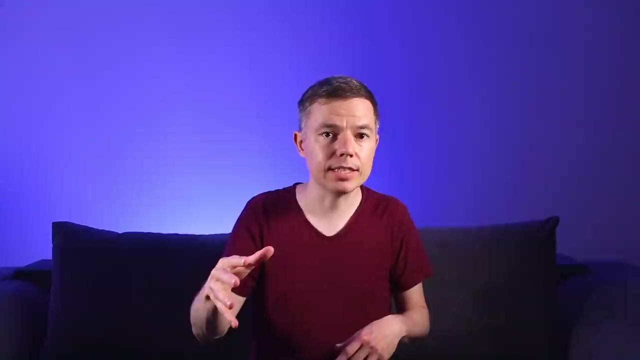 They start searching for a vendor organization that can help. As a result, their representatives contact the sales team in your organization. That's how the pre-sales phase of a project begins. You see, before it gets into the project management realm, the sales team and the client should negotiate the terms. 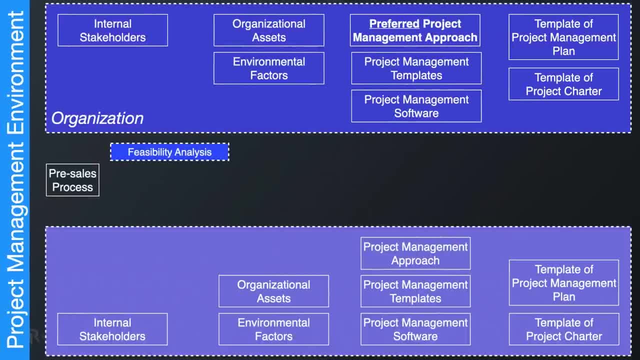 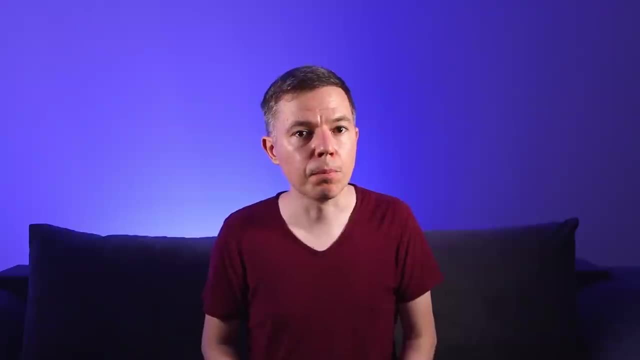 and conditions of a contract. As a project manager you may help the sales team to develop realistic terms. So you may need to perform super high level planning here to ensure feasibility and identify the duration and the budget for the project. Here's a critical point where theoretical books 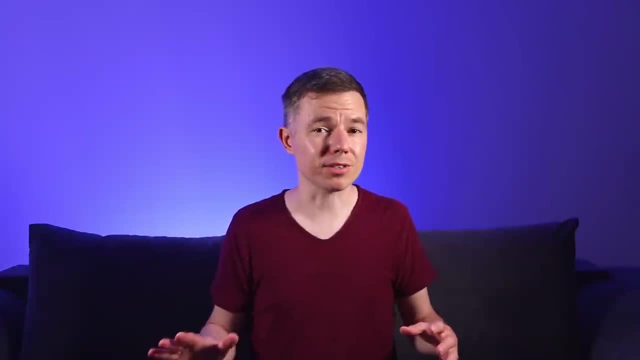 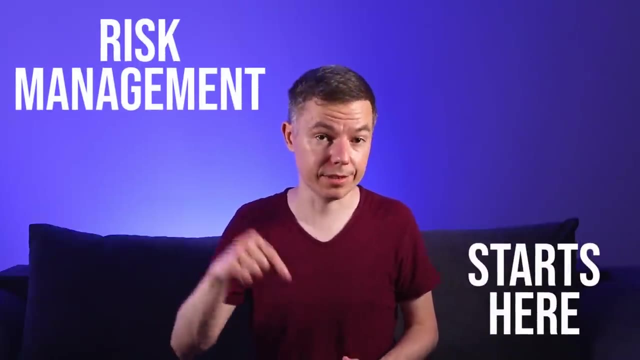 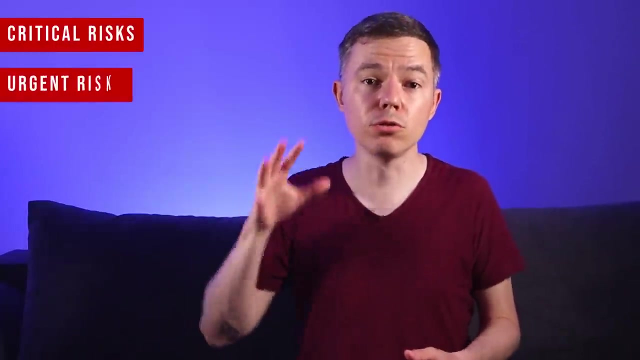 on project management may mislead. you Think about risk management way too late In the real world. you start risk management activities in the pre-sales phase. You may have critical risks right at the beginning of the project. Moreover, there might be urgent risks. 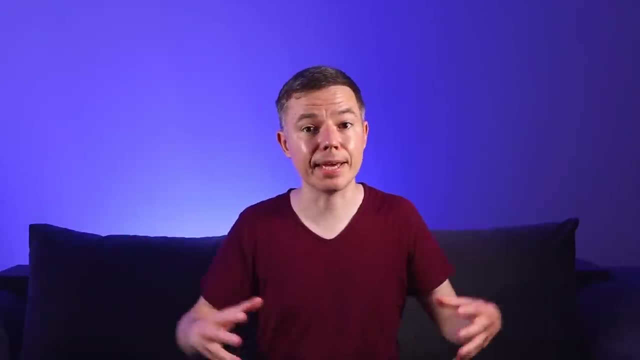 that you need to resolve right away. For example, such risks may embed a problem at the start of the project that will fire up later during the execution, Or it may simply kill the project's feasibility before it starts Because you missed an opportunity. 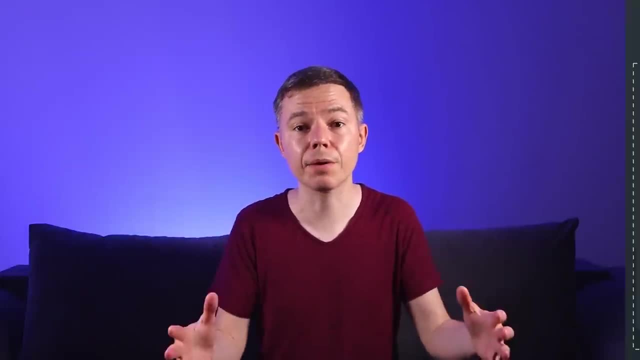 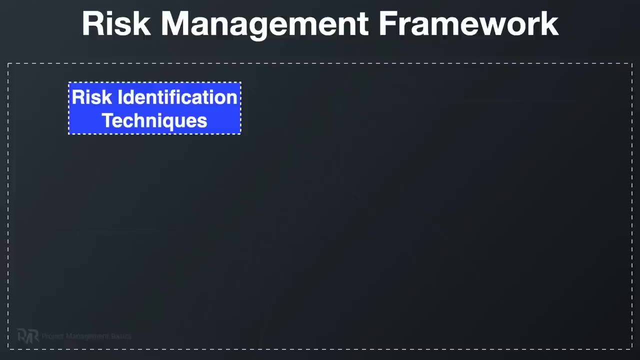 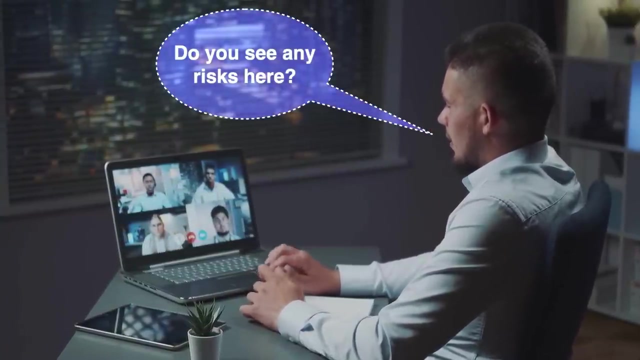 That's why you do risk management continuously, And the framework may be as simple as this one. You continuously apply risk identification techniques in all project activities, And the simplest one is always to ask the team and stakeholders: do you see any risks here? 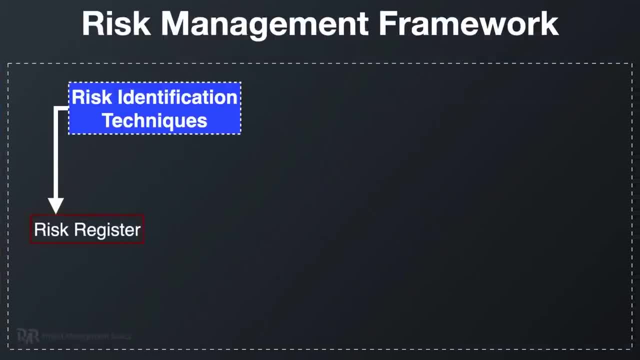 Then you log all identified risks into the risk register. After that you perform risk analysis. You should do qualitative risk analysis. You should do qualitative risk analysis And you may consider a quantitative one in some cases. Then you select several most critical risks. 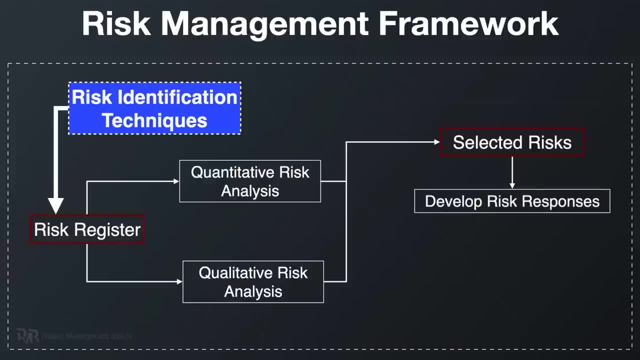 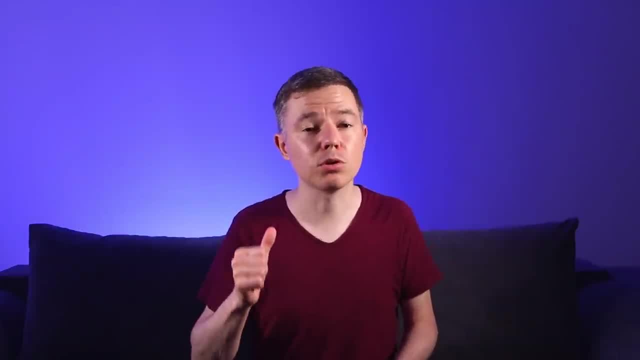 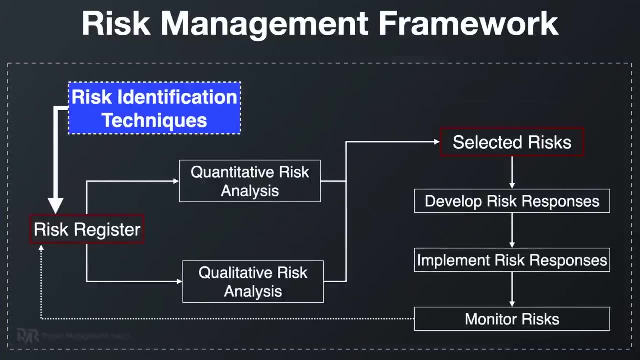 and develop risk response plans based on your analysis. There is one critical concept about creating risk response plans that I'll explain later when we talk about planning. So then, during execution, you monitor risks and implement risk response plans. In essence, this process never stops during the whole process. 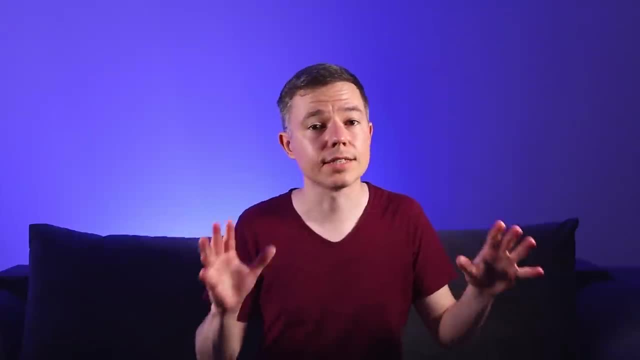 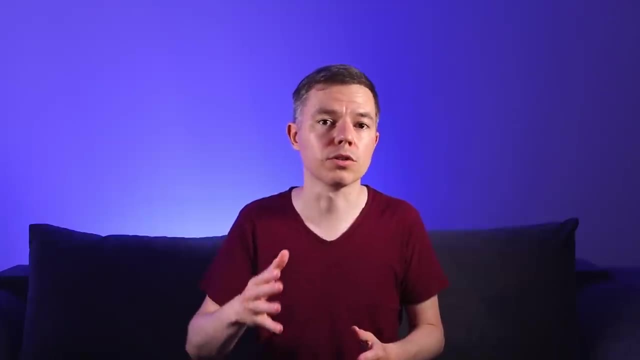 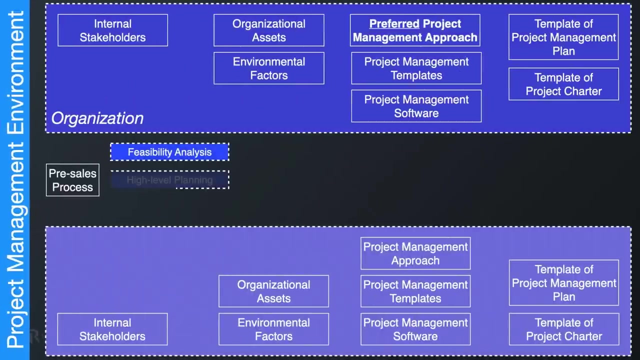 During the whole project lifetime. But again, in early stages of the project you usually focus more on identifying risks And you are always on the lookout for those urgent and critical risks that can ruin the project. But let's get back to the pre-sales phase. 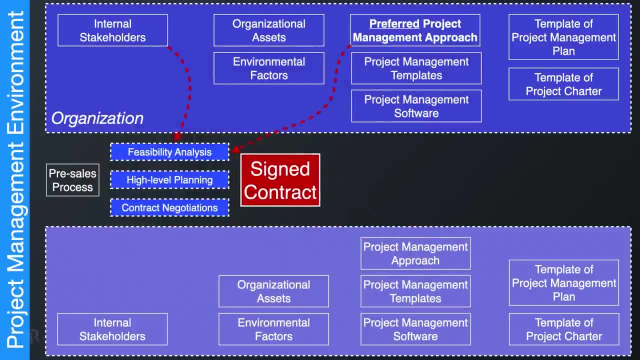 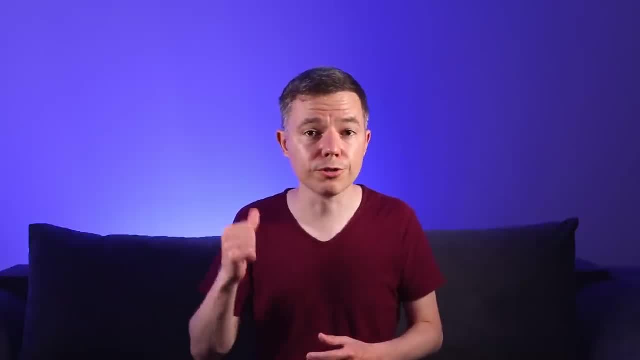 Again, the outcome of this phase should be a signed contract with the client. Quite often clients talk about their real goals for the project during the pre-sales phase, for the project during the pre-sales phase. But here's the catch: Usually a contract doesn't include 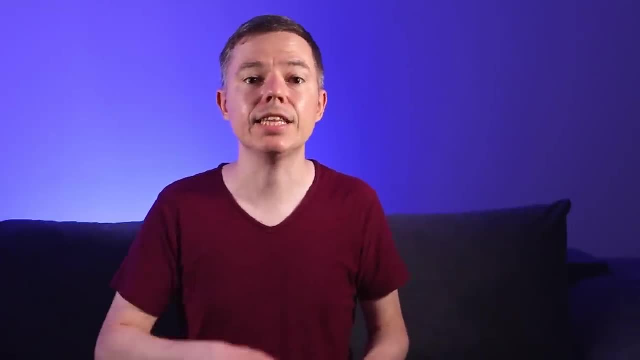 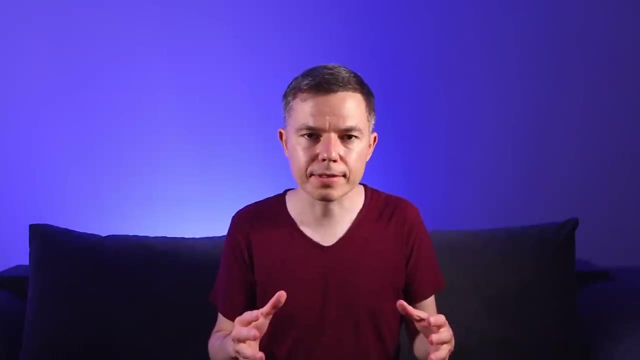 all those details of a project. Instead, it outlines only the overall business relationships between our organizations. If you don't participate in this phase, you need to find a way to get access to the notes, emails and agreements that were made here. 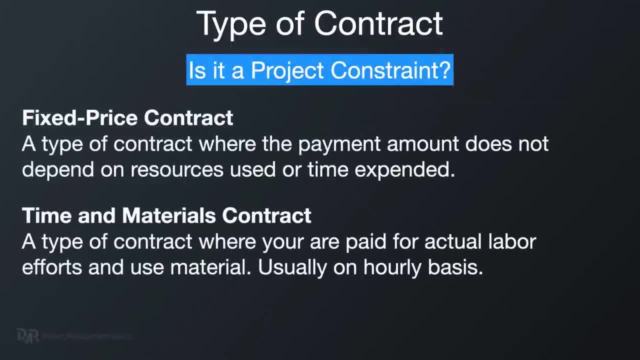 On the other hand, a contract may have a strict deadline or total budget. on the other hand, a contract may have a strict deadline or total budget. It's a constraint for you, so you should know about it In any case, whether you participated. 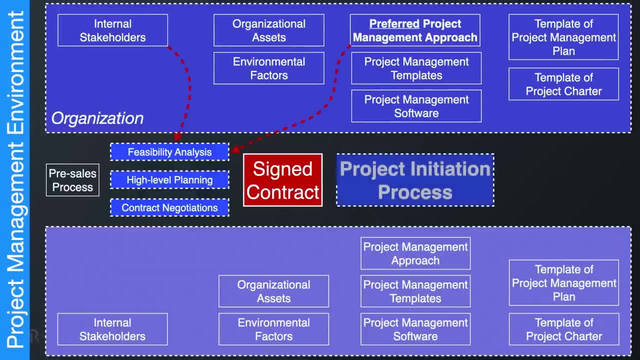 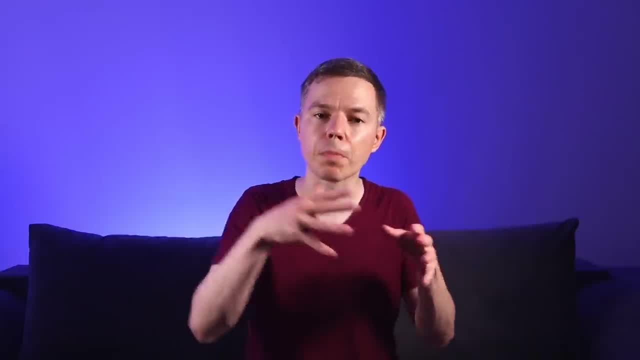 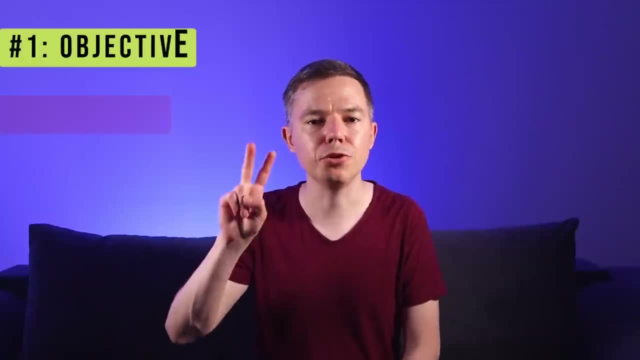 in the pre-sales phase or not? next, you need to initiate a project. It's a transition from the sales and contract negotiations into project management And, as you remember, from the definition, we need to identify three things: The business objective. the unique result we are going to produce. 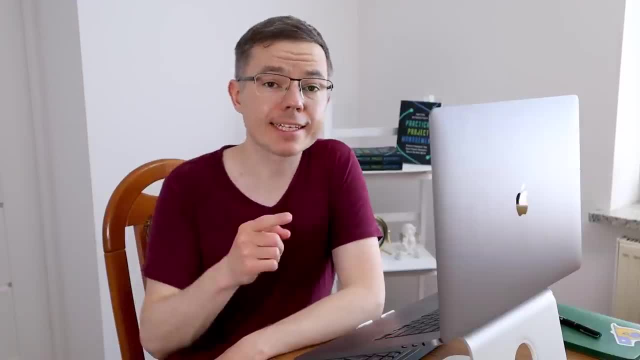 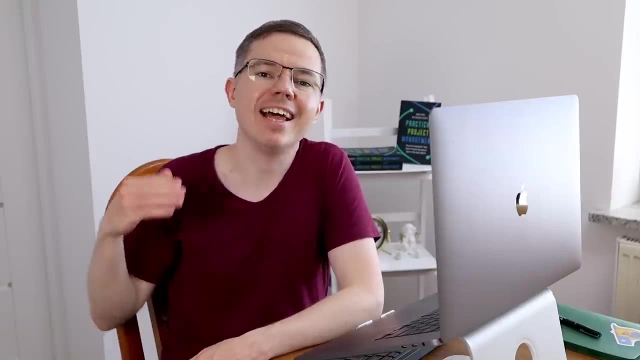 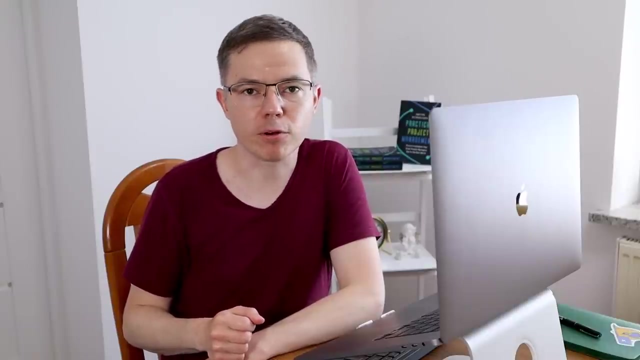 and the boundaries of the project. And in practice, to initiate a project, we use a tool called a project charter. So the project charter includes high level information about the project And we need this information before we start planning process. Project charter is a simple text document. 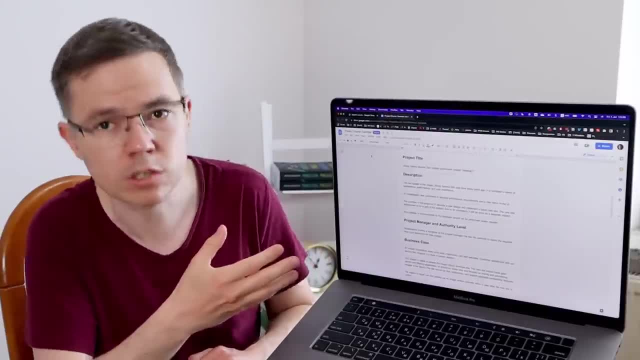 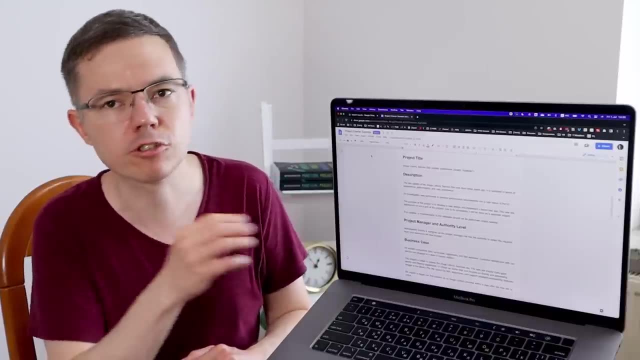 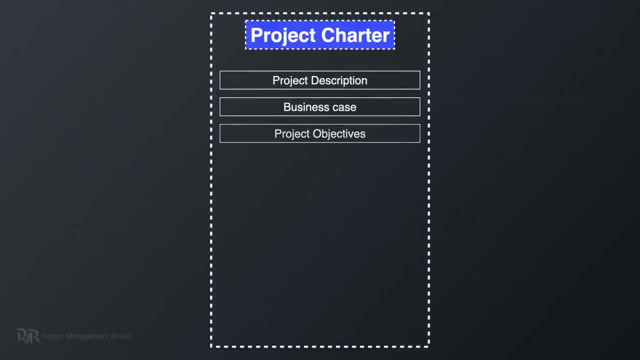 You can use it in Word, in Google Docs or in email if you want. I also recommend that if you use a project management tool, keep the project charter right inside there. A project charter usually includes project description, business case, project objectives. 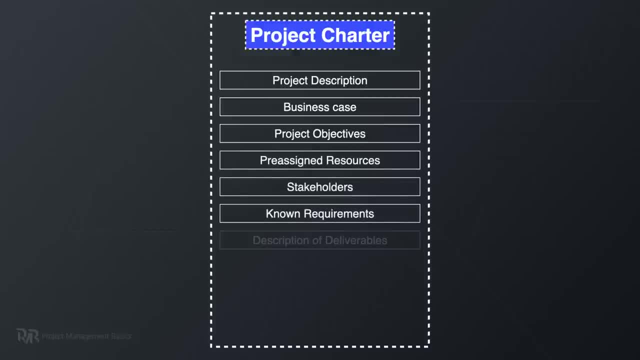 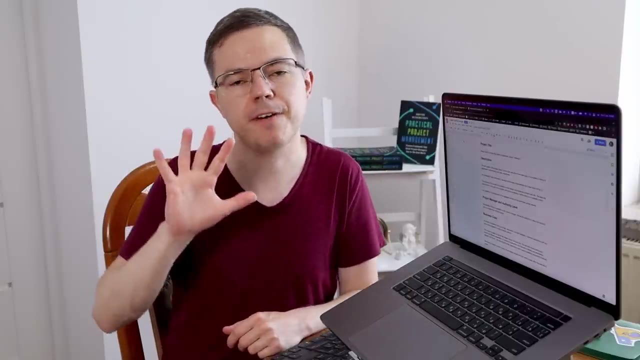 pre-assigned resources, stakeholders, known requirements, description of products, services and major deliverables, assumptions, constraints and project risks. Keep in mind that it's not a comprehensive description of the project. The project charter should be no more than five pages long. 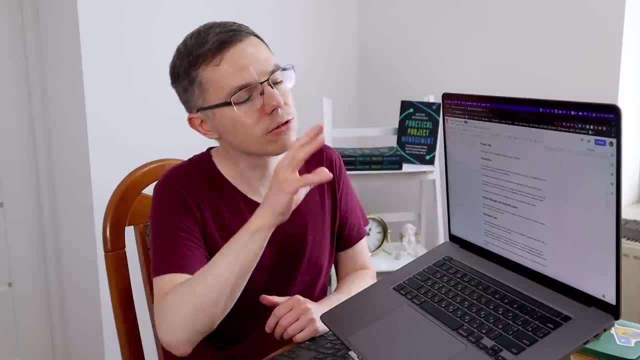 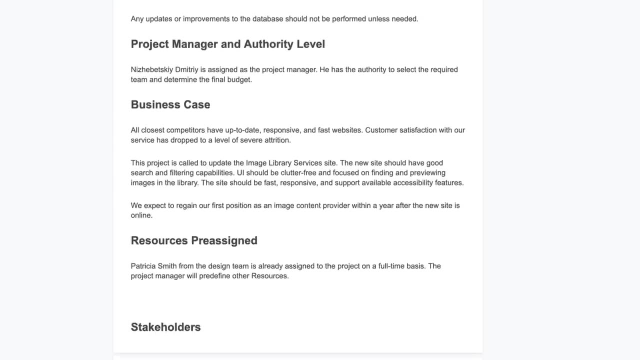 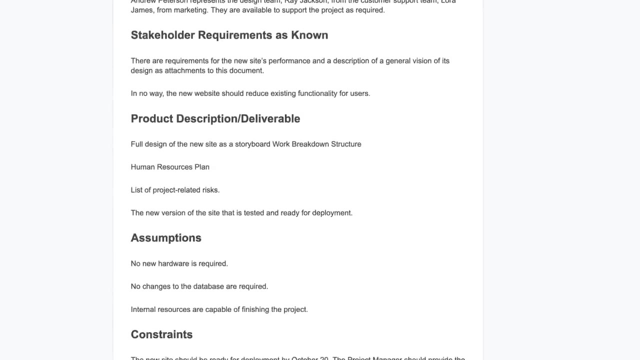 The shorter the better. you may need to create a formal document, But in most cases you simply collect this information and talk through it with your project owners. So you need to develop a common understanding of the project. It's critical because in the process, 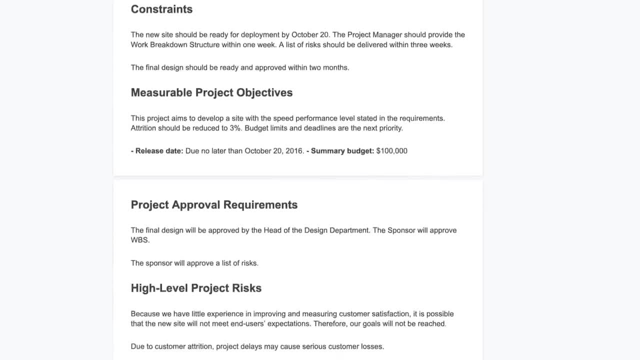 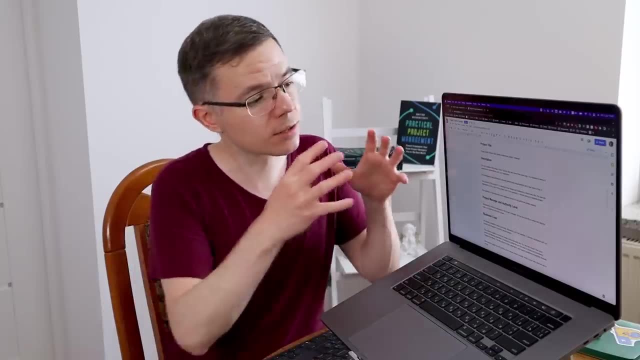 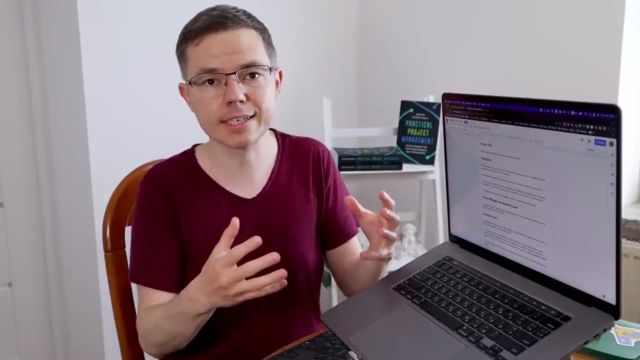 you remove lots of miscommunications right at the start And also you begin to control the client's expectations. You do it by showing what's in the scope of the project, What are the boundaries of the project And whether the constraints look realistic to develop the results that were outlined. 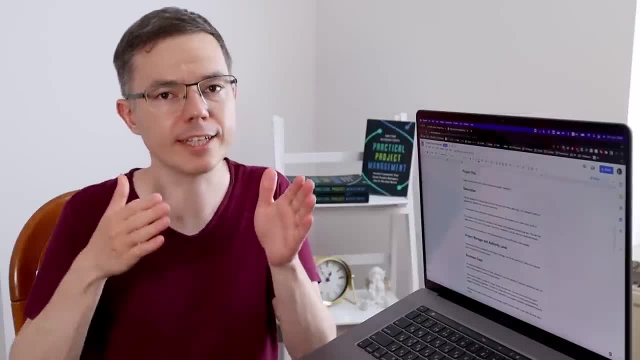 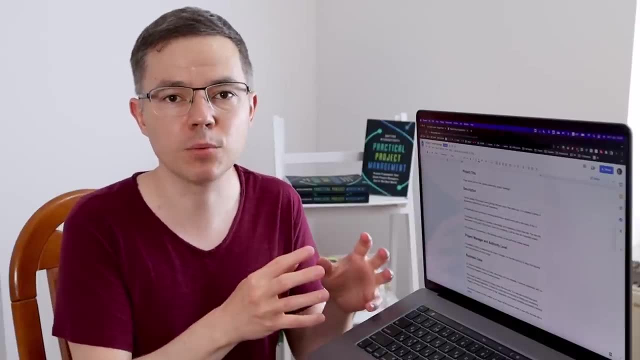 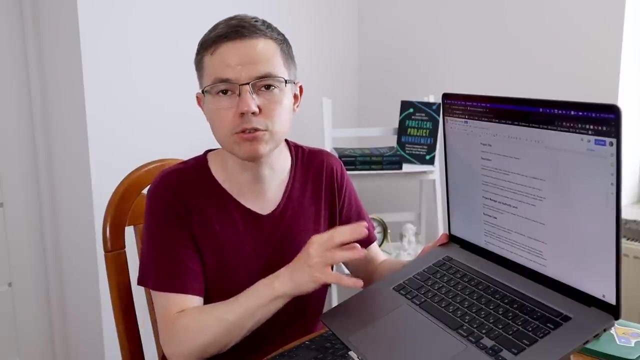 in the project chart. But what's even more important, you should align all your future efforts with the project chart. You need to question everything that doesn't align with the project goal or business case in this chart. Now let me show you why it's so important. 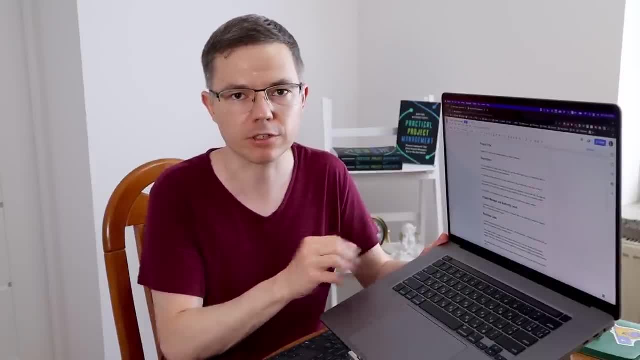 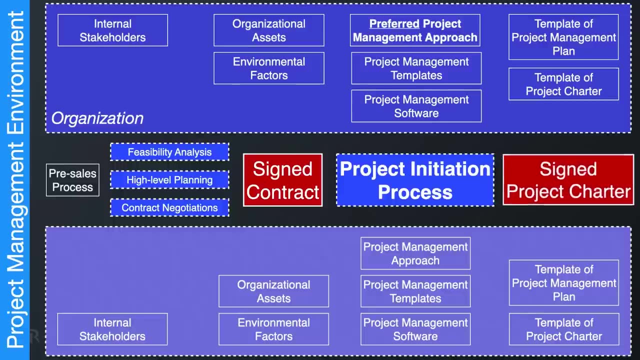 to have a project charter and how we use all this information. Okay, After getting a sign off on the project charter, you need to pause. Take a broader look at the project charter contract, your clients, your environment, available tools, processes and templates. 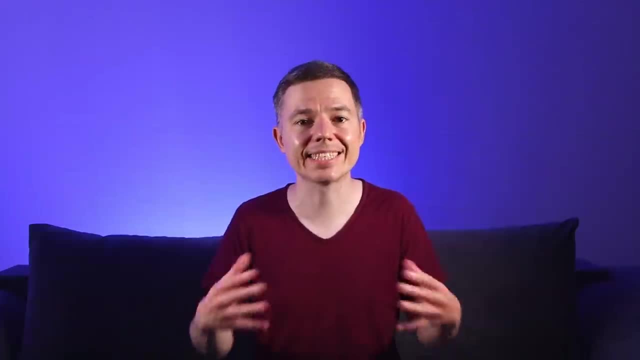 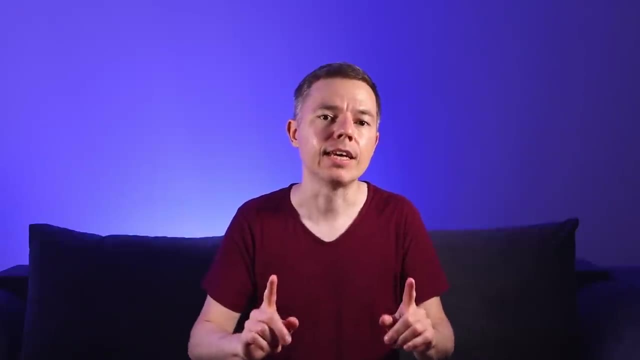 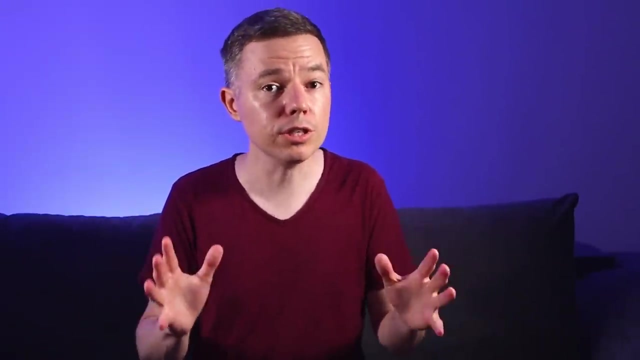 and everything else at your disposal. Now you must decide what project management approach to take and what frameworks to use. But again, it's all based on the project life cycle, So it's not like you need to invent something new. You'll need to choose from one, two. 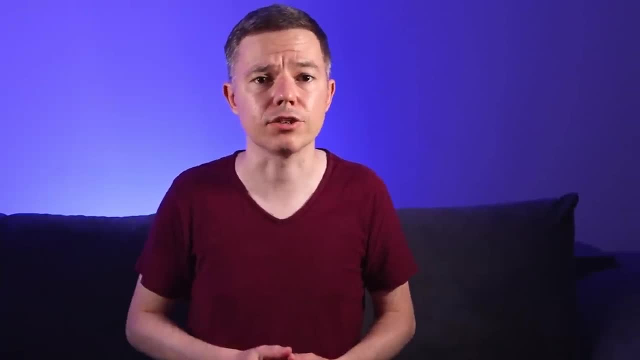 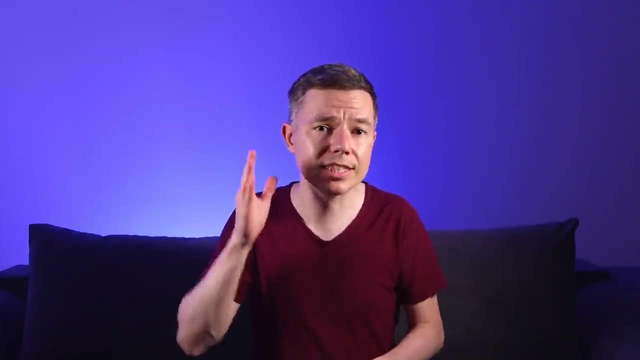 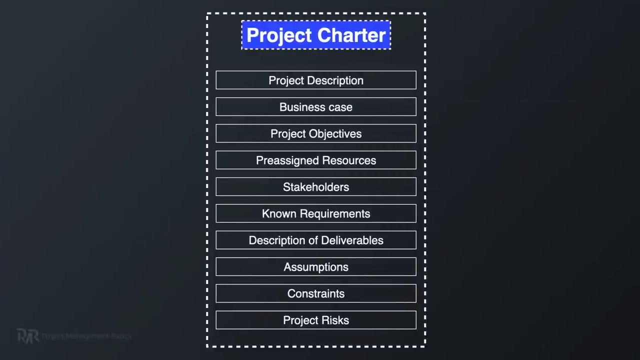 maybe three available options in your organization. Then of course you'll need to adjust them a bit to the needs of a project, But in most cases you'll simply follow the organization's established project management approach as is. Next you need to outline a project management plan. 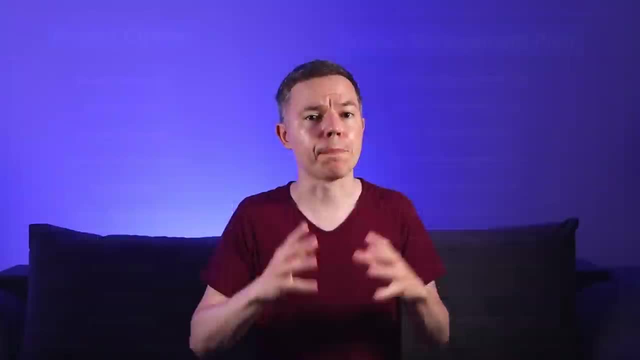 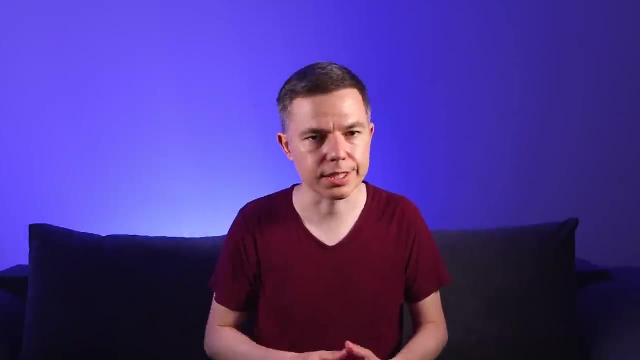 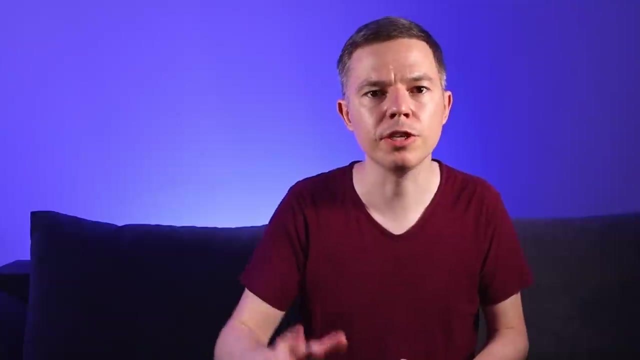 And I want to stress this out once more. A project plan may be a mandatory document in some industries, So it should contain all the details, But the majority of projects don't need a fully written plan, So it's totally fine to keep it all in your head. 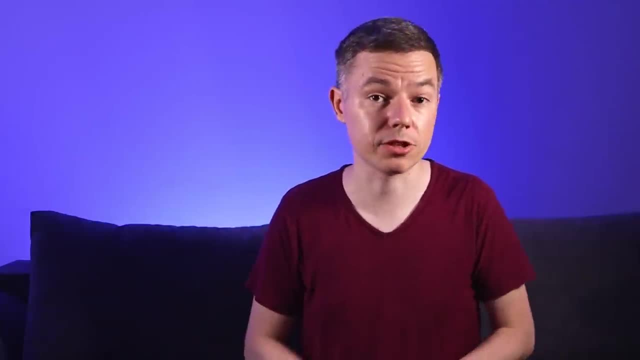 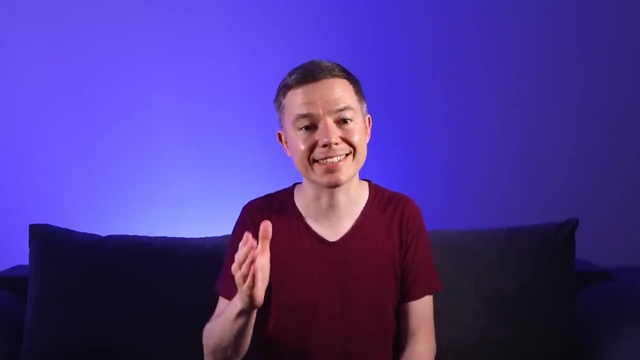 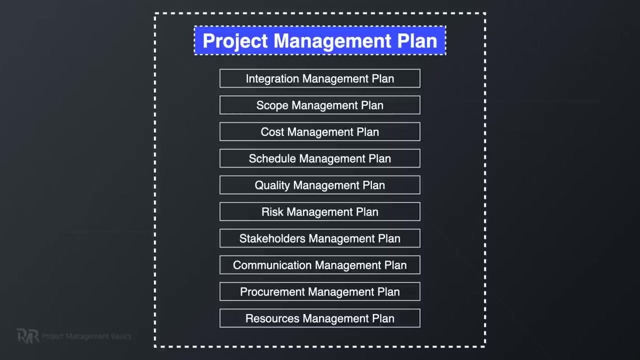 until all stakeholders understand how you manage the project. However, if you have never created a formal project management plan, I recommend doing this exercise at least once. So take the major project management knowledge domains that PMI describes: Integration, scope, time, cost, budget, quality, risk. 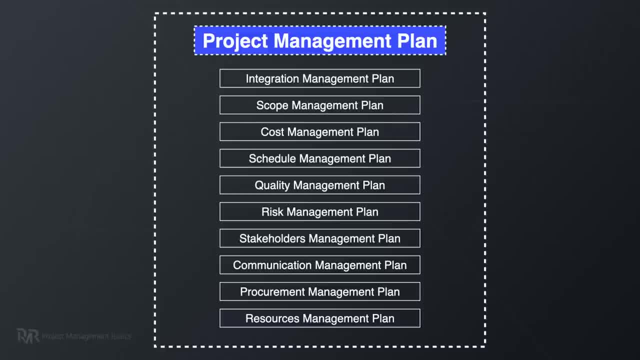 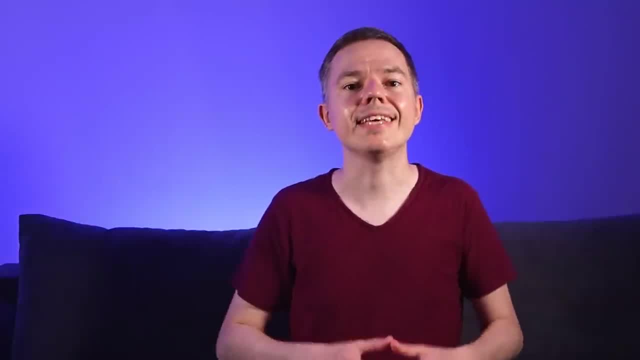 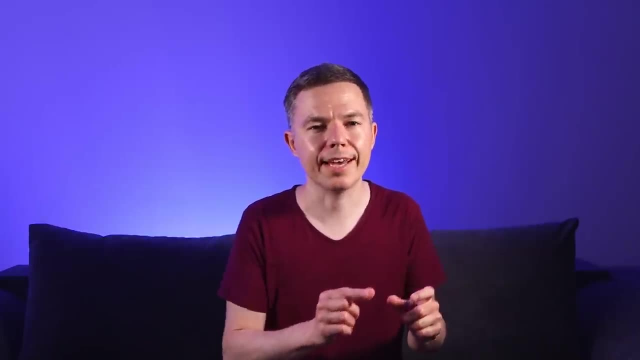 stakeholders, communication resources and procurement management. Now list all the processes, tools, templates and workflows inside your organization, Then illustrate how they interact with each other. This exercise will help you identify weak spots and inefficiencies in your project management approach. 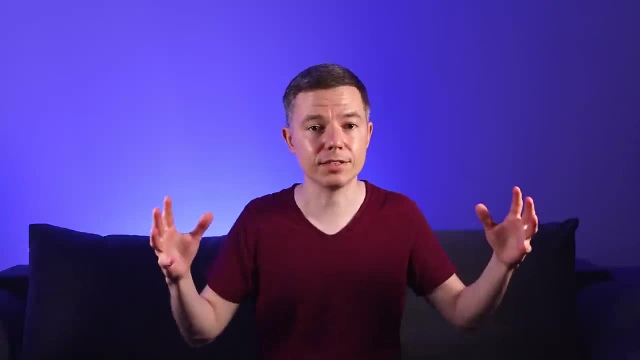 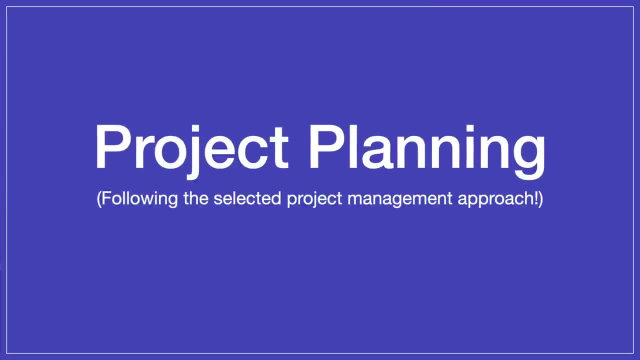 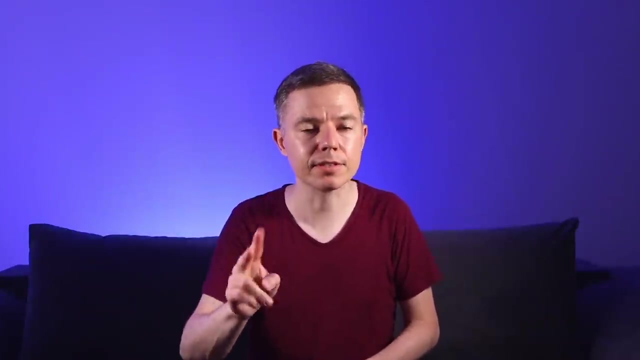 and knowledge. In addition, it will help you systemize your knowledge and understand the whole system. All right, at this point we start planning process Following the project management approach we selected, But there are two fundamental principles you need to follow. 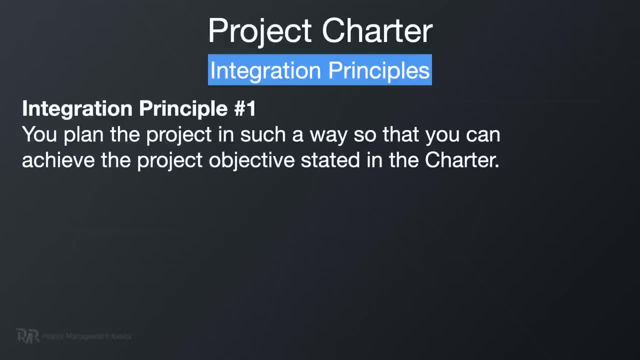 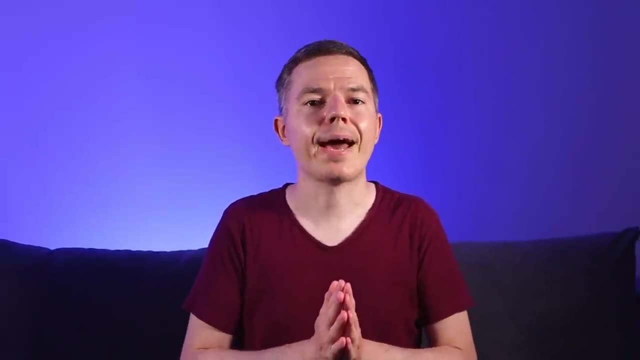 First, you plan the project specifically to reach the objective stated in the project charter. Second, you focus on specifying and digging deeper into the high level information you captured in the chapter. These two principles will safeguard you from spending resources on something clients didn't ask for. 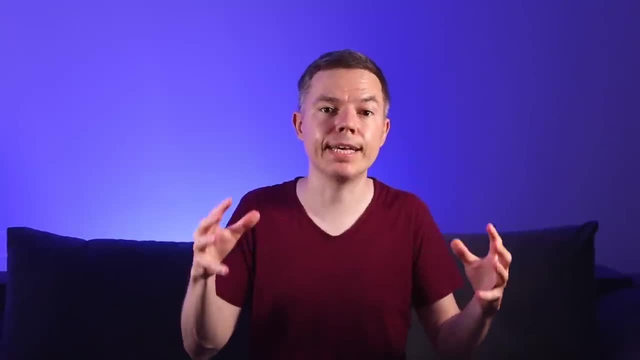 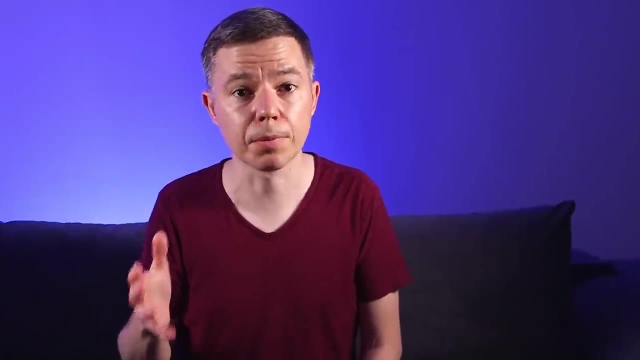 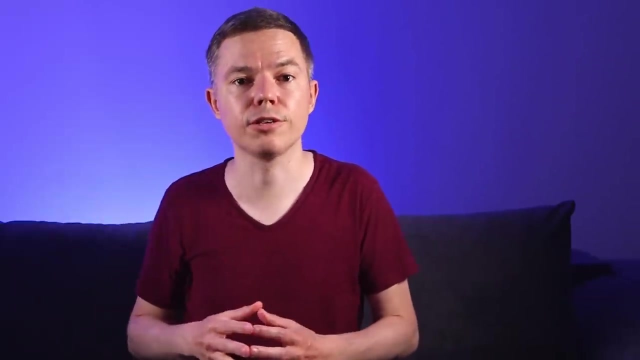 Moreover, it will keep your clients expanding demands within the constraints and boundaries of the project. On the other hand, if clients want to adjust project objectives, it's totally fine, But they need to update the charter, which will allow you to renegotiate project budget timeline. 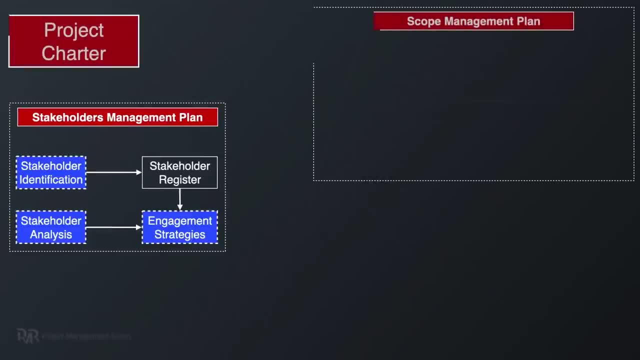 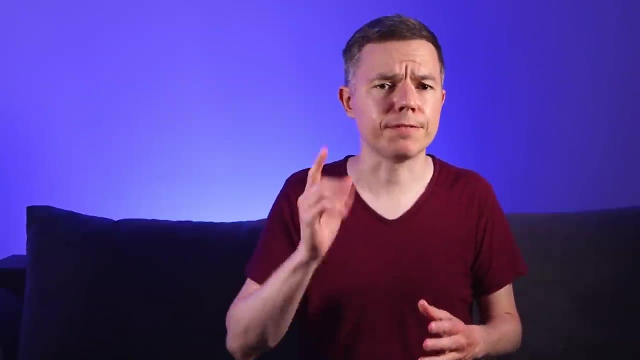 and scope. So as the starting point of planning, we need to take high level requirements and scope of the project from the project charter. We'll break these requirements into smaller pieces and start to work out the details of each requirement. Then, if needed, we write specifications. 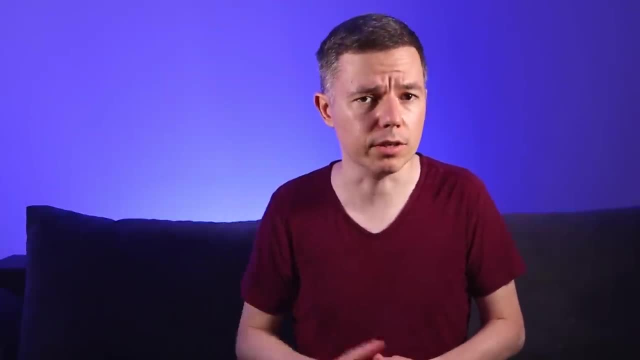 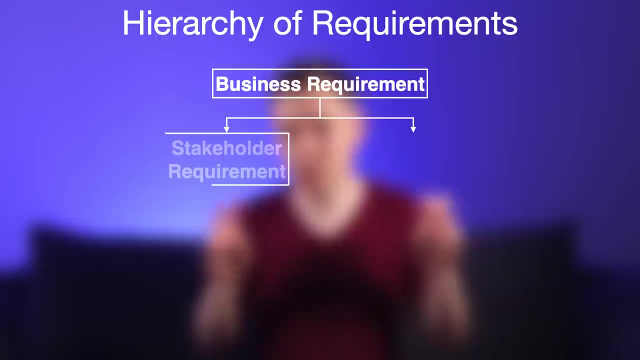 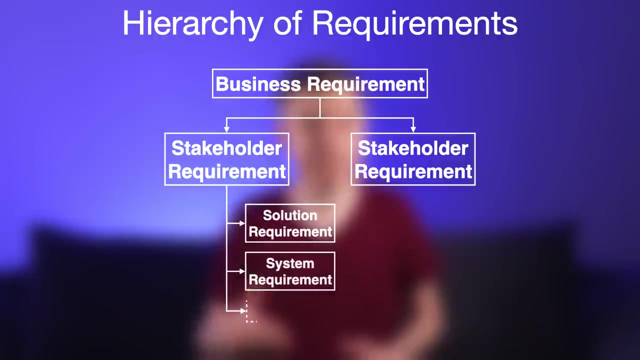 use the stories, draw mockups, wire frames and so on. So first you need to collect business requirements from the clients, Then you need to identify stakeholder requirements, and so on. You need to identify the requirements from clients and subject matter experts of all relevant fields. 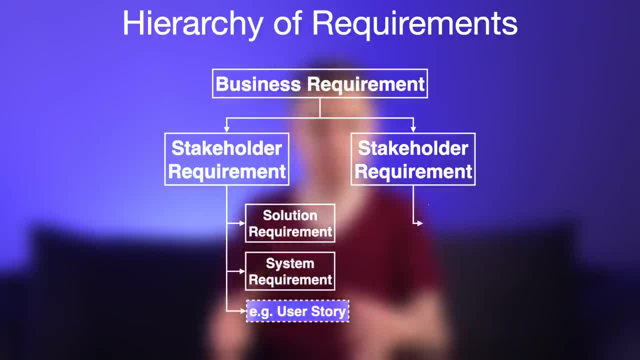 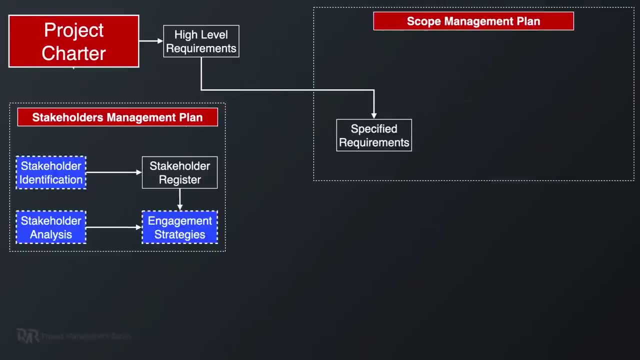 And after that you need to work with your project team and subject matter experts to produce solutions and specific product or system requirements. So that's why stakeholder identification starts here as well, and it continues throughout the whole planning process. Again, keep in mind that each new stakeholder 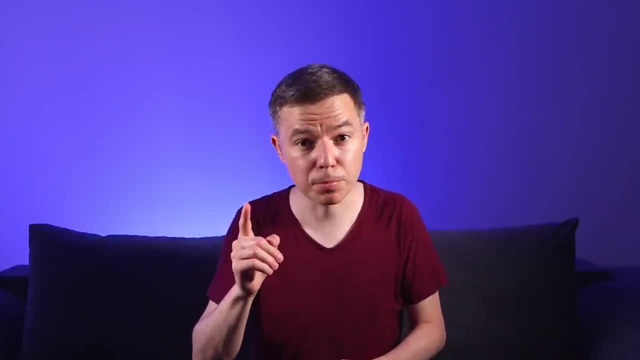 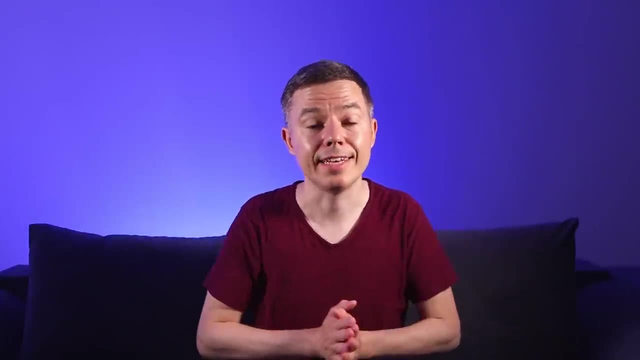 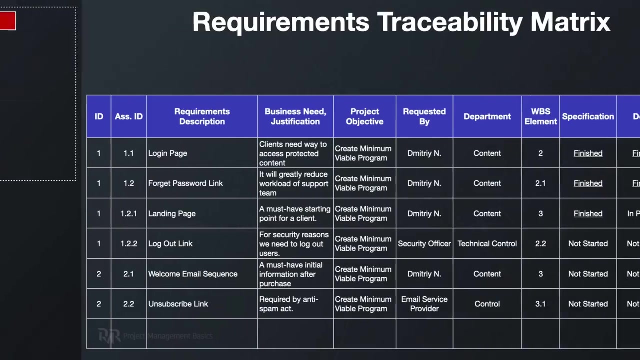 may provide you with new requirements, But what's even more important, your goal here is to ensure that all stakeholders pursue the project's objective in the first place. To help you manage stakeholder requirements, you can use requirements traceability metrics. It's just a spreadsheet that maps all project requirements. 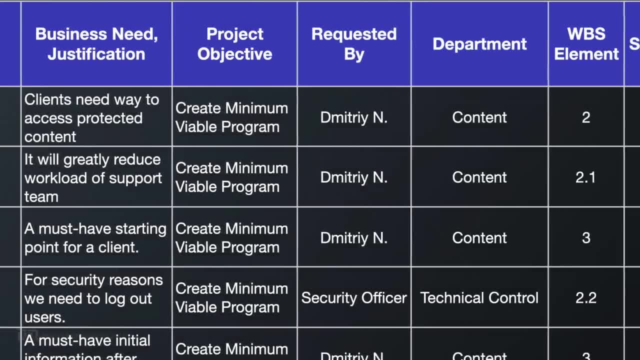 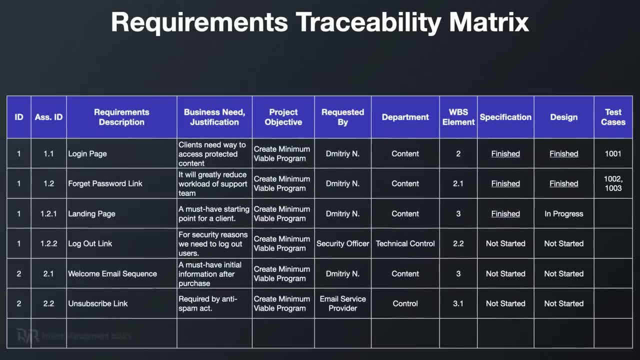 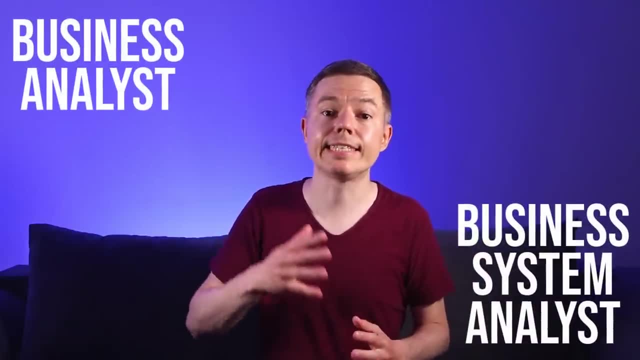 to stakeholders who requested them project objectives that these requirements help to achieve, work, breakdown, structure elements and support projects. By the way, I believe you should not collect requirements yourself. Business analyst is a dedicated role on a project specifically trained to collect requirements professionally. 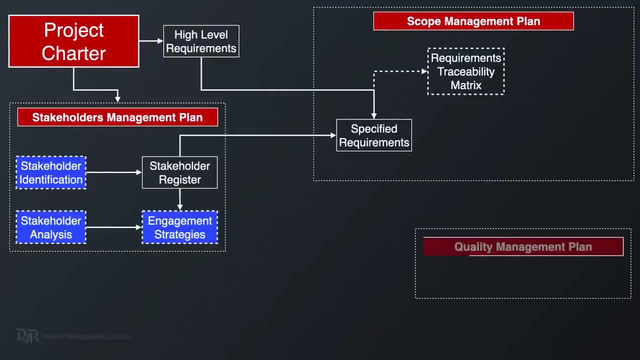 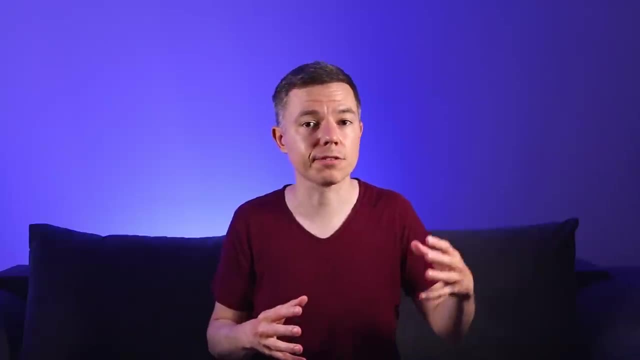 But in any case, when you define the requirements, you also need to think about quality management. In essence, the quality of the product is the part of the project scope You see. later you will need to identify specific tasks and make a resource of time and resources. 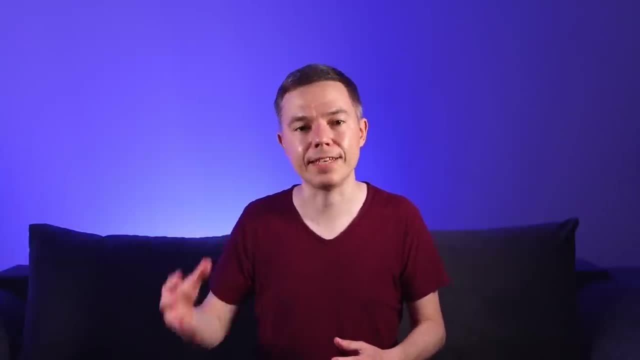 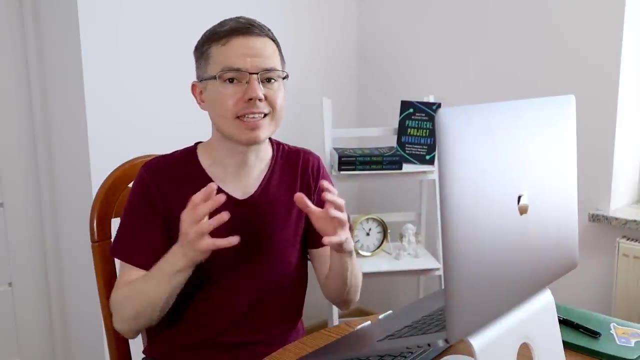 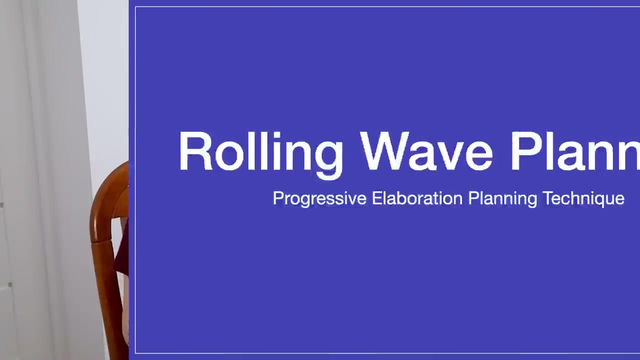 so that your team can ensure quality and fix defects. Okay, here's another intervention from the real world. In many industries, you can start implementing the product or service before you have collected all the requirements and finished planning. In this case, you can apply. 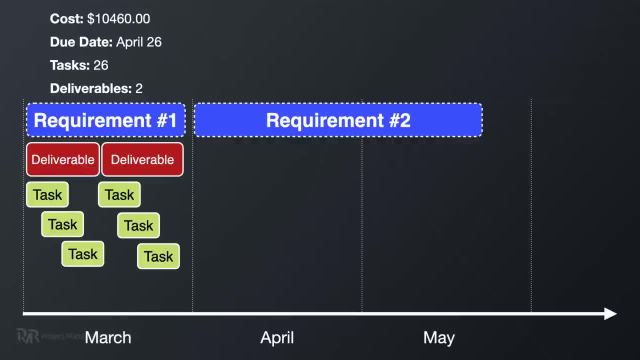 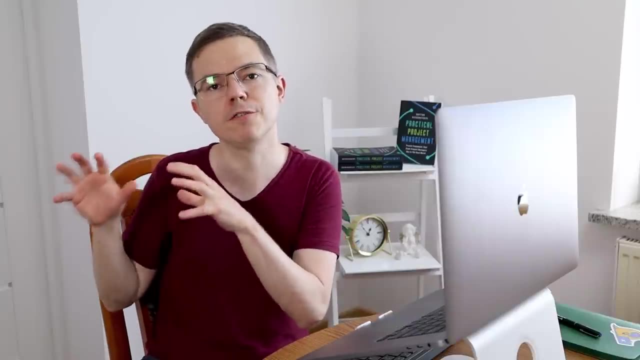 the rolling wave planning technique. This is a progressive operation technique in which you plan all the requirements and finish planning. You plan for the imminent requirements in all the details, but requirements that are logically further in the future can remain on a higher level. Nevertheless, you do plan for these future requirements. 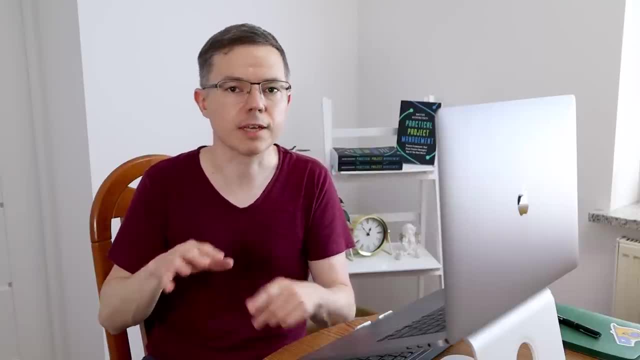 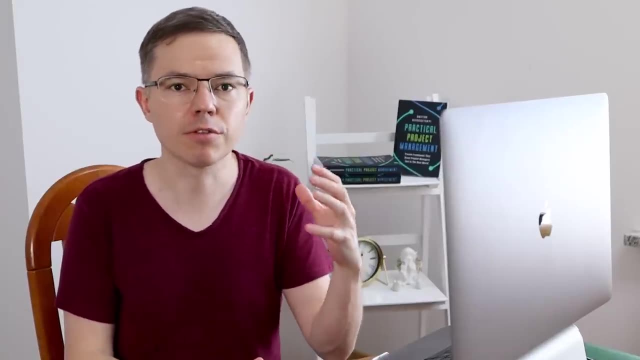 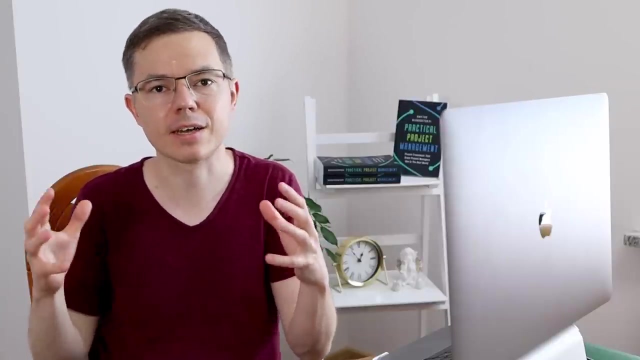 on a high level in all terms of project management, like project scope, budget schedule, risks and other aspects. And, yes, you do it right at the start of the project And your goal is to allocate enough time and resources so that you can implement these requirements. 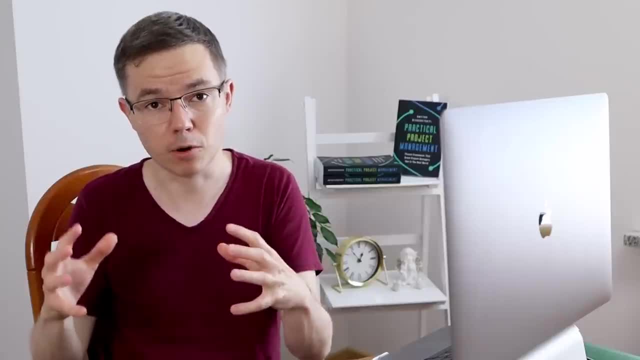 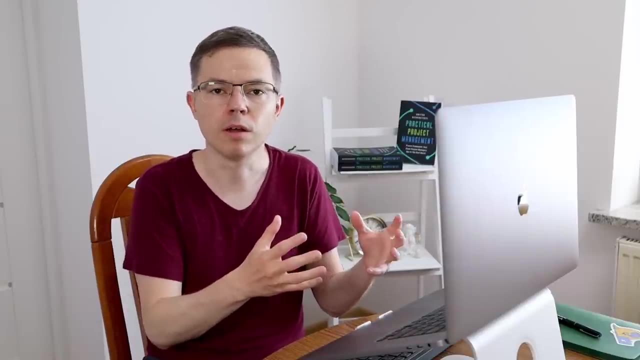 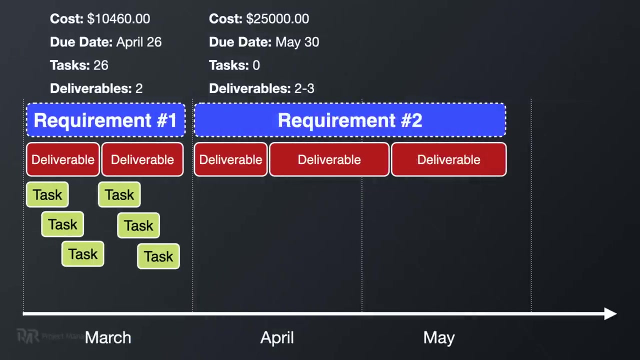 considering all the uncertainties you have at the moment. That's exactly why you don't spend months planning out the whole project in, for example, waterfall methodology or any other plan-driven methodologies. Instead, you plan for the next few weeks of work in all the details and you keep the rest on a high level. 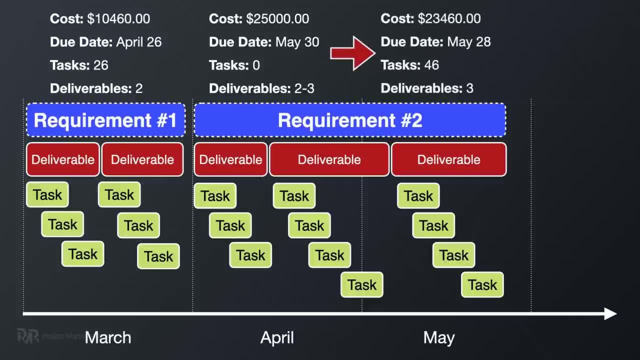 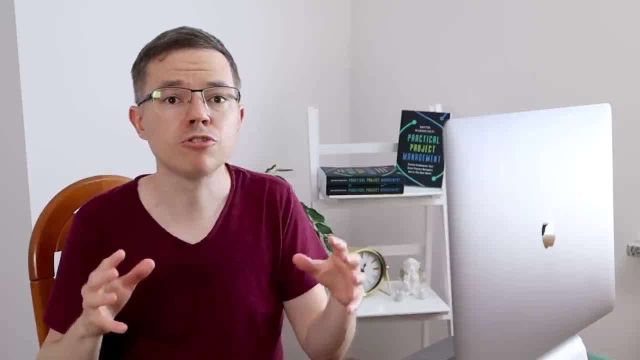 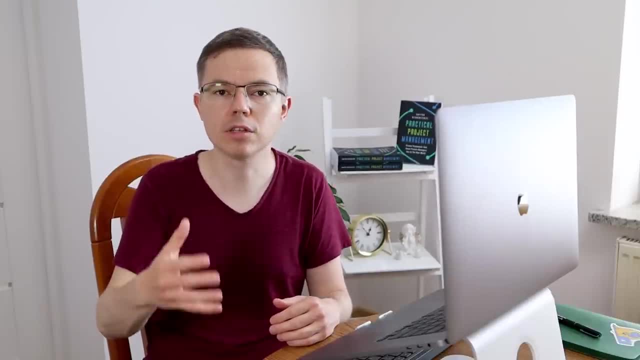 But then, during the execution, you elaborate on your project piece by piece. So keep this specific technique in mind, because your overall project management approach should allow for additional efforts required to elaborate your project management plan And if you apply the rolling wave planning technique. 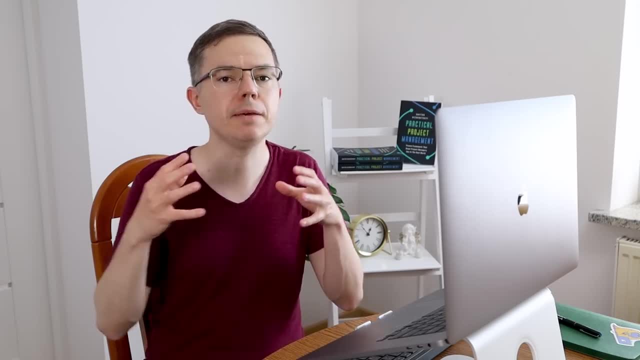 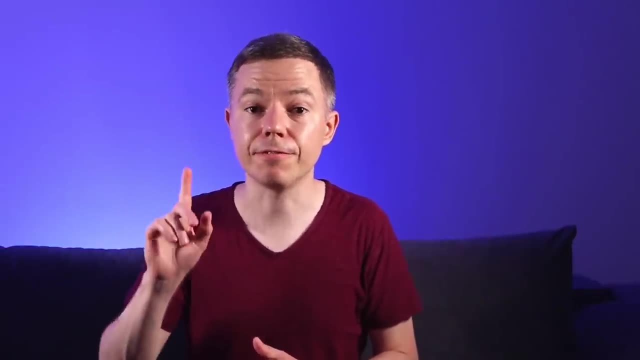 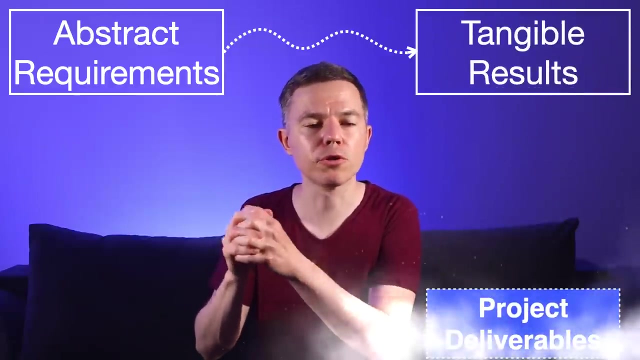 then all the processes and tools that you use will be impacted by this decision. Okay, no matter what planning technique you use, the next step is vital. You need to transition from the abstract requirements to tangible results that your project team will create. These tangible results or parts of the project- 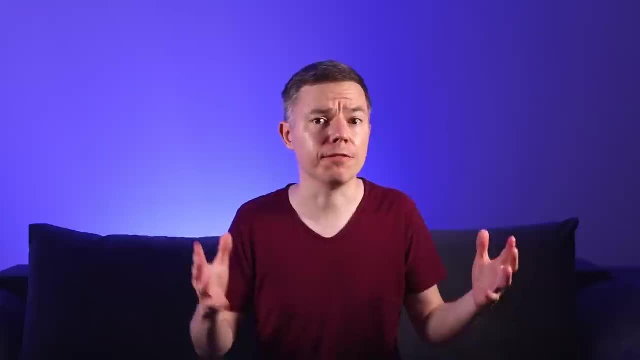 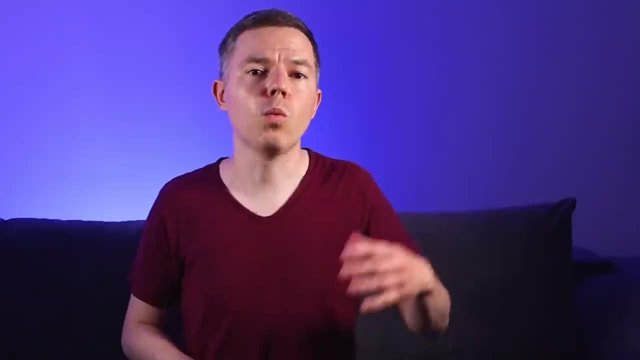 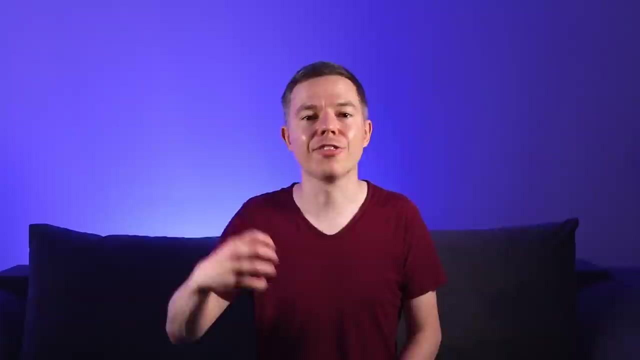 are called deliverables, And here's the main challenge. Unfortunately, there are no simple techniques or step-by-step instructions for this transition. From one side, your industry and the nature of the project will dictate the most common deliverables. On the other hand, you need to decide which deliverables. 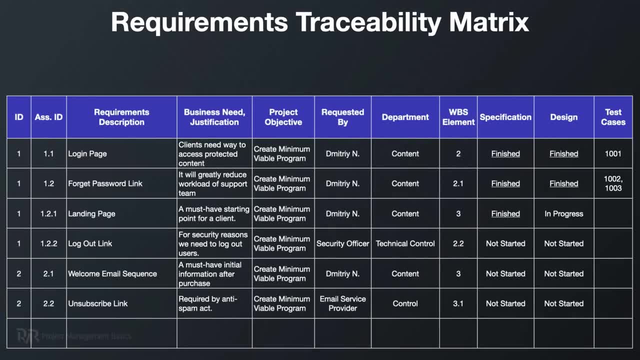 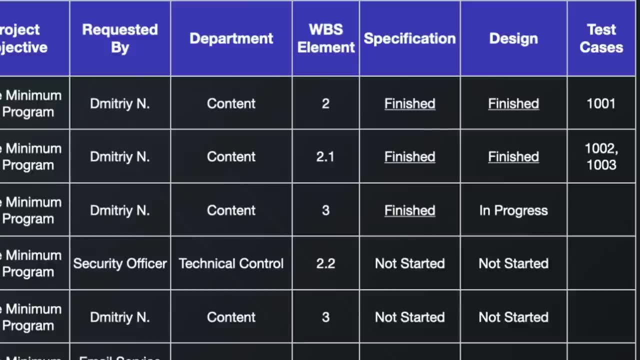 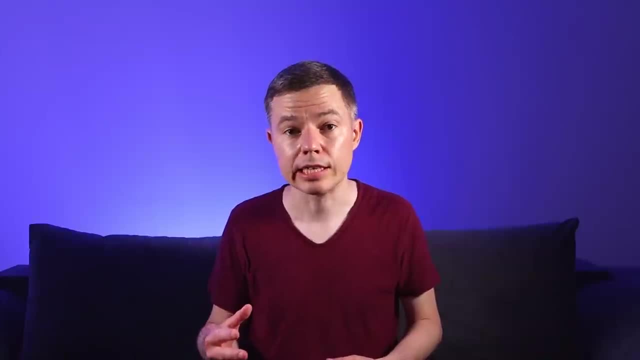 will include which sets of requirements And the requirements. traceability metrics, combined with the work breakdown structure, may help you map requirements to specific deliverables, So this way you can ensure you don't forget about these requirements in the process. It's a critical concept and we'll get back to it in a minute. 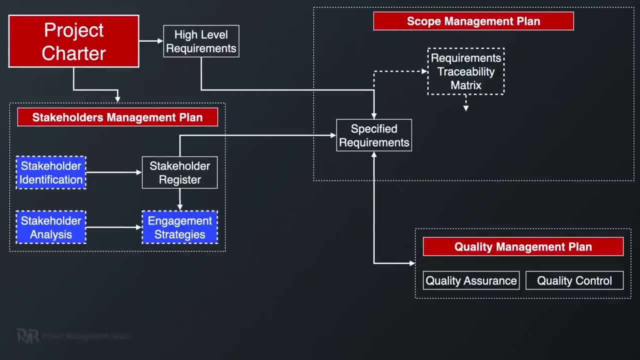 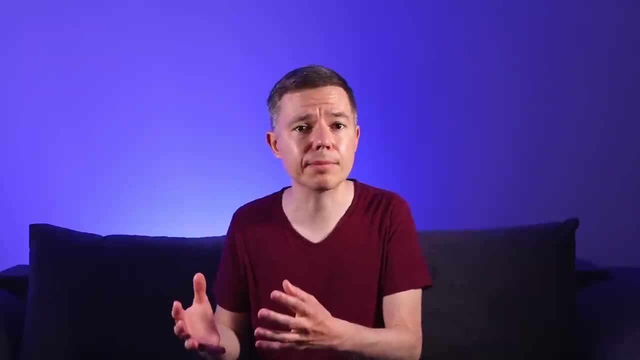 So stick with me here, Because first you need to create the project scope statement. It's another critical checkpoint in project management. It's another critical checkpoint in project management. You see, you collected requirements and identified deliverables, But don't assume that your clients 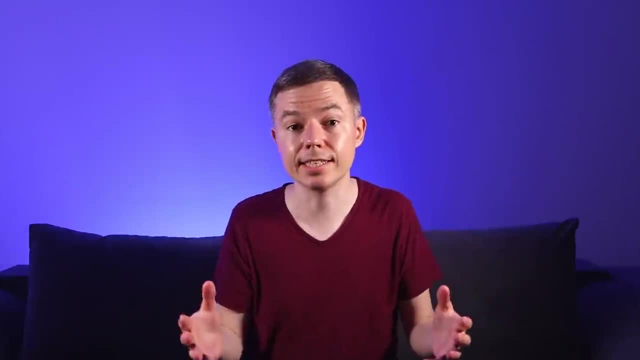 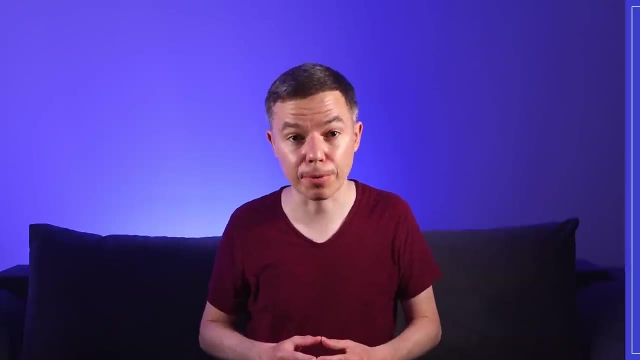 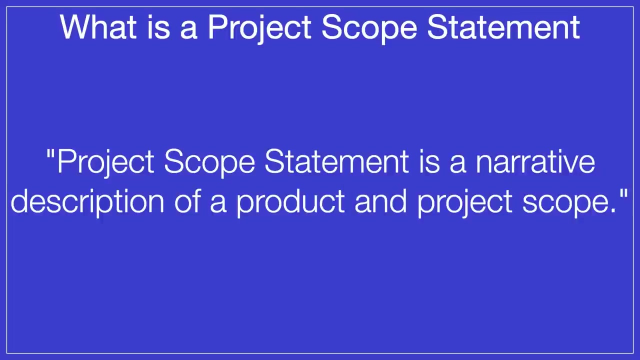 have the same industry knowledge and understanding as you do. You need to explain what they will get as the result of the project. So the project scope statement describes all project deliverables and how you will create them in simple language. Clients should understand what you will do, even in a technical industry. 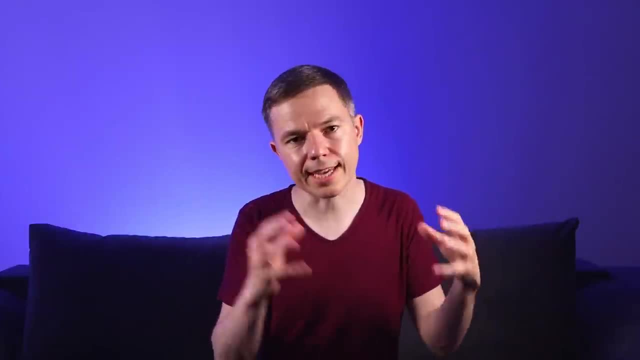 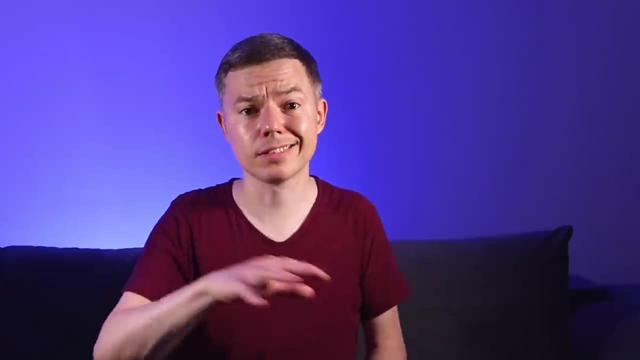 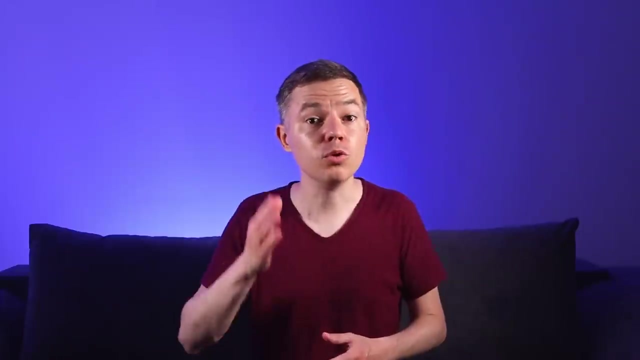 It's critical because next, you'll put a lot of time and effort into creating a plan to implement those exact deliverables And, as a result, you'll spend all the allocated resources of the project to create those deliverables. So you've got to be certain that that's exactly. 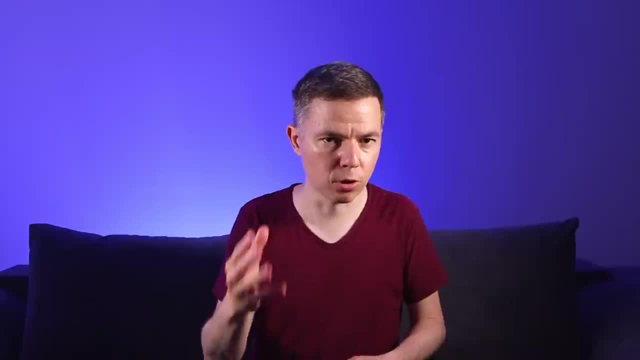 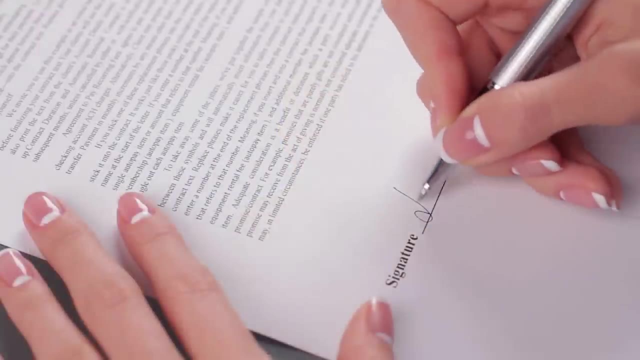 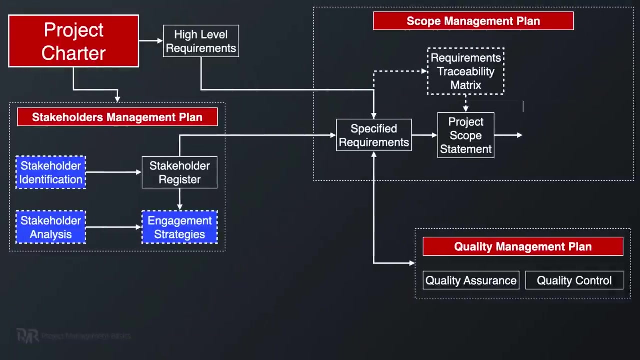 what your clients need. Moreover, they should be confident that these deliverables will help them reach the project's business objectives. Ideally, clients need to put a signature on this scope statement. Next, we have another critical integration point: We need to transfer deliverables that client signed off. 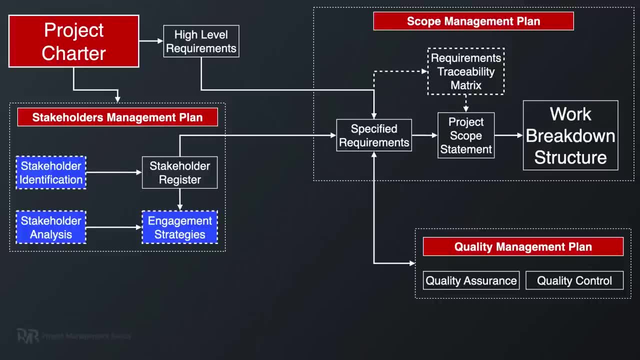 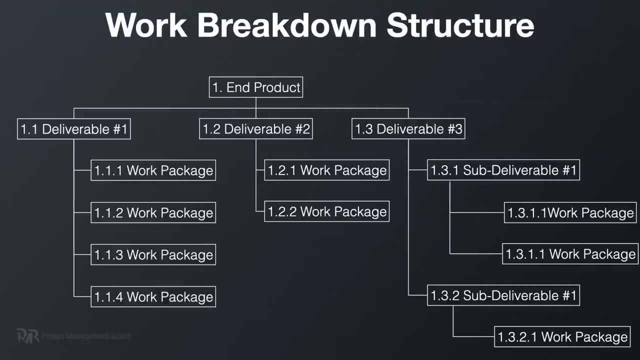 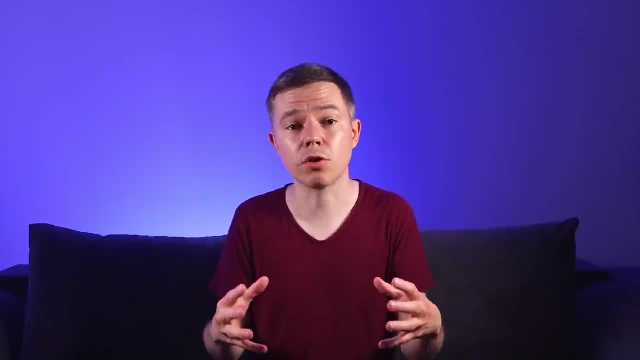 from scope statement into work breakdown structure. Okay, the work breakdown structure is the tool that helps you break down the whole project scope and identify 100% of it. And, by the way, project scope is simply the description of all the work that your project team needs to do. 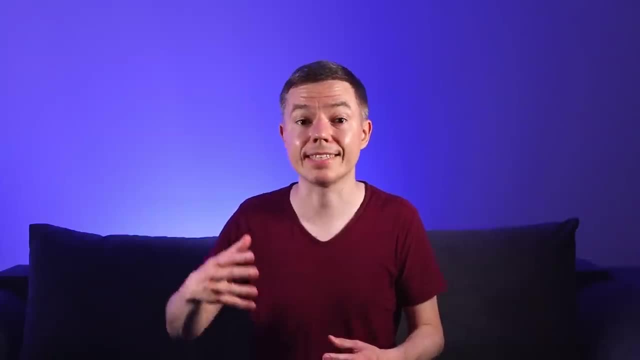 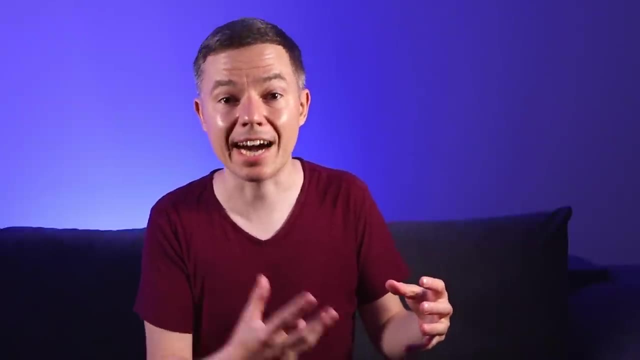 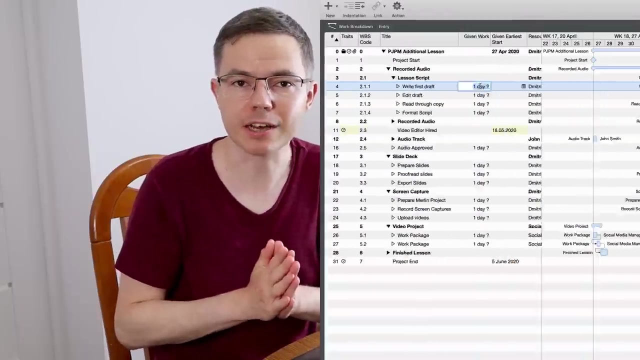 to create these deliverables. Usually, we describe them as tasks. From a practical standpoint, I recommend that you keep the naming of deliverables and their meaning. that comes from clients. You're still watching. good for you, because now we're going to talk about cool stuff. 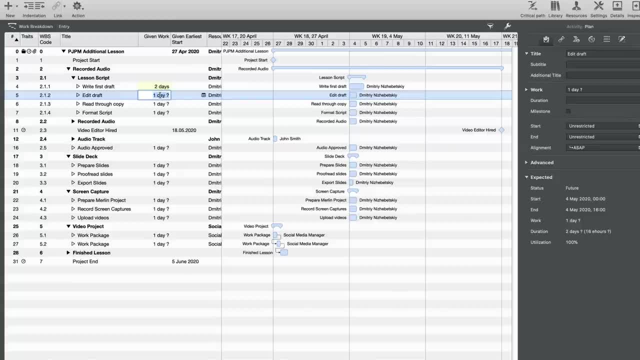 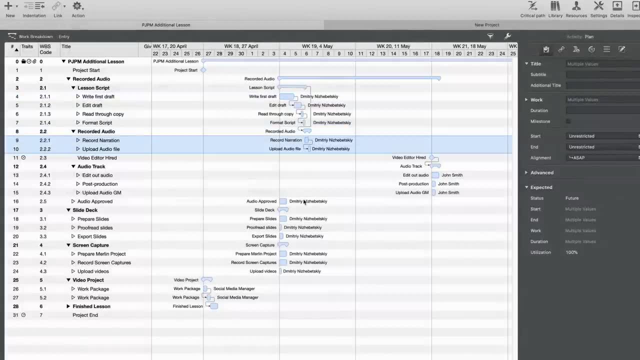 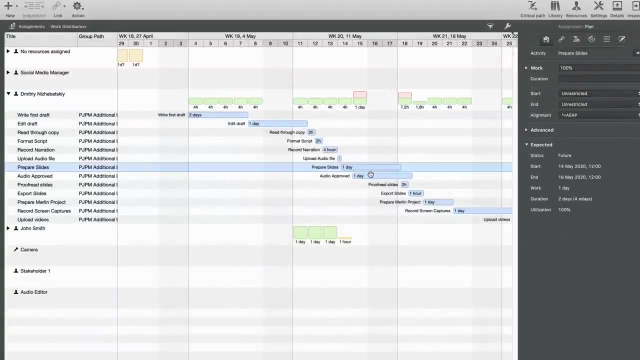 the project management software. As you already understand, there will be hundreds of tasks. These tasks will have lots of attributes, and then you will assign dependencies and line them up on a gun chart. So tracking all these attributes manually, for example in Excel, is a waste of your time and effort. 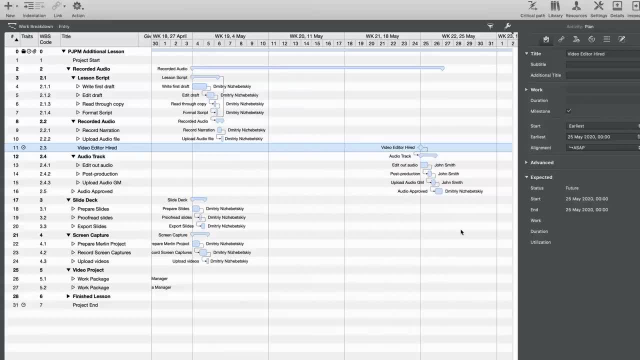 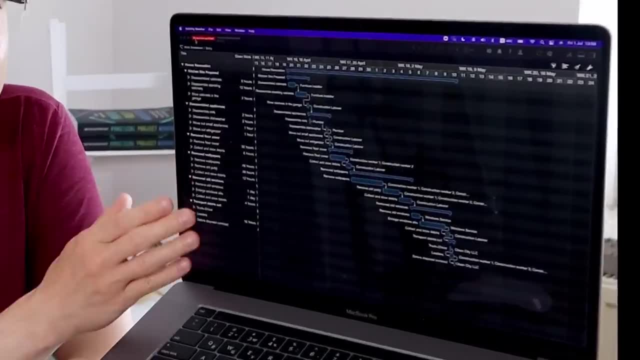 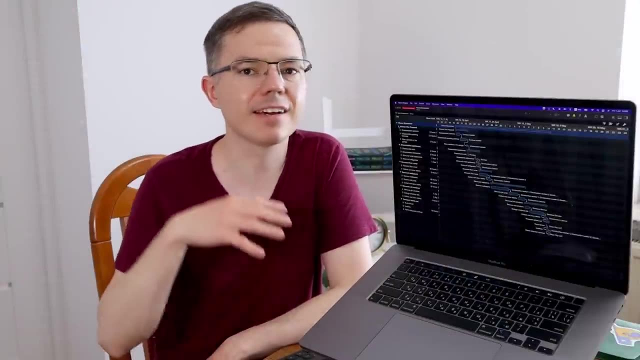 Making a change in the project management plan like that will be painful as hell. That's exactly why creating a work breakdown structure is the common starting point for all these project management software applications. So the decomposition of deliverables and the rest of the steps I will explain further. 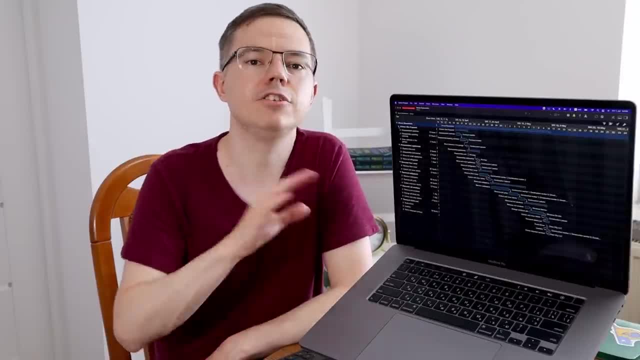 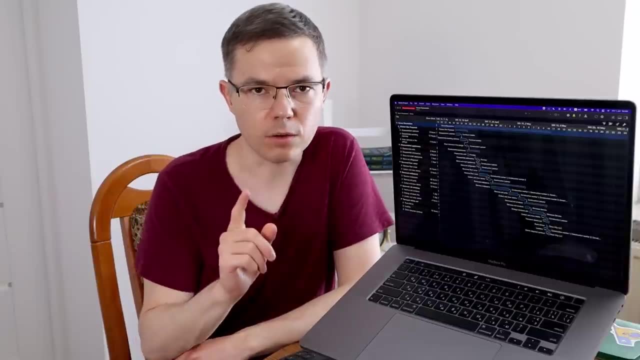 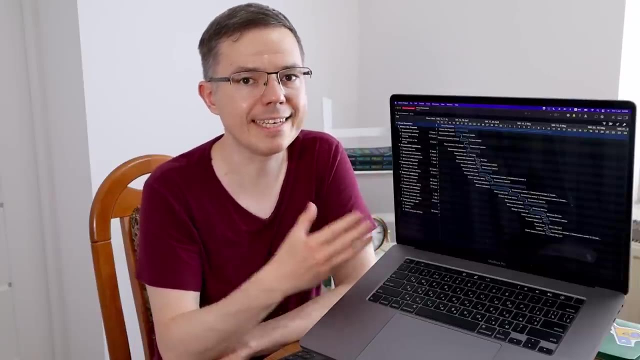 should happen in the dedicated PM software And, in general, you should try to keep all project information in one tool right from the start. A word of warning, though: any project management application is dumb. It's just a fancy calculator, So it does what you tell it to do. 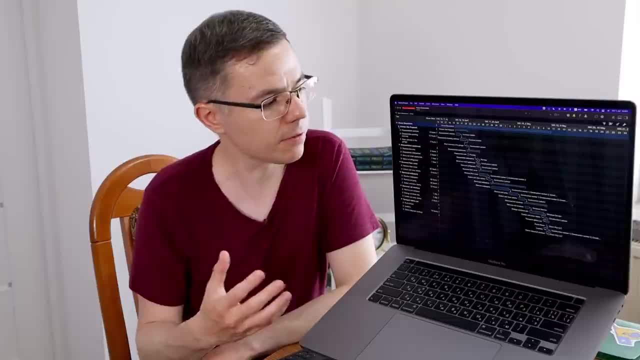 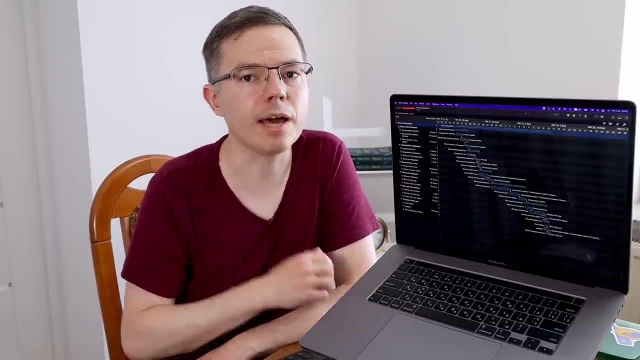 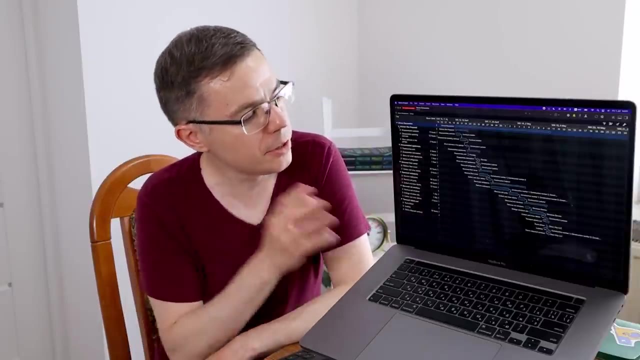 So if you use incorrect project management principles, for example, the principles of creating a high quality work breakdown structure, your software will give you a misleading picture. Therefore, you must understand the underlying project management principles used in these apps. That's why we're going back and we'll discuss. 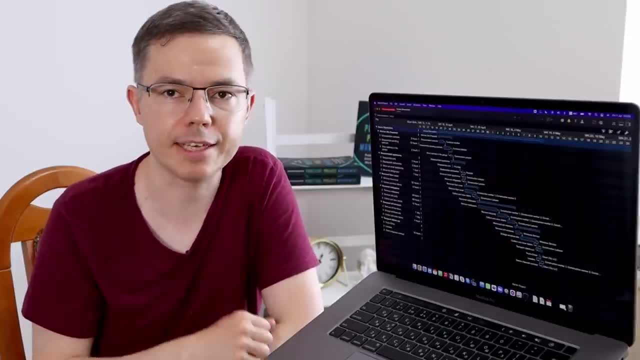 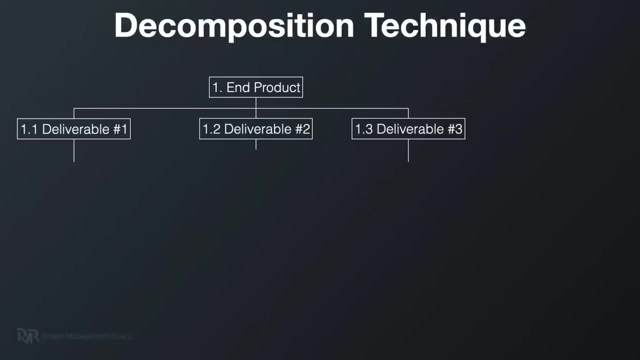 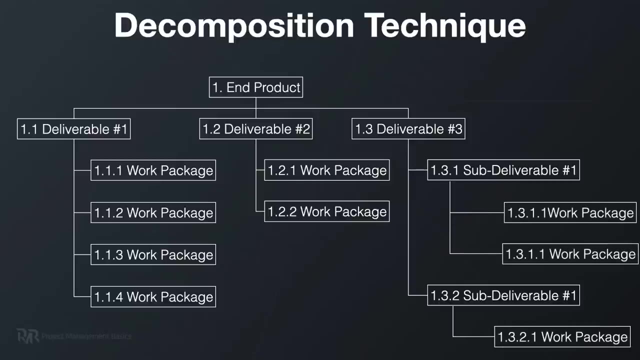 the decomposition technique in project management and few other key principles. WBS consists of big pieces of tangible results that we called deliverables and smaller pieces called work packages. These all have unique identifiers that clearly state their position in the structure. So we put deliverables from the scope statement. 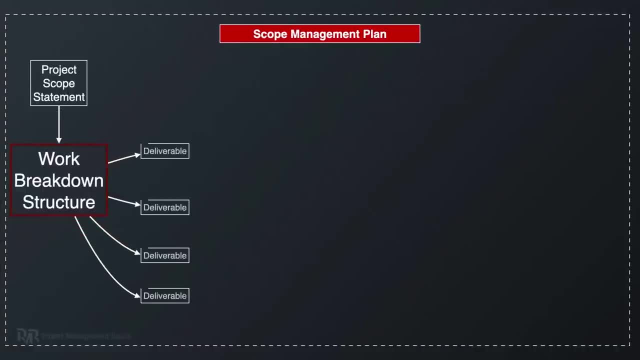 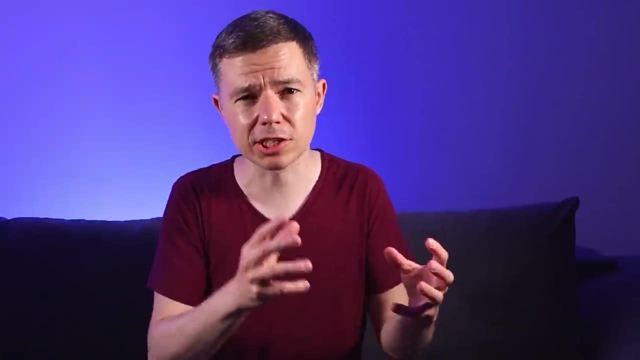 on the first level of decomposition. The idea is that we first list all the major pieces of the project. Then we need to decompose each deliverable into smaller components, the work packages- Again, work packages should also be finished- tangible and testable pieces of the project, but smaller. 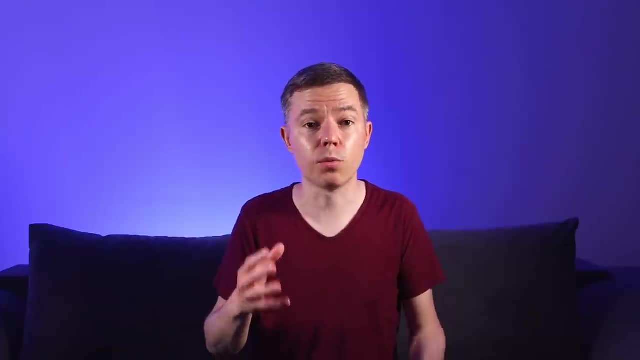 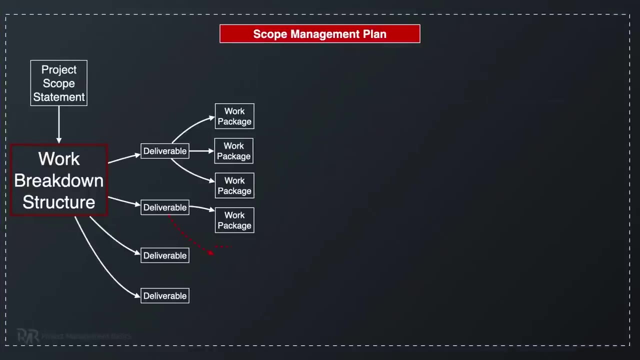 The rule of thumb from the practical standpoint is to make work packages small enough to fit within reporting period. And here's another important rule: If something is not in the work breakdown structure, it's not a part of the project. You see, it means that if you can't logically put 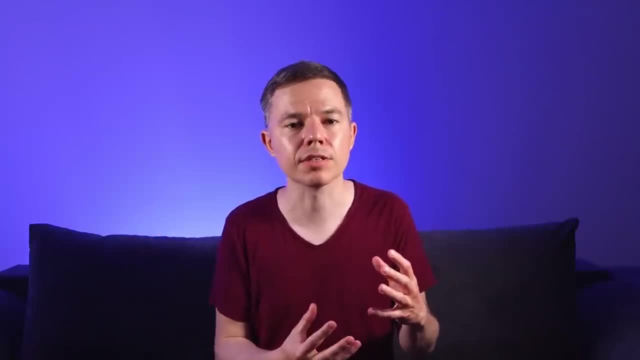 a piece of work under one of the major deliverables. you can't put a piece of work under one of the major deliverables. You see, it means that if you can't logically put a piece of work under one of the major deliverables, 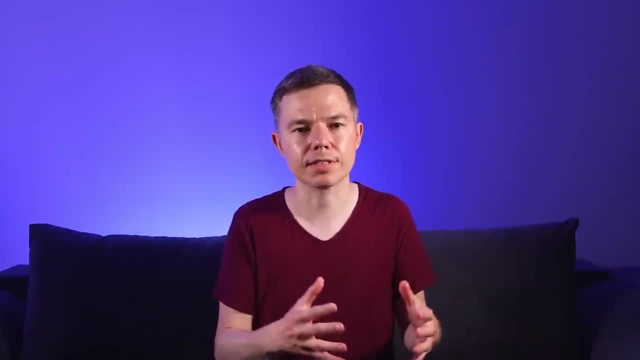 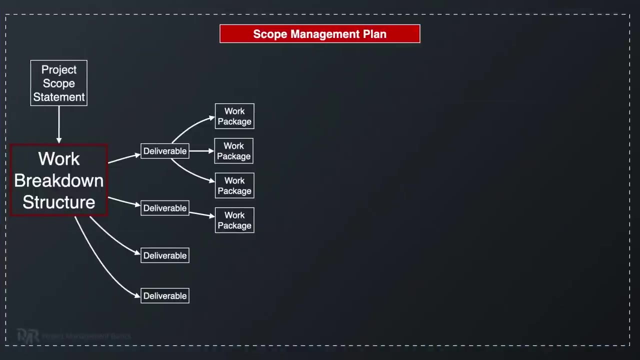 you most likely fail to identify 100% of the project scope in the beginning. It's a warning sign of scope creep. Next we go one step further. We decompose or break down all the work packages into tasks- Ideally, again, from a practical standpoint. 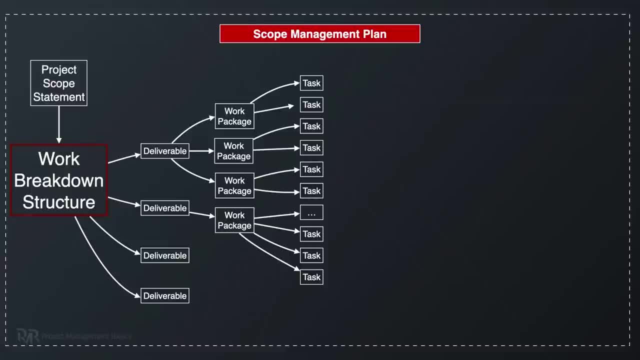 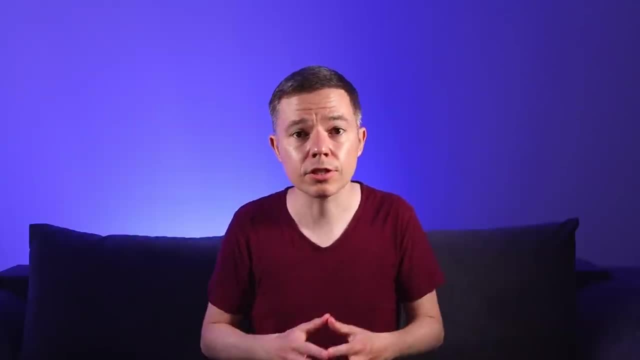 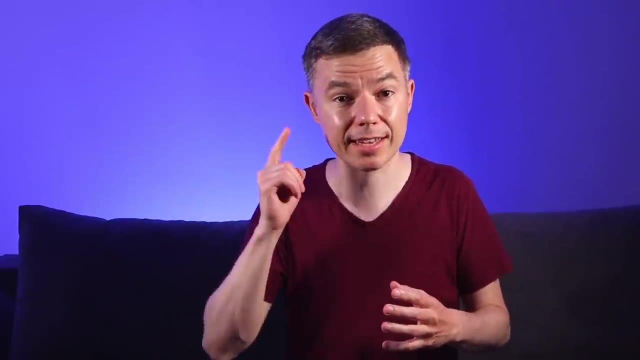 And from experience, I prefer tasks no longer than three work packages. And, from experience, I prefer tasks no longer than three work packages. Such level of decomposition provides better accuracy. By the way, some way at this point in planning, you may also need to start thinking about: 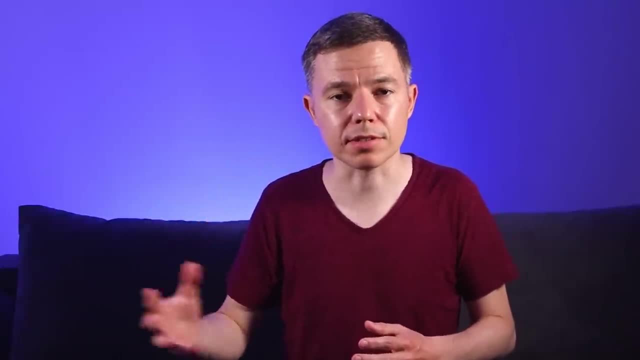 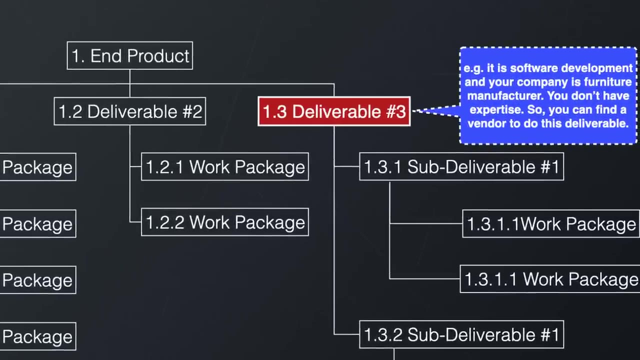 whether you need to outsource some project deliverables. It's called make or buy decisions. Many considerations go into these decisions. The major one is whether your organization has the required resources and expertise to implement all these deliverables. But let's move on. 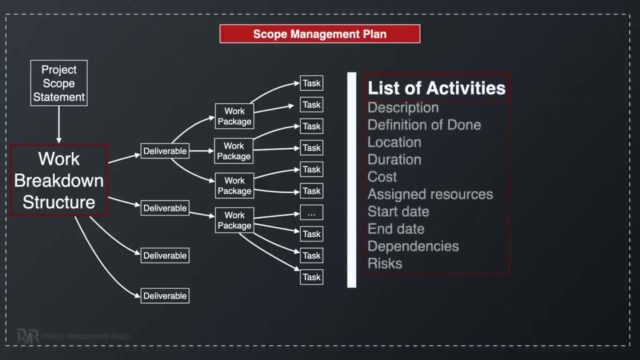 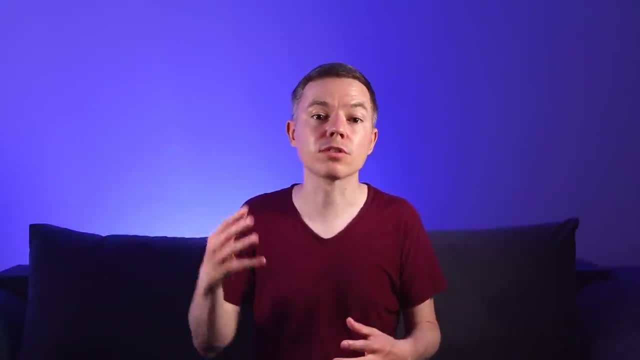 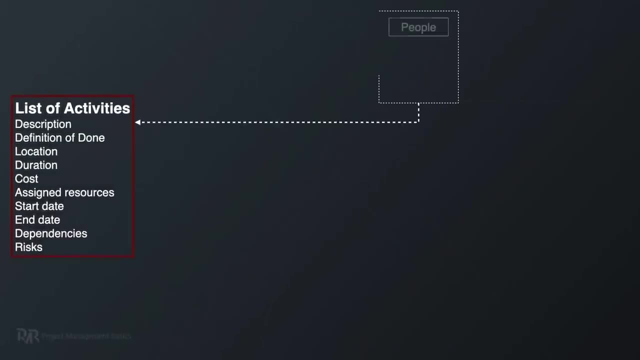 We have decomposed the work packages into tasks. Now our goal is to estimate each task. Usually, we start by assessing what kind of resources we need to finish this task. You need to think about people, their skill set and their level of expertise. 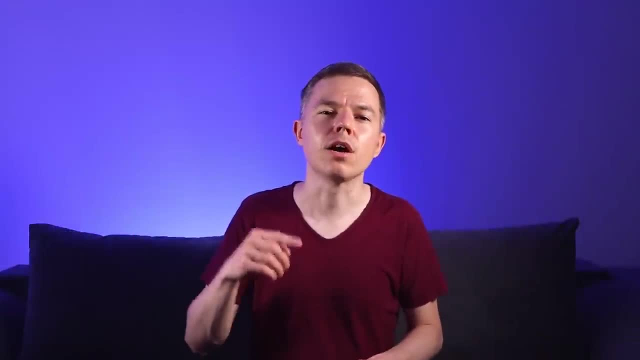 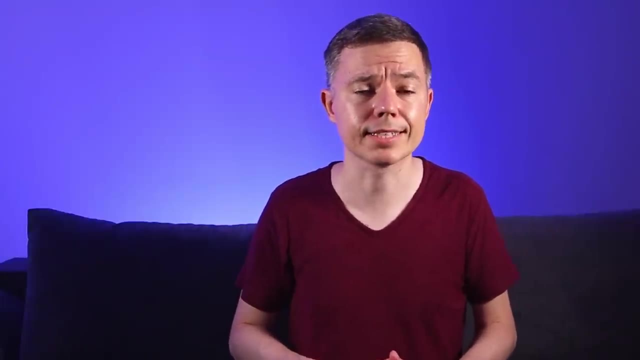 If you don't have a team yet, you'll have to create these role descriptions for the recruitment department. Or if you have a team already, you can assign people to the task. You can assign people to the tasks at once. On the other hand, we need to analyze what equipment 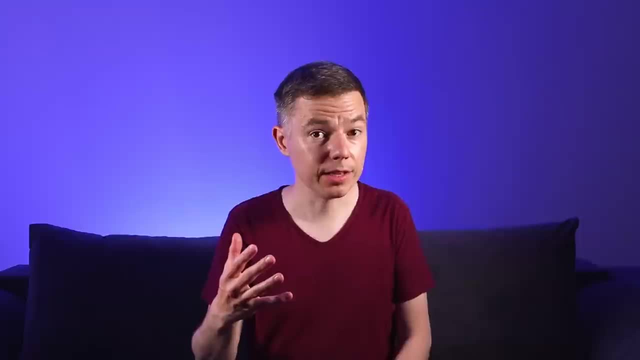 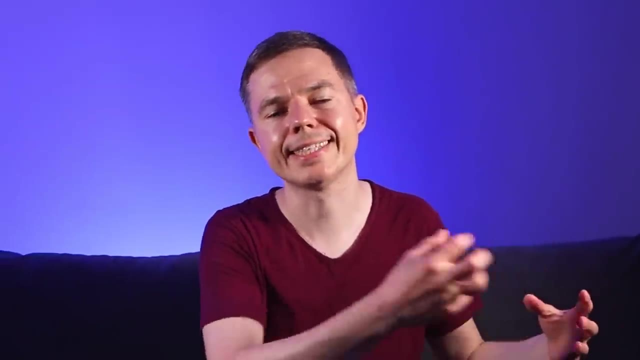 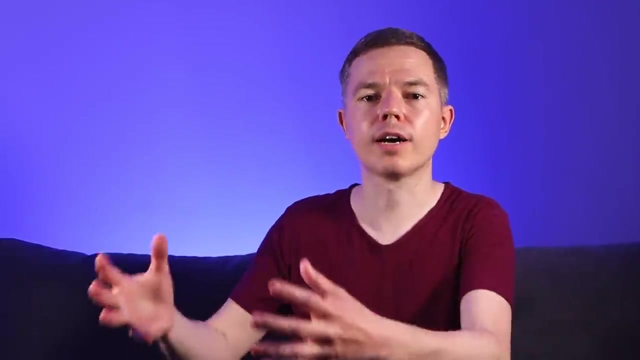 materials and tools we need for these tasks. So then we need to plan to acquire all these resources. Sometimes a company has a pool of people we can take for our project, so we'll need to negotiate internally, But likewise we may need to hire these people. 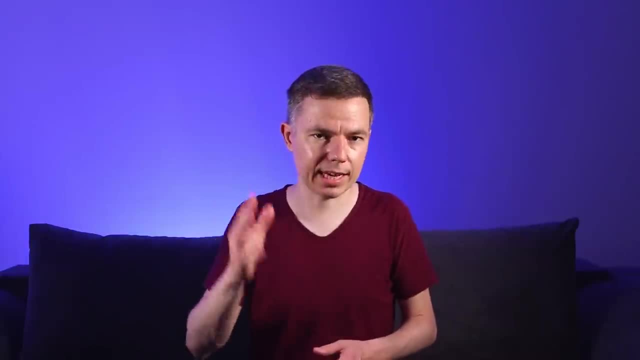 From an equipment and materials perspective, we have the same situation. The company may have a team, it may have the stock that we can use, it may have a list of vendors that we can contract, or we may need to find all these vendors from scratch. 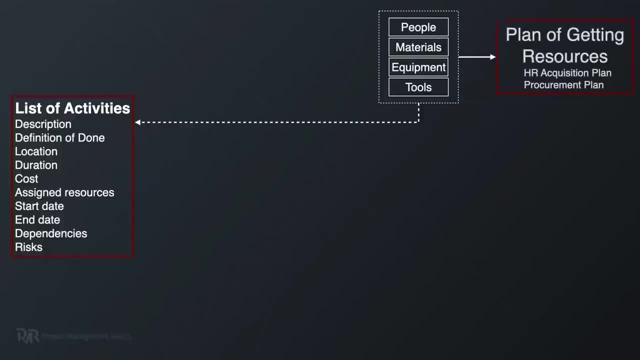 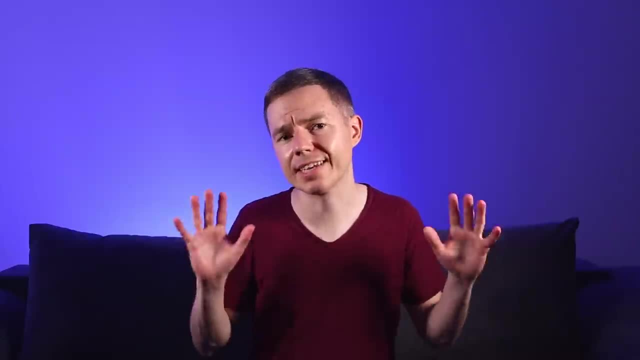 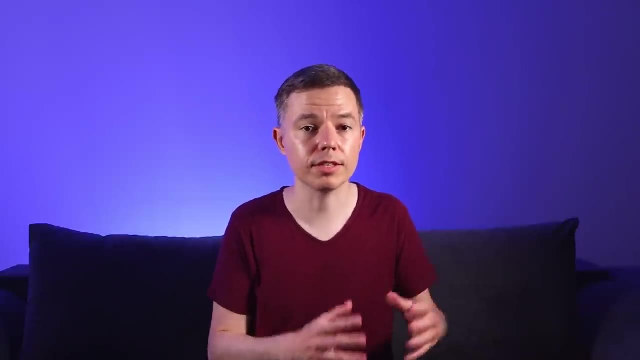 This analysis of required resources will result in two separate documents. The first one is the human resources acquisition plan. Nothing scary here, it's just the list of vacant roles on your project and the dates when you need them to join the team. The second document: 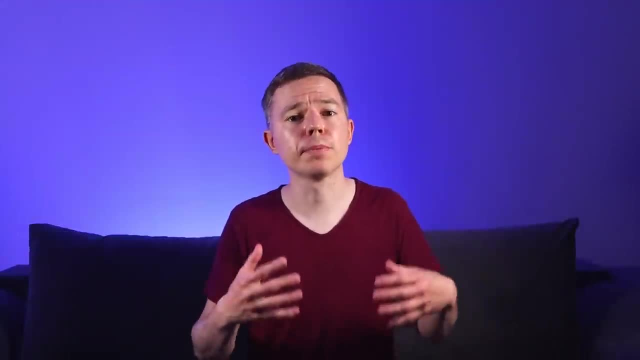 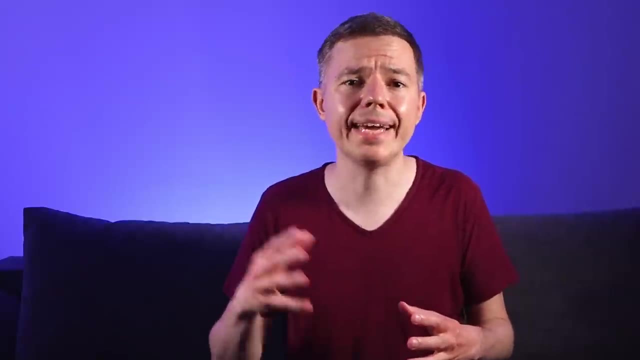 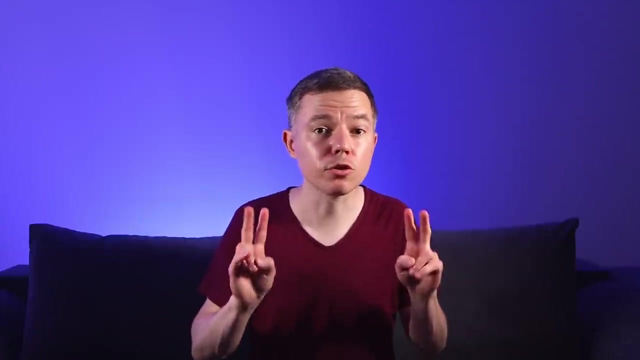 is the procurement management plan. Again, you need to plan how you will acquire equipment, tools and materials and when you expect it. So here you may need to engage with the procurement department or procurement manager of your organization. In any case, these two plans will impact your schedule. 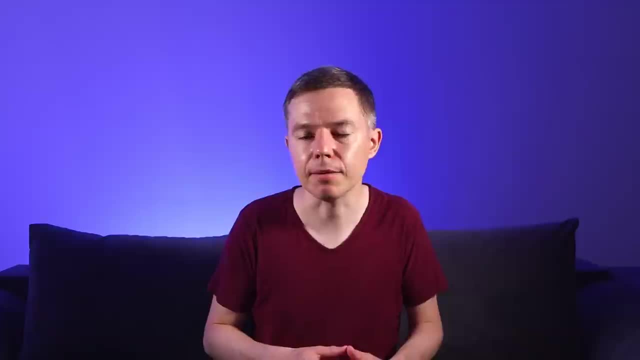 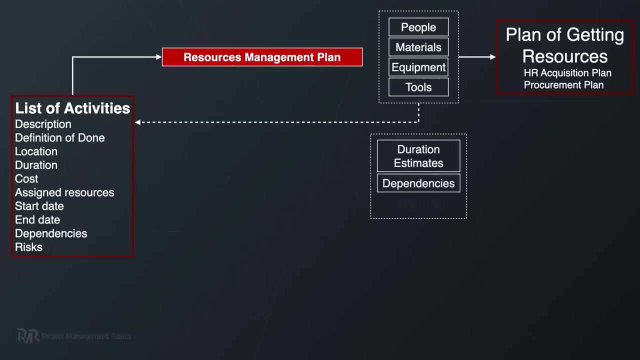 because we can't hire people the next day when we need them. It may take months. The same goes for equipment and materials. Your project schedule will have due dates for all those resources. Now we need to estimate the duration it takes for the assigned roles or real people to finish each task. 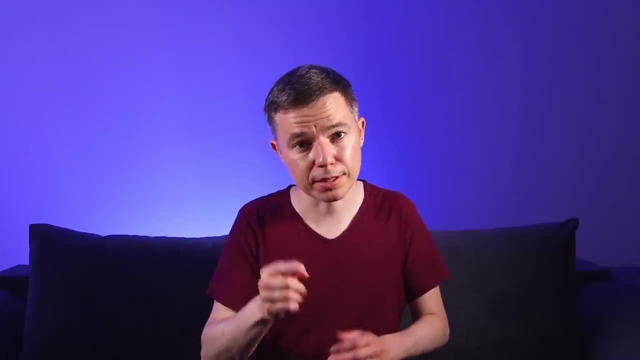 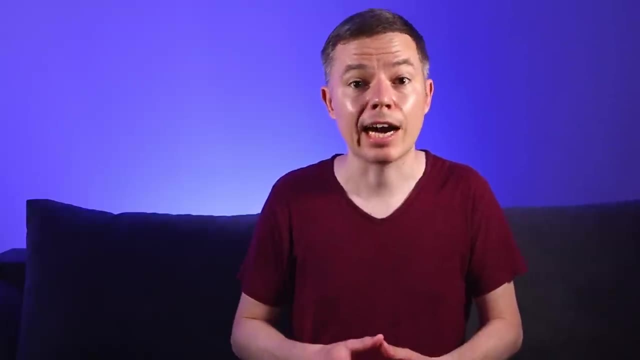 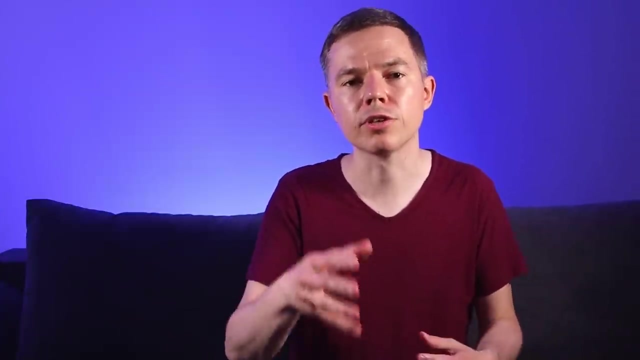 And a critical side note here- you, as a project manager, should not estimate tasks yourself. If you have the team already, obviously they do it. However, if you don't have any team members, you should ask for a pre-assigned expert to help you out here. 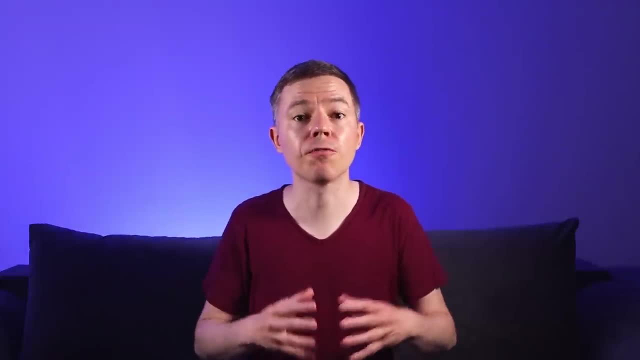 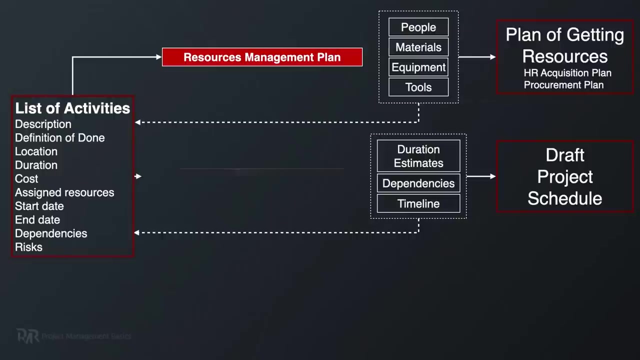 So always consider the average productivity of a role based on the experience level you identified, not the knowledge level of an expert who does the estimates. With all this information, we can assign dependencies between tasks and create a draft of the project schedule. You have to play around to create a final. 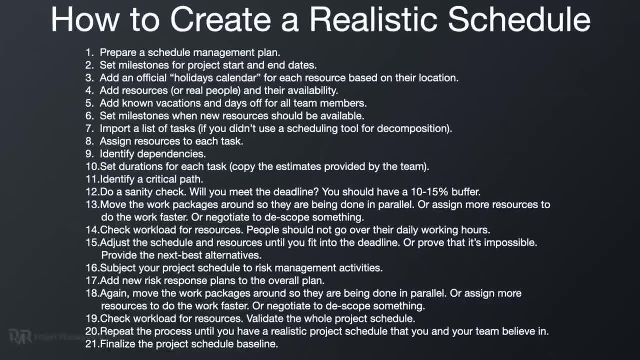 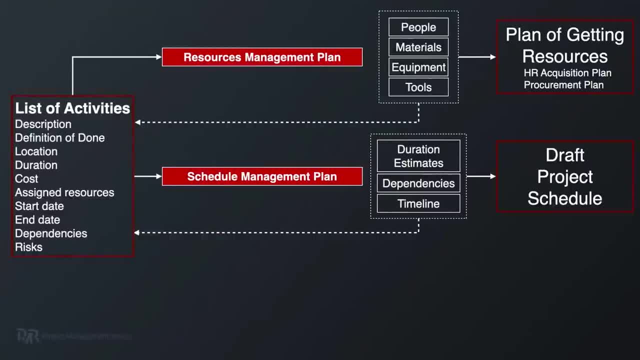 and realistic version of this schedule. So here is a step-by-step instruction on how to do it. You can pause now and read through this. Next, we can also find the average prices for the materials and hourly rates for the type and level of labor we need. 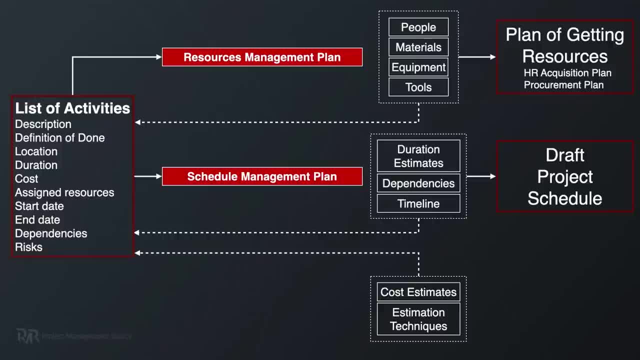 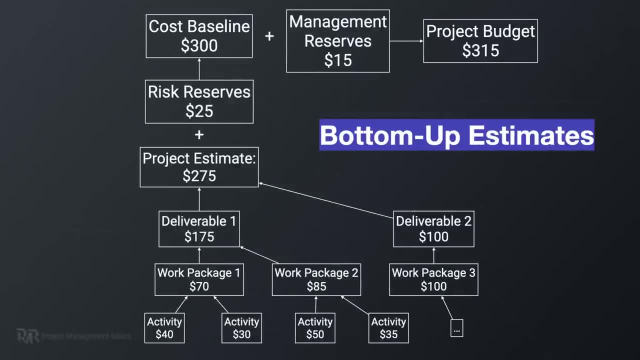 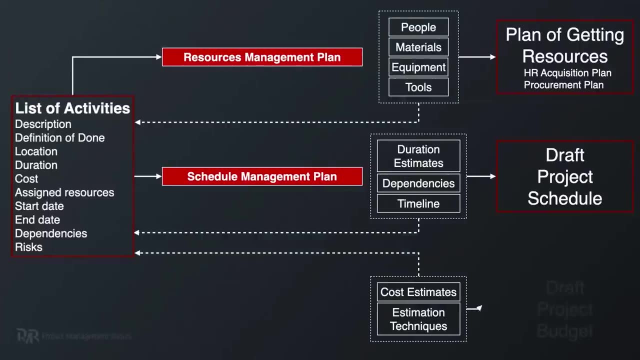 So we can easily calculate the total cost of a task. The idea is to perform the bottom-up estimate. First you estimate all tasks, then summarize them to the work package level. Then you summarize work packages to the deliverables level. As a result, you can create a draft. 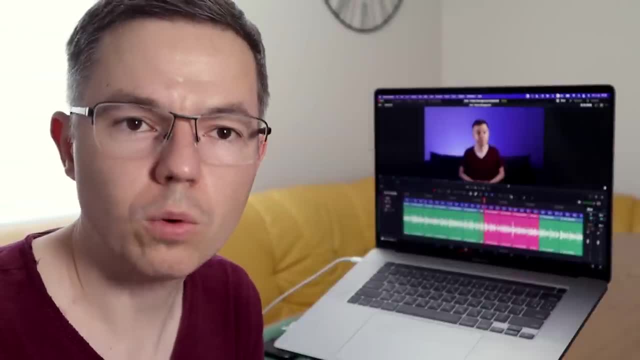 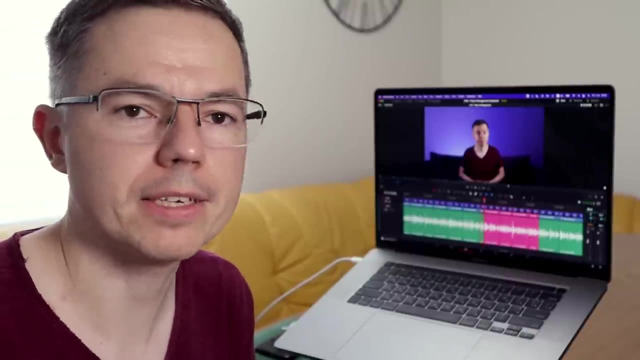 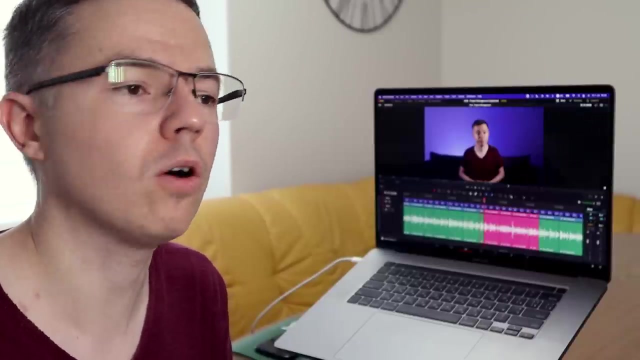 or the project budget. Another critical note here: what I've just described is a generic way of estimating tasks. If you work in the software development industry, for example, you have a prepaid team for the next few months. or if you work in a company that uses only in-house. 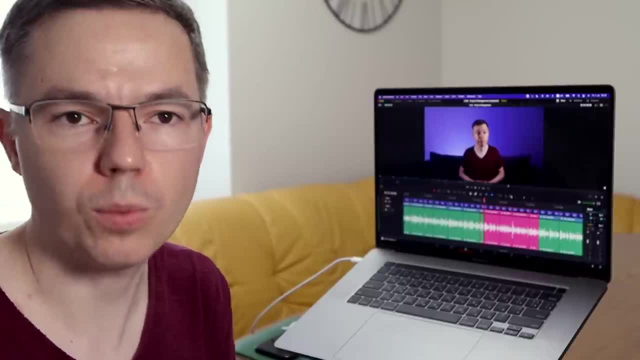 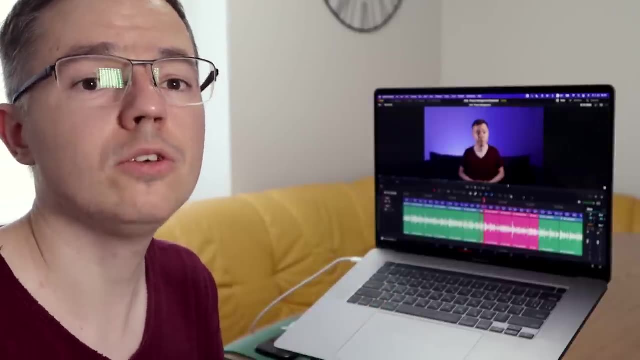 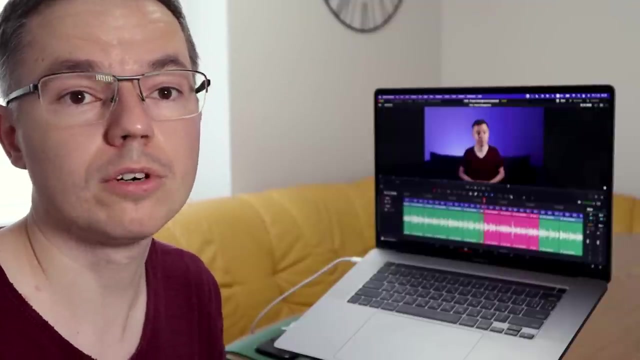 resources. there is no need to do it this way. So rather than assigning resources, estimating the duration and calculating the cost of the task, you directly estimate it in efforts, in-person hours for an average role that you will have on your team. 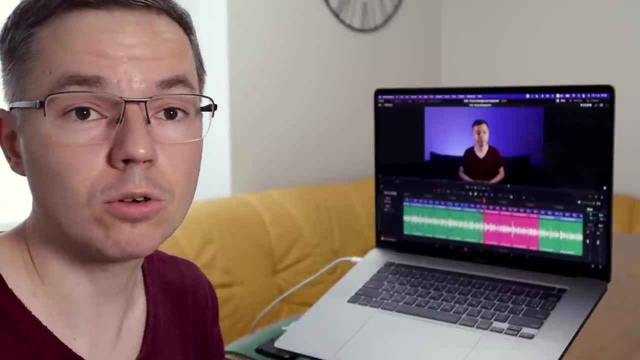 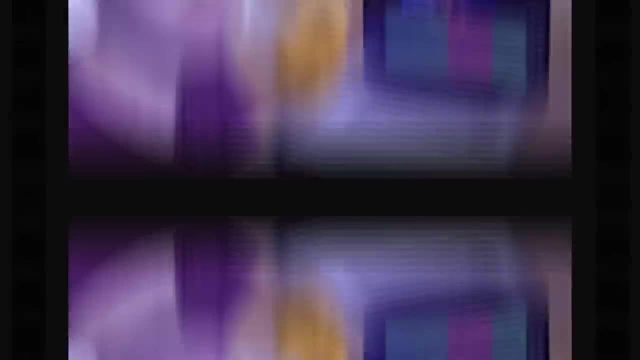 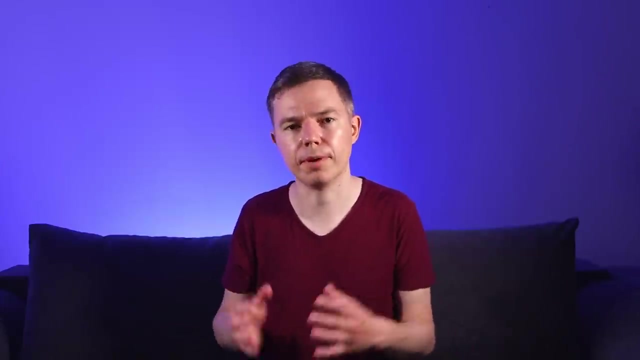 So in this case, you are more interested in leveling your resources and ensuring that you are using all the available efforts. Okay, let's get back to planning process. Okay, I keep telling you that you have created the draft version of the schedule and budget. 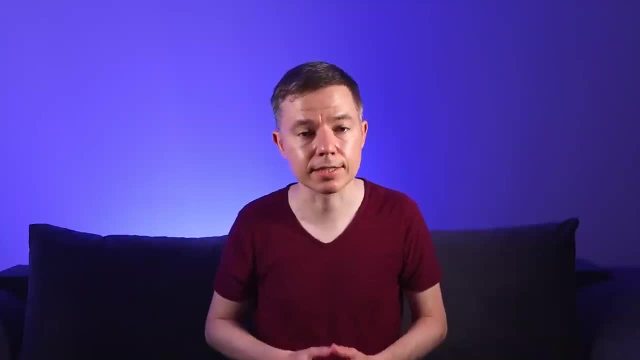 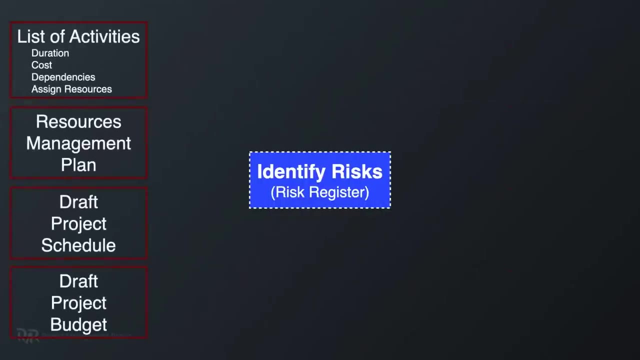 That's because we need to perform risk management activity, because we need to perform risk management activity, because we need to perform risk management activity before we can finalize the project plan. Okay, we've been identifying and analyzing risks since the start of the project. 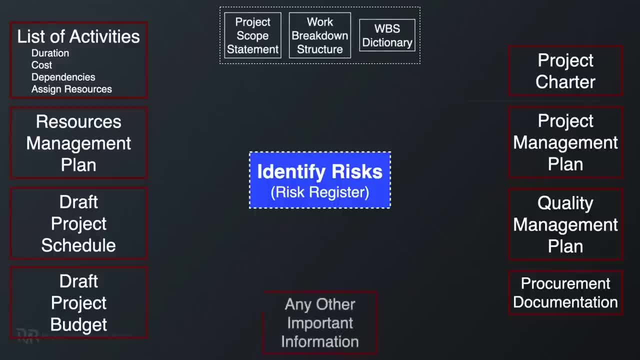 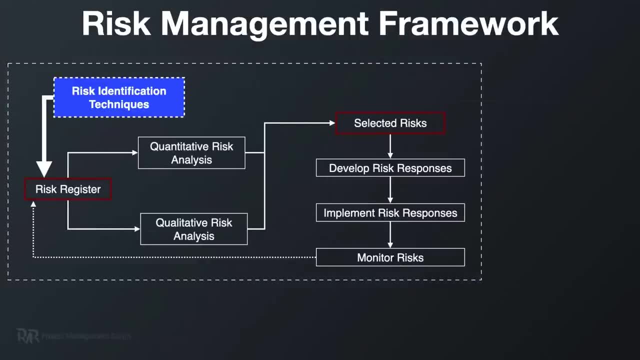 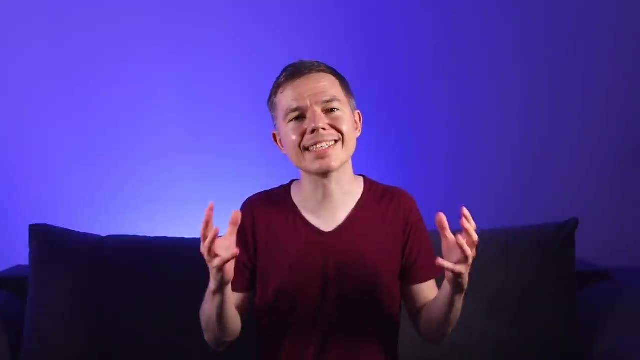 Now we need to run dedicated risk identification sessions based on the draft of our project management plan. Then we need to finalize the analysis, select the risk we need to address and develop risk response plans. But what does it mean to create a risk response plan? 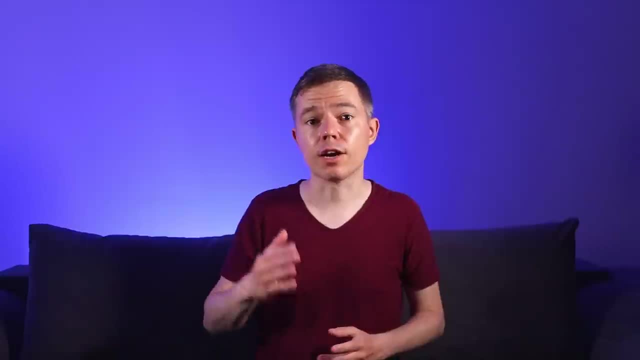 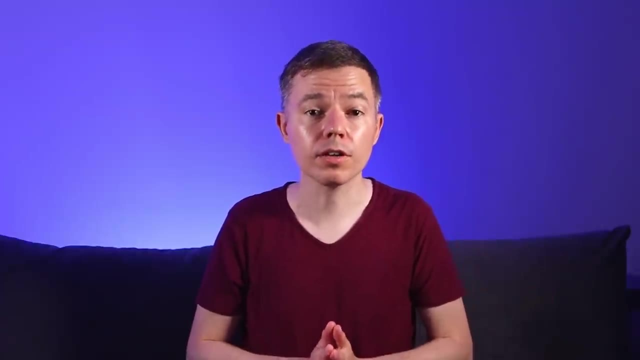 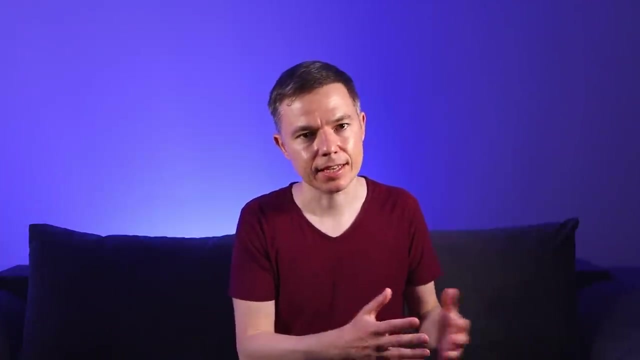 but what does it mean to create a risk response plan? First, it means that you come up with a specific action plan. Then someone needs to execute the plan. Moreover, they may need money and other resources to do that. So in essence, it means you need to add tasks. 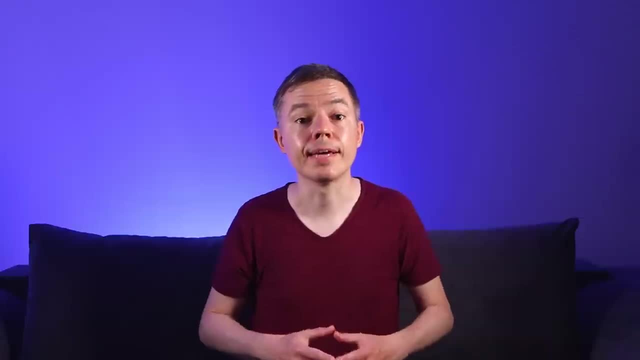 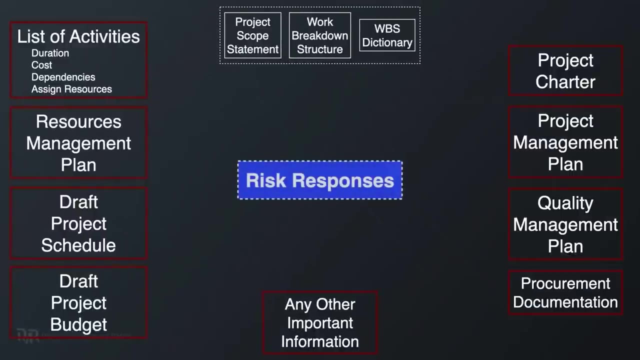 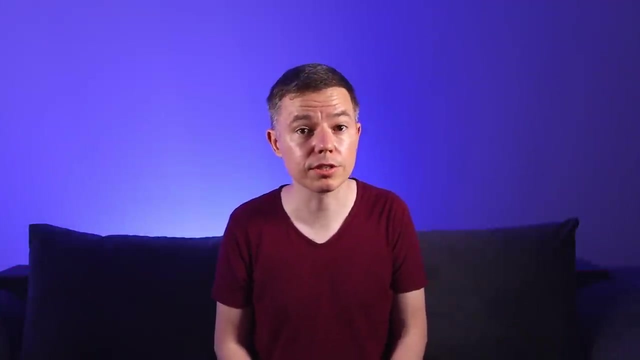 Also, you can allocate additional time or money to overcome negative effects of a risk, if it happens. So each risk response plan should become a part of the project scope, schedule and budget. By the way, sometimes you'll also introduce new processes and tools to overcome a risk or even a group of risks. 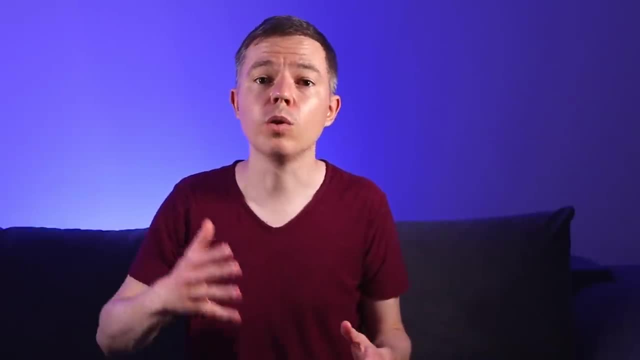 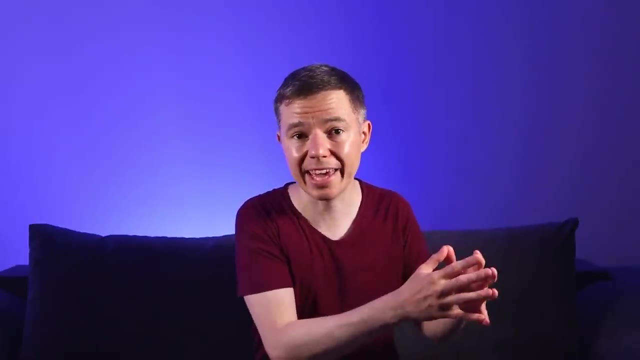 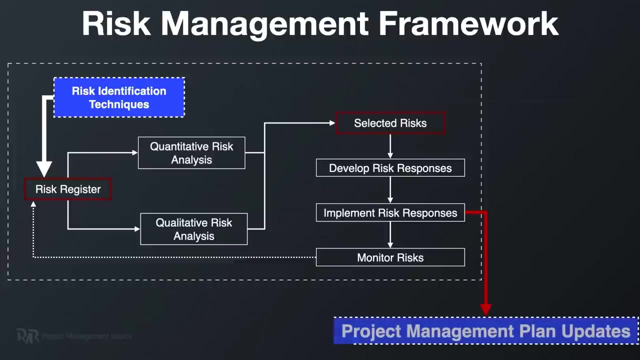 In this case, you must ensure that these new processes will work well with other processes and tools. Also, you need to ensure that stakeholders are okay with these changes. After all these updates to the project management plan, it will change. You need to validate that it's still working. 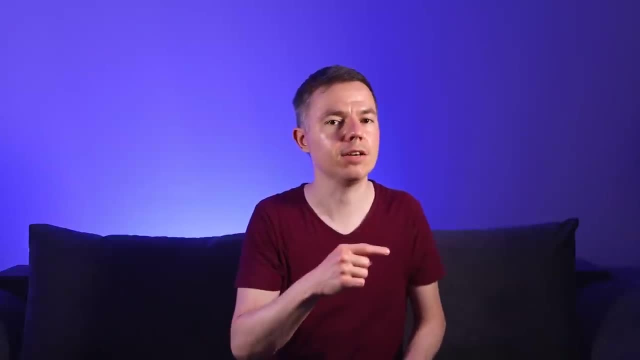 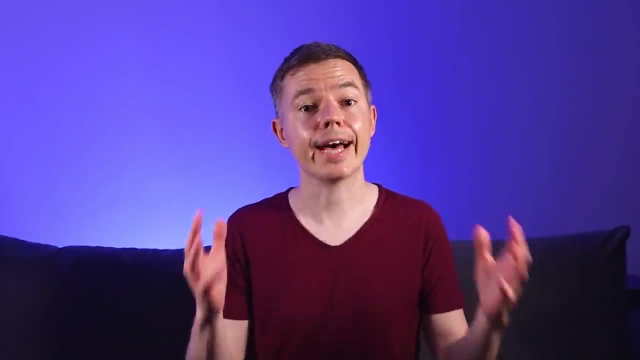 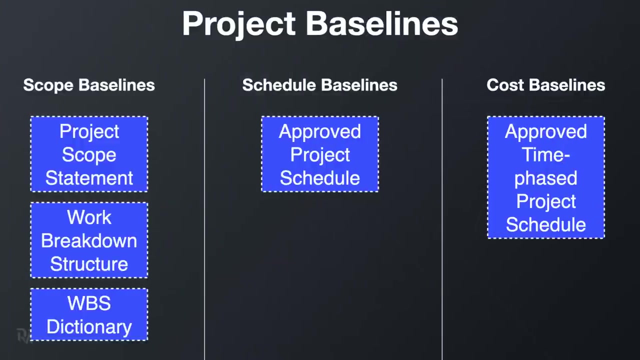 that it's still feasible. So you literally go to the beginning of the process and quickly run all the checks that we have discussed so far. All right, the last critical step here is to create project baselines. A baseline is nothing more than the final approved version. 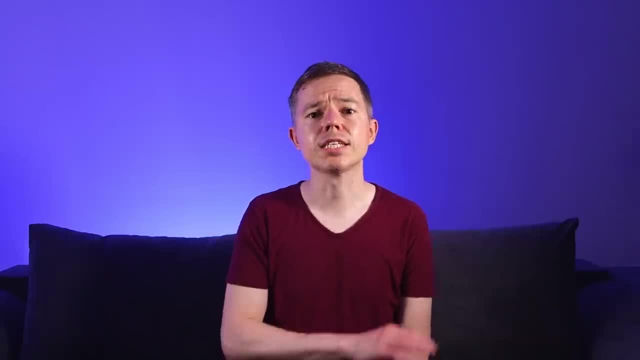 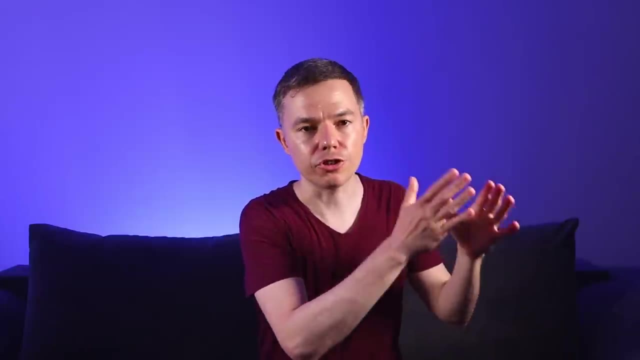 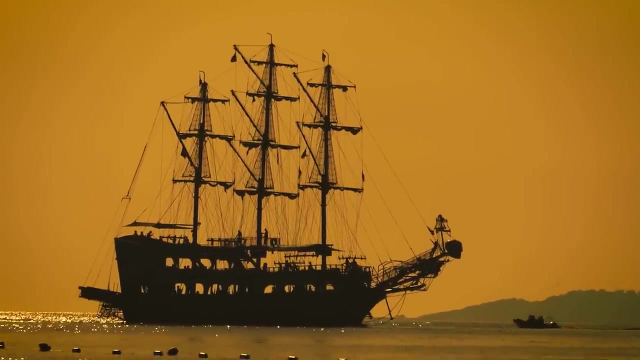 of project scope, schedule and budget. Baselines are critical for any project management approach. They will help you to track progress towards the initial goal. Let me try to explain the importance of this project management concept. Imagine you are a captain of a ship. 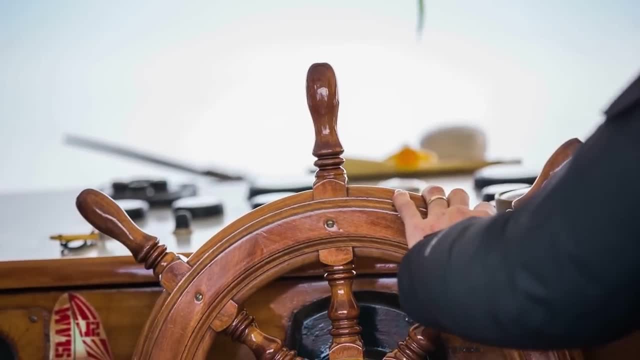 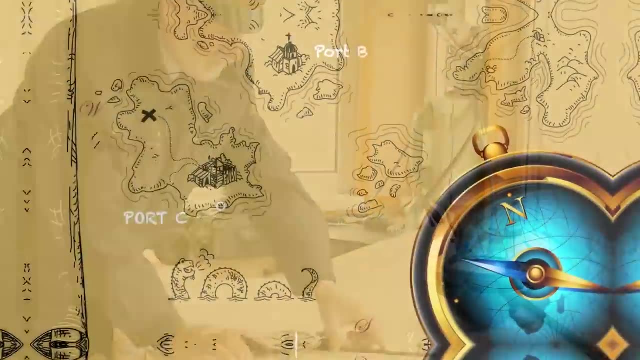 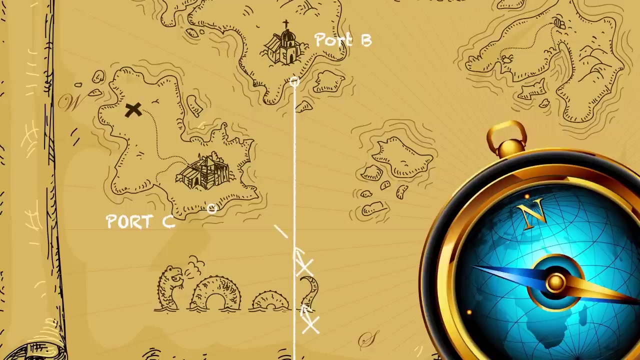 You need to sail from port A to port B. In the real world, a single vessel can leave a port without a plotted route. It's not allowed. The idea is that you have a plotted path and you continuously track your progress along this path. 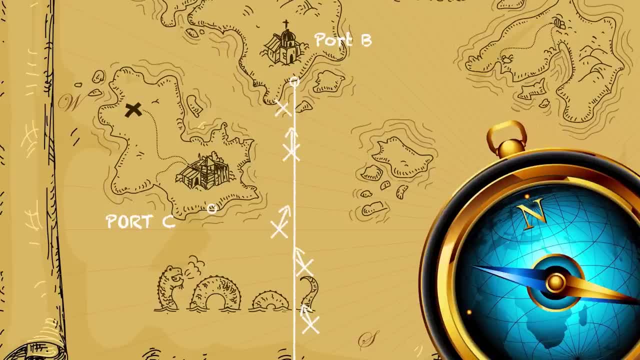 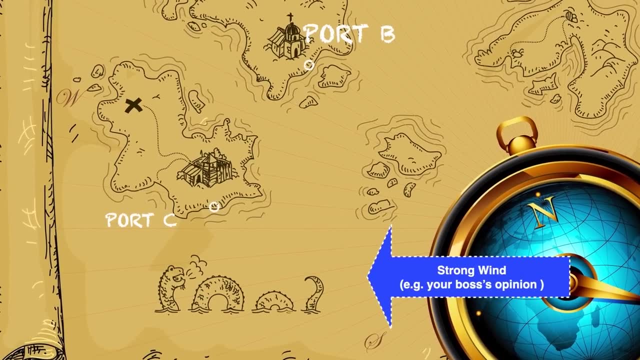 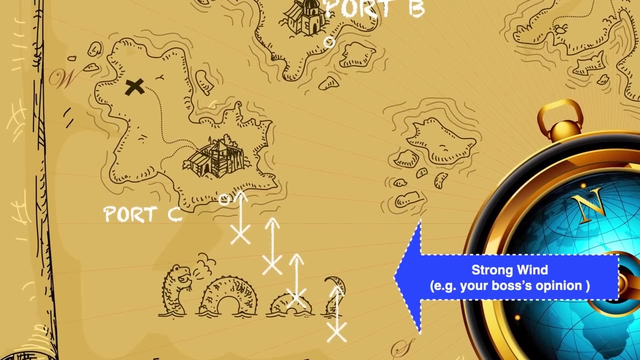 If you deviate from this path, you adjust course to get back to this line. You don't change the whole route. Now imagine you don't have this plotted path, You only have direction. In this example, even following straight north. 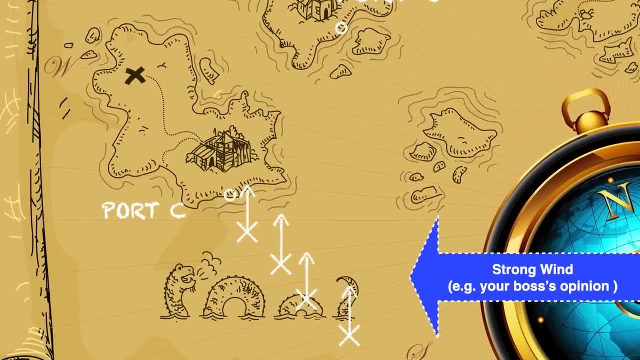 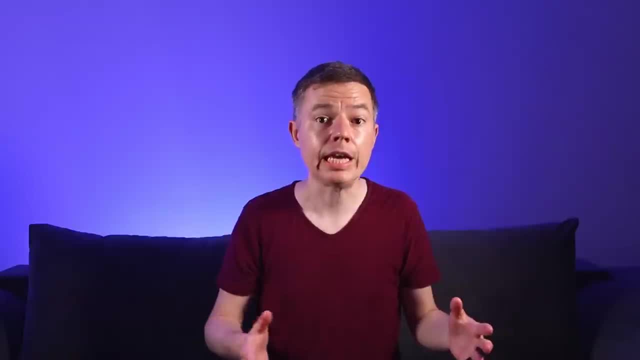 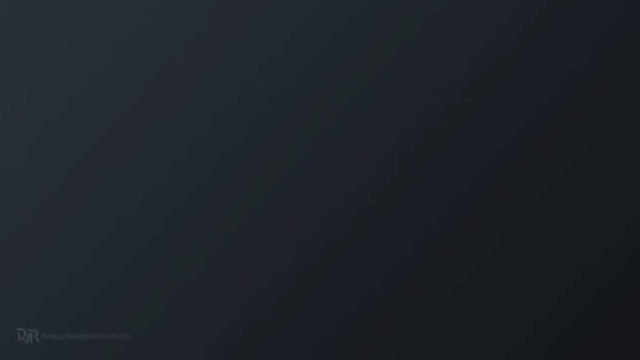 you may end up in a completely different port after a slight deviation. So I want you to remember that you don't merely manage the work on the project. You execute the project management plan you created. I can't stress enough how important it is. The plan gives you planned values. 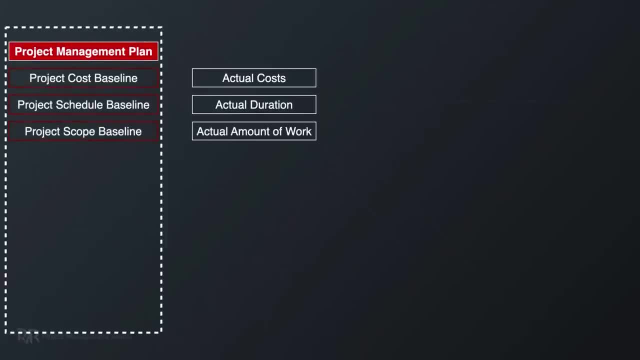 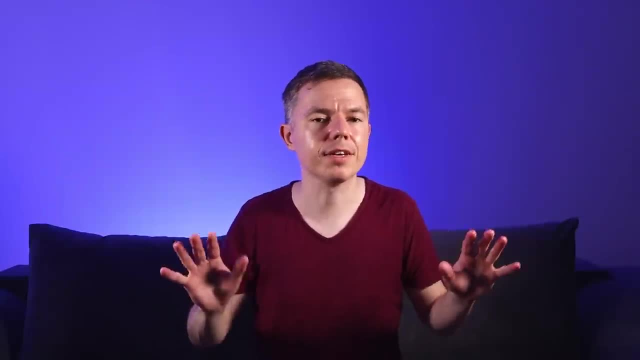 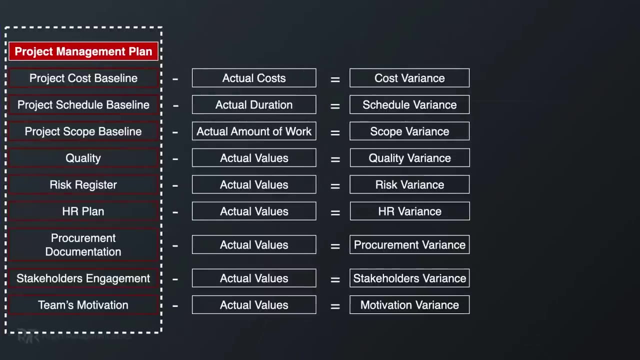 of all aspects of the project. Then, in the process of executing the project, you'll collect the actual values, And in the real world, nothing goes as planned. Now, if we talk about professional project management, you need to track all aspects of the project the same way. 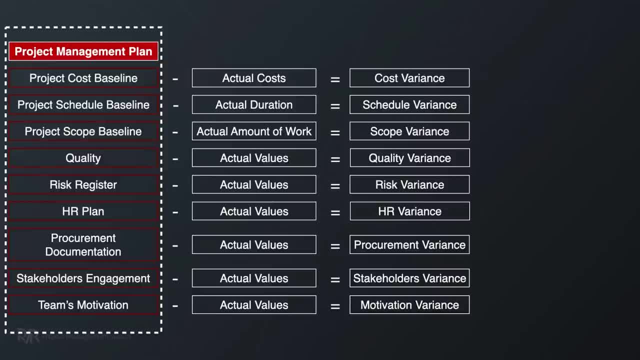 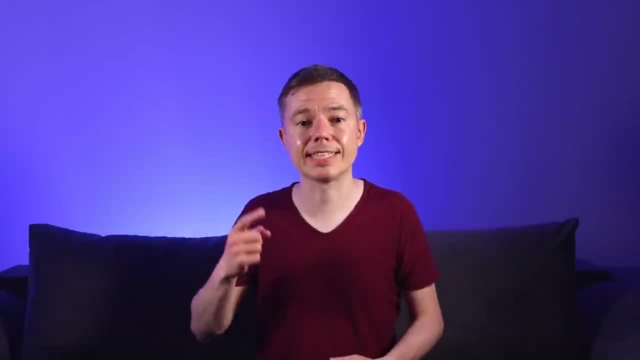 Quality communication, stakeholder engagement, motivation of the team, acquiring resources, everything. If you see deviation, you start applying productivity techniques, motivation, leadership tricks and maybe even a bit of micromanagement. to get back to the initial plan. 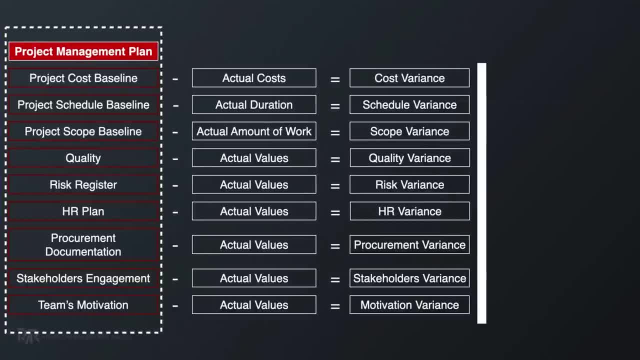 Only if the deviation is too big. you need to start negotiating to make a change in the project plan, specifically in project baselines. These are changes in deadlines, budget and scope of work. But you need to ensure that after these change, 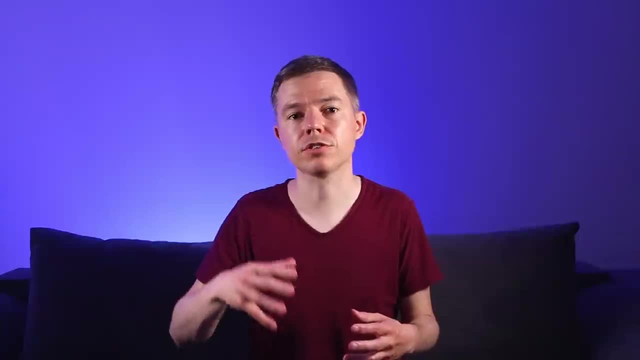 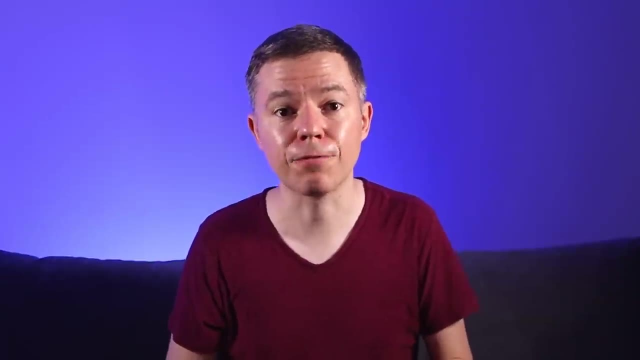 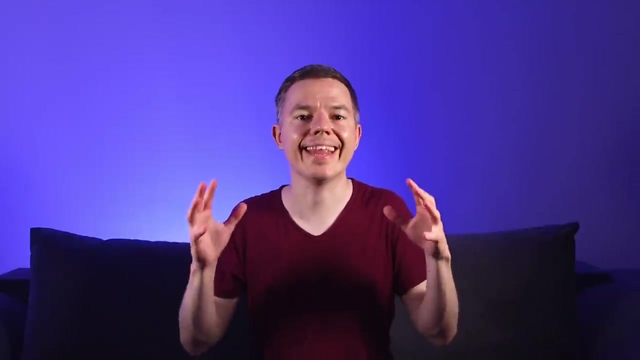 you take the action, But you need to take the action change. you'll be able to finish the project with the updated baselines and, most importantly, you won't be asking for another change request for the same problem in a week or two. Okay, finally, we are now getting into the execution of 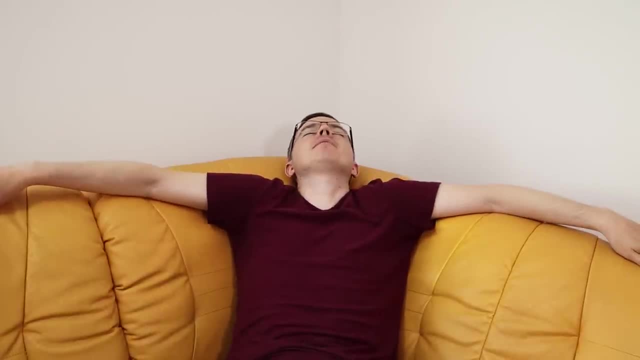 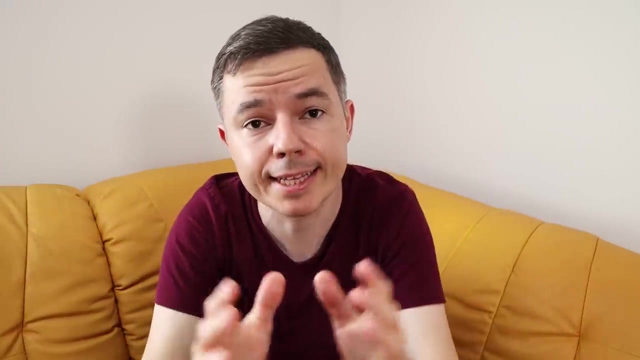 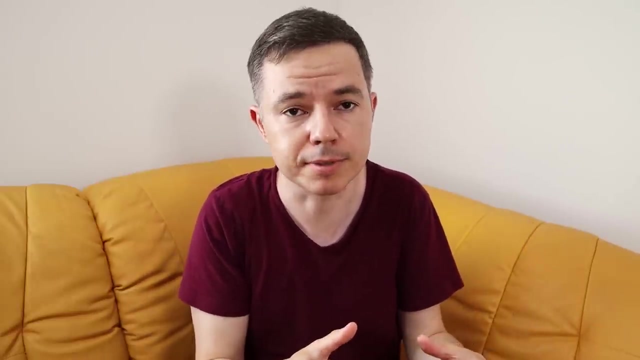 your project. I have finished planning the project, so it will go smoothly now. Now this project manager can take a rest, but for some reason I have a bad feeling. So, jokes aside, your project management plan simply outlines the work, but it doesn't have all the detailed instructions for technical problems. It 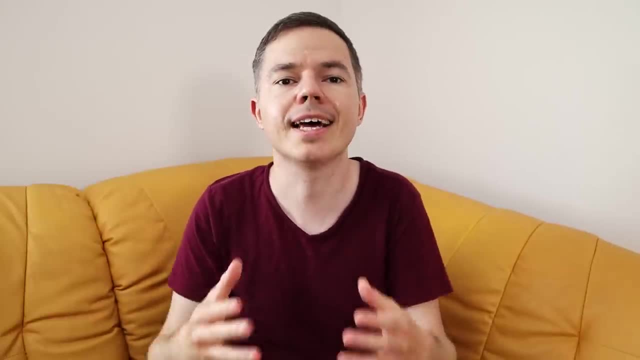 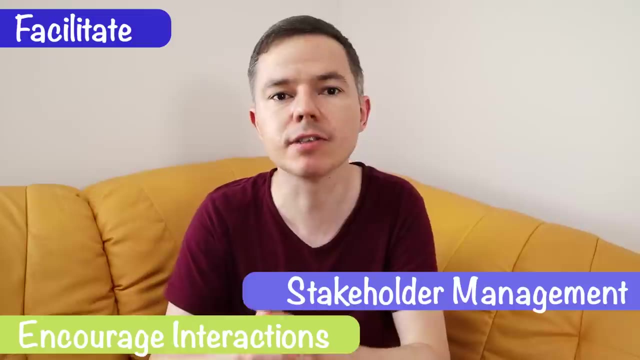 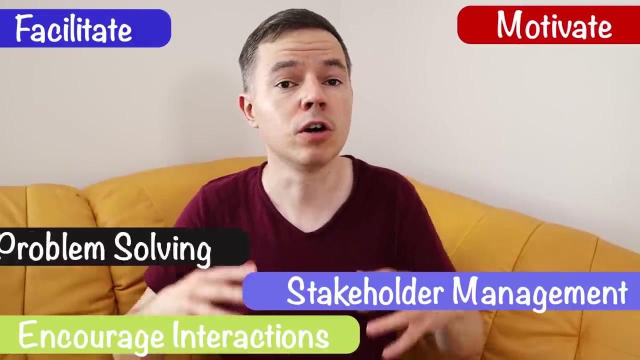 doesn't solve conflicts and, of course, your plan doesn't motivate people to act. So you need to encourage and facilitate interactions between team members, stakeholders and your project manager And subject matter experts on a daily basis. You need to motivate them to search for. 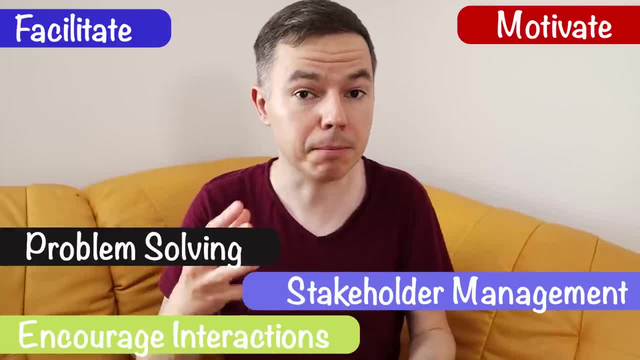 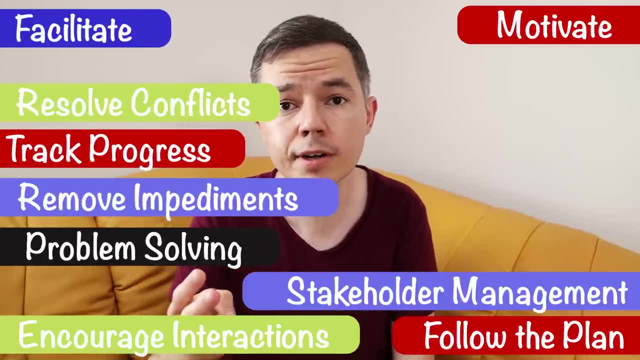 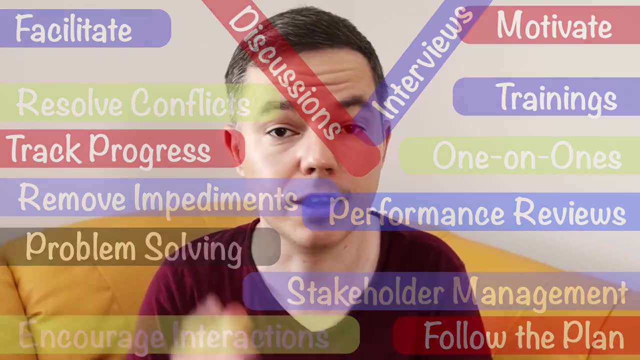 solutions to technical problems and implement them according to your project management plan. Then you need to resolve conflicts, remove impediments, track progress, interviews, performance reviews, one-on-one meetings, trainings, discussions and so on and on and on. All these activities transform into some. 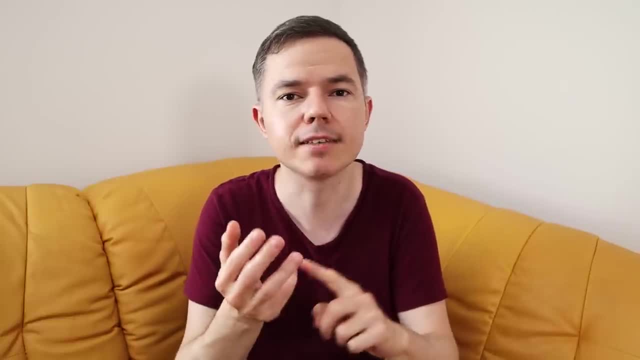 sort of communication. Most likely it will be a different type of communication. Most likely it will be a different type of communication. Most likely it will be a different type of communication. Most likely it will be additional meetings, emails, phone calls, documentation and things like that And overall. 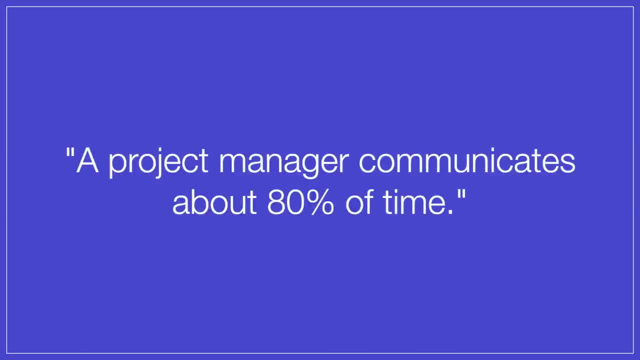 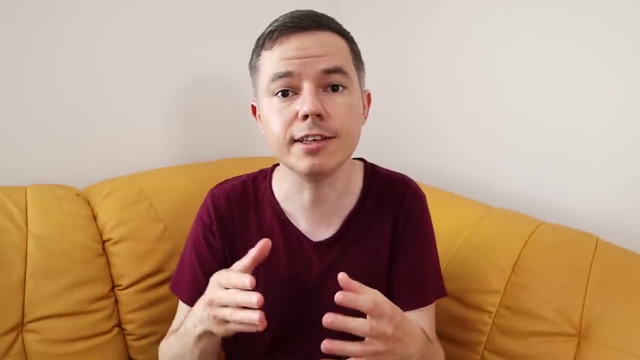 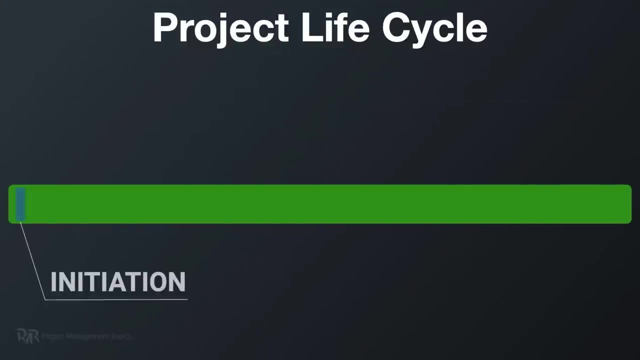 you will communicate about 80% of your workday, So your goal is to aber ensure that the team works on the task they need to work on today And, additionally, you look a few of the project is a daily grind. That is why I recommend. 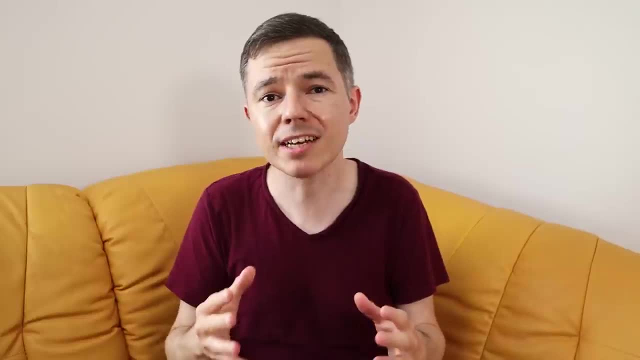 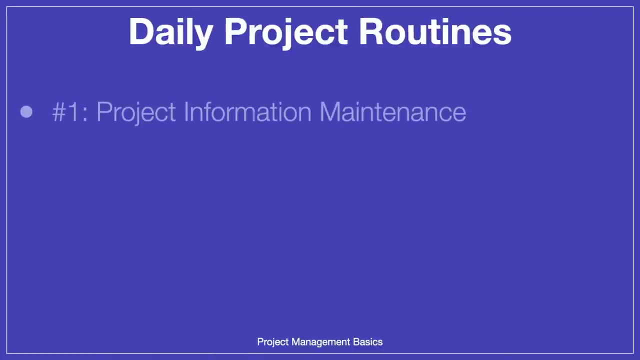 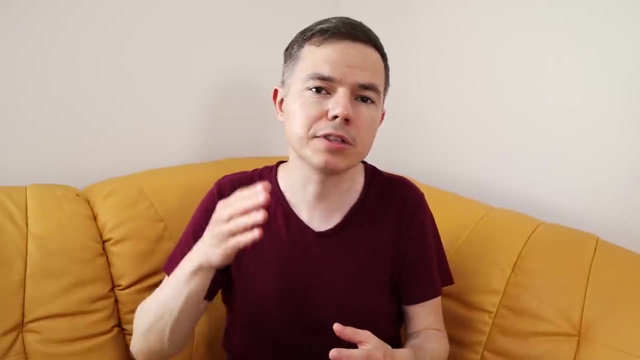 that you establish daily project routines. They will help you to keep your sanity and control over the project. So here are the routines I recommend to have. First of all, project information maintenance routine. You must dedicate up to half an hour a day to ensure that all team members report their progress. 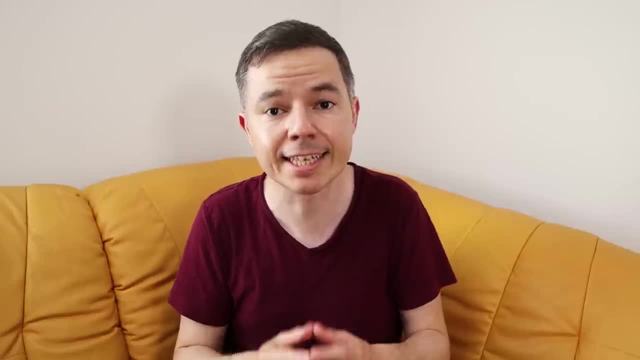 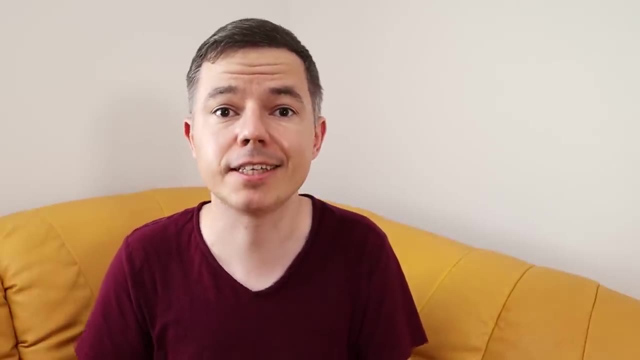 log their time, expenses, risks and other performance data in the project management software. It's better to do it daily rather than scramble all this information late in the Friday's evening when you need to send a progress report. Second, a daily sync up meeting with the team. 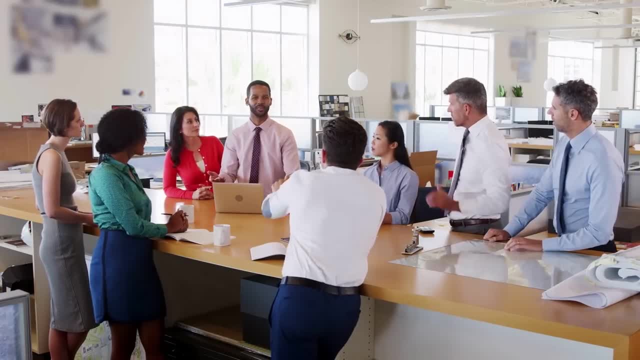 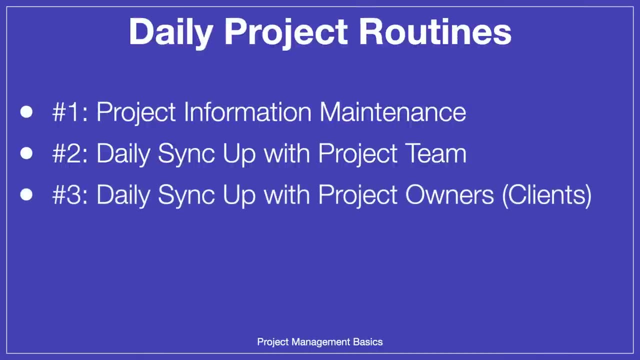 It's a short meeting where team members report on their daily progress and problems, And it's your opportunity to correct the team's work if needed. Third, daily sync up with clients and project owners. Ideally, you want to keep project owners up to date. 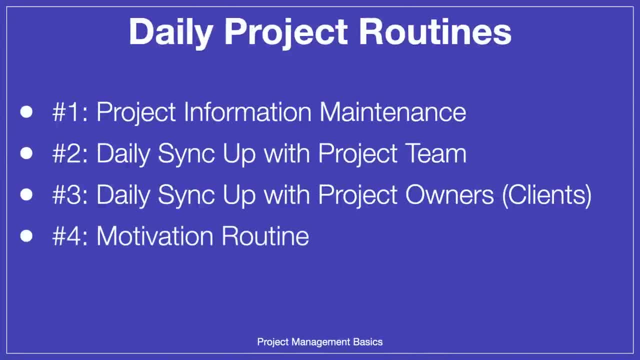 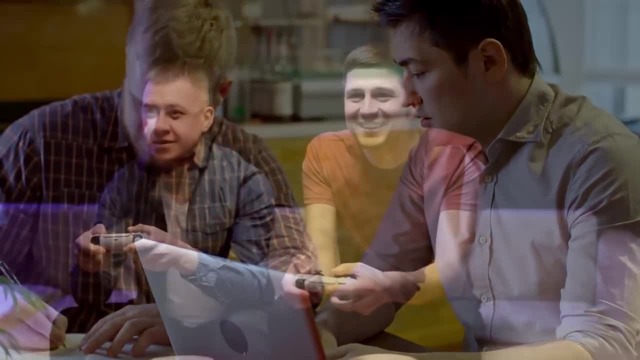 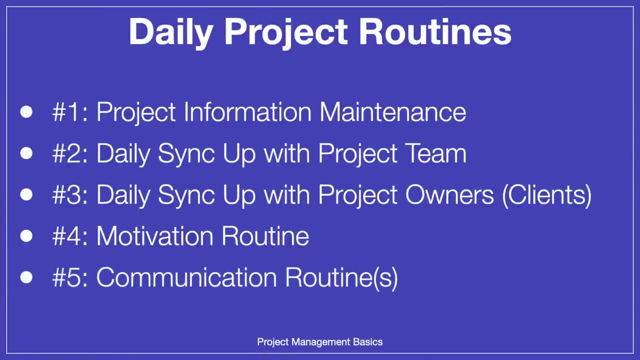 and engaged on daily basis. Fourth, daily motivation routine: Dedicate 30 minutes per day to motivate one or two team members. Don't wait for a special event to connect with these people. These small, meaningful interactions have a great effect. Fifth is the communication routine. 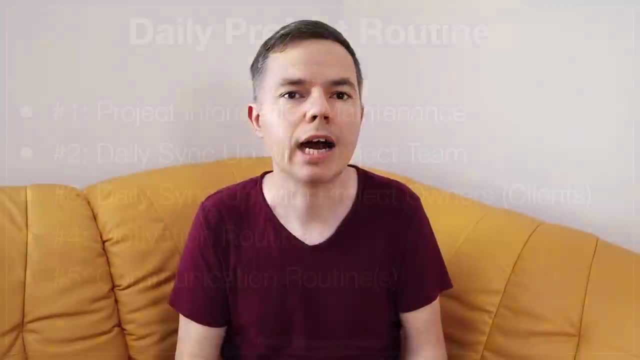 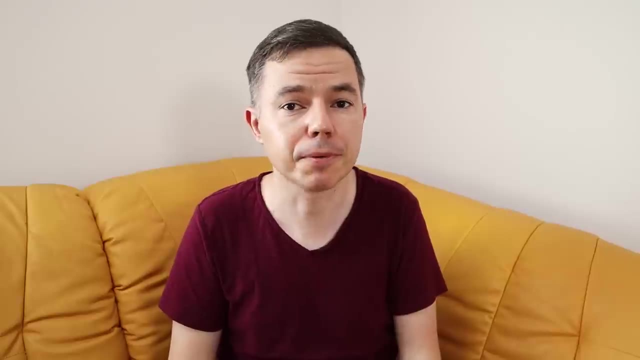 Specifically, I'm talking about writing emails and reports. I recommend that you reply to emails at specific times. Pick two, three or maybe four time slots per day and be intentional to clean up your inbox and answer all important emails. Thank you. 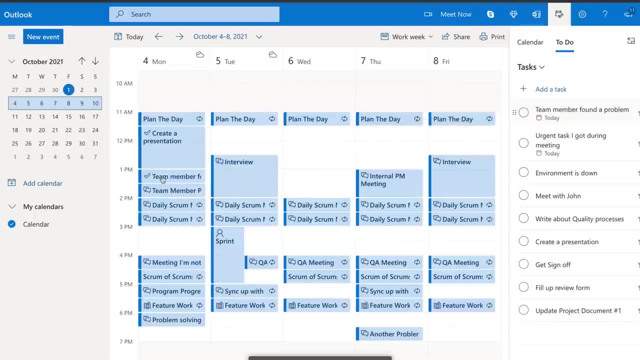 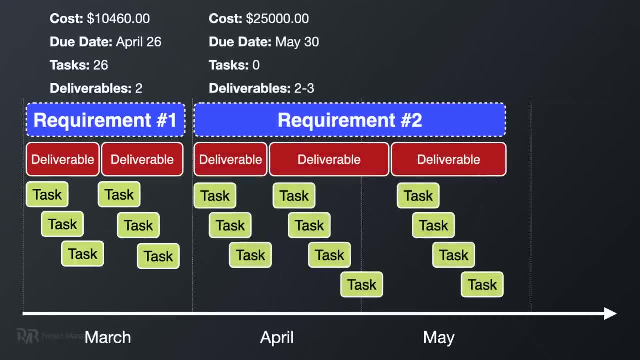 Also, you can put meetings in batches. It will give you free time slots for deep work. And again, remember that you must continuously dedicate time to rolling wave planning. You need to work with the team to collect requirements, decompose and estimate future tasks. 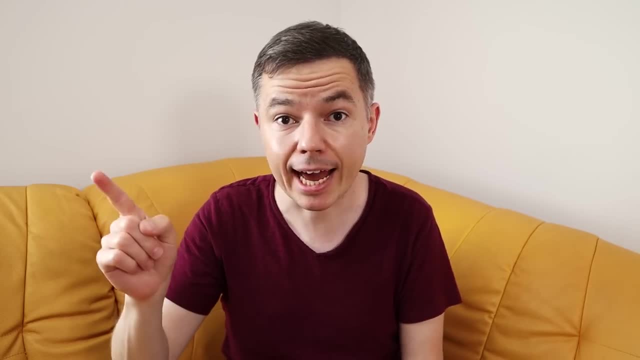 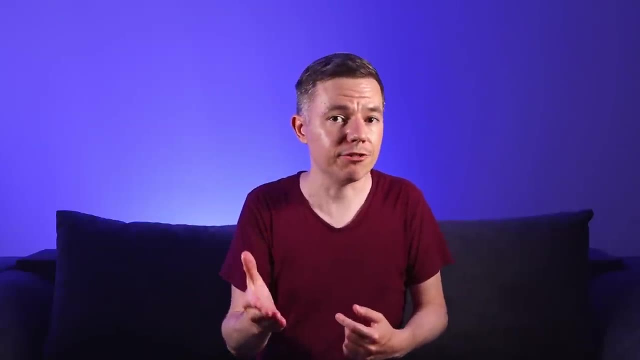 add details to your schedule and budget. Okay, let's get back. I have one more critical thing to share with you. So here's the problem as I see it In this video. I've just scratched the surface. You can try and see if you can do it. 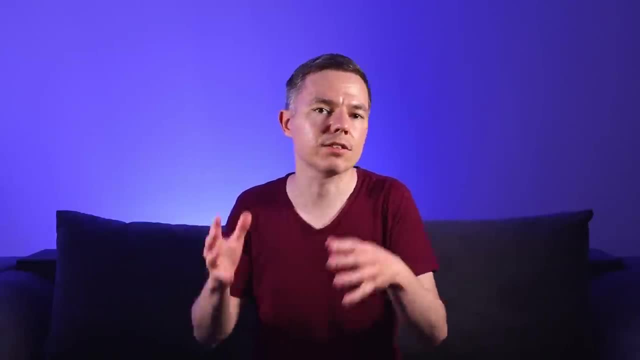 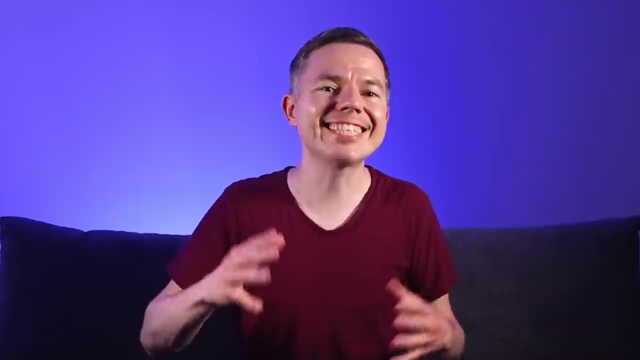 You can try and search all these processes, tools and techniques on YouTube, but then you still need to find a way to make it all work together as a whole. So instead, let me ask you this: Do you want me to explain this whole project management? 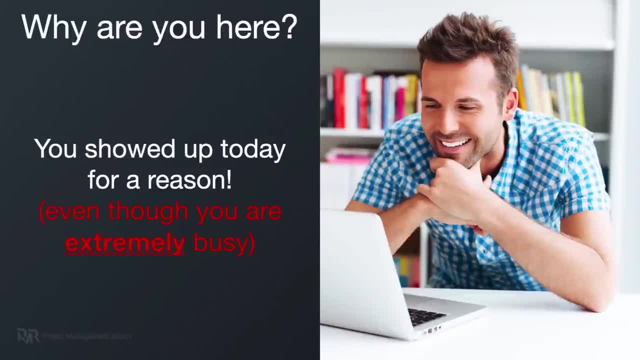 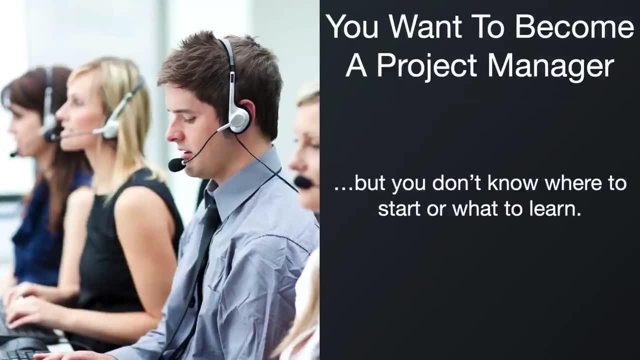 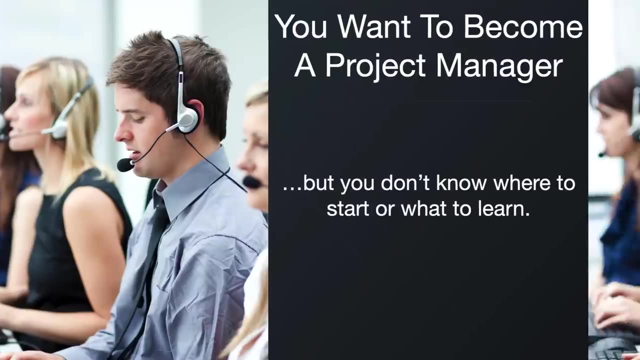 framework in all the details. I'm asking because you watch this long video even though you are extremely busy. for a reason Maybe you want to become a project manager, but you don't know where to start, what to learn and how to get your first project management job. 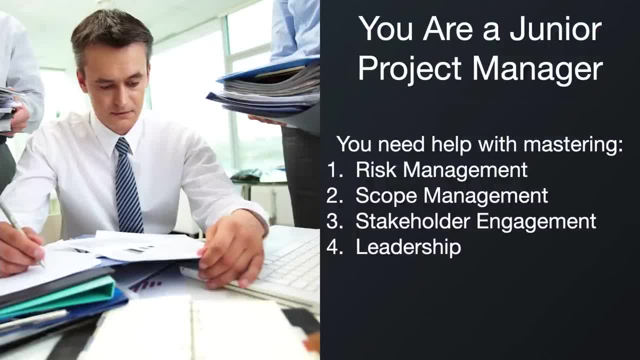 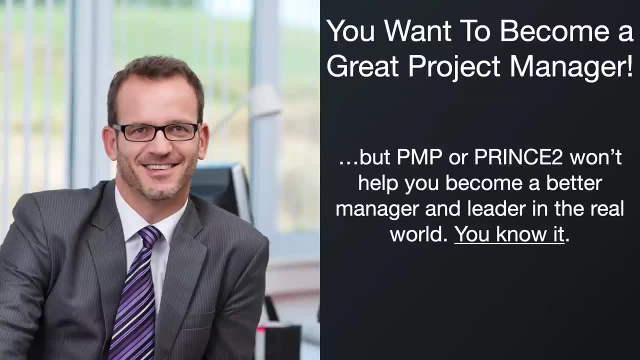 Or you are a junior project manager who struggles with mastering all these risk management, leadership, stakeholders and how to manage an experienced team. Or maybe you are a mid-level PM already and you want to become a great project manager and leader, but you already know that PMP or PRINCE2. 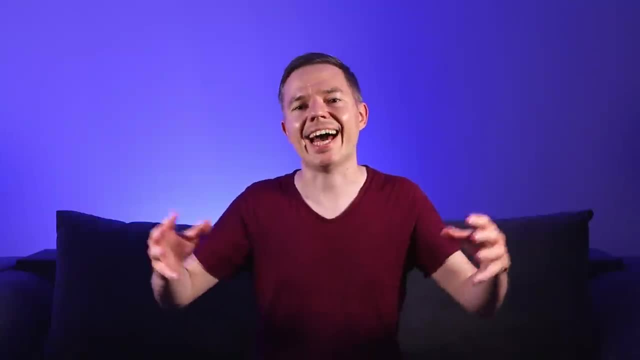 won't help you in the real world. In any case, as I see it, you have only two options here. You can start with the first one, and then you can start with the second one, And then you can start with the third one. 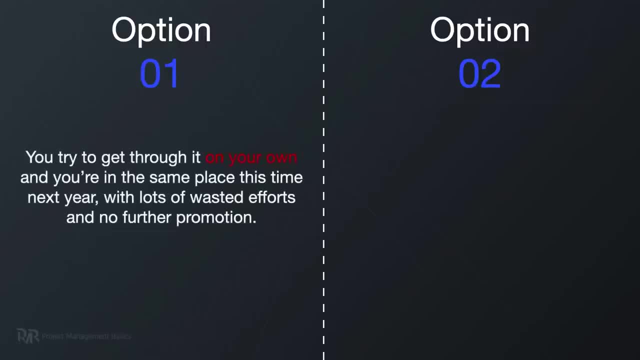 There are two options here. Number one: you try to get through it on your own and you are in the same place this time next year with lots of wasted effort and no further promotion. And option number two: you 100% commit to mastering practical project management framework. 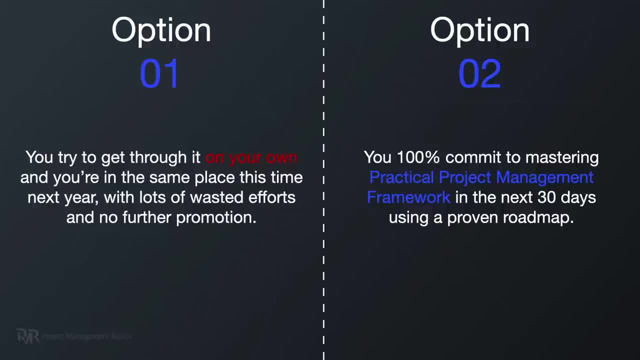 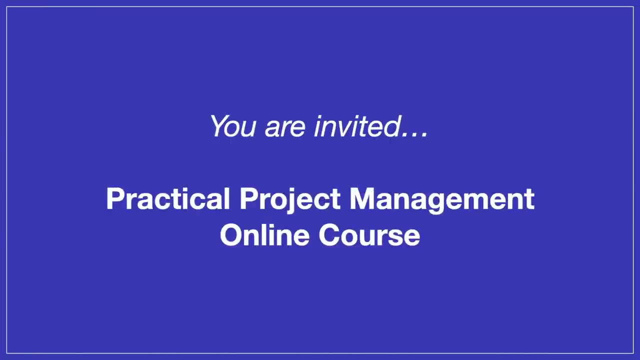 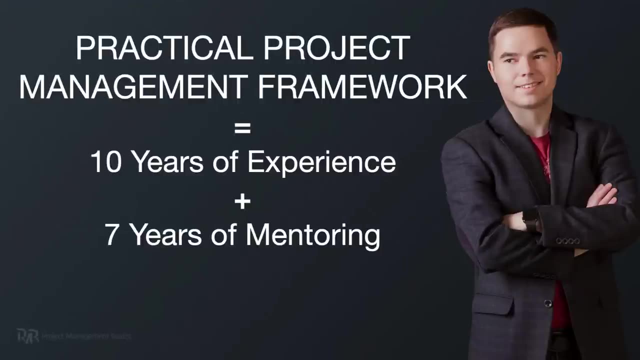 in the next 30 days, using a proven roadmap. You're going to make this decision right now. That's why I'm so excited to let you know that my practical project management online course is exactly what you need. I've used my 10 years of experience. 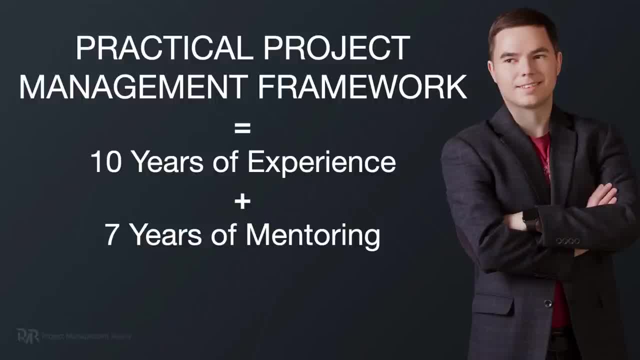 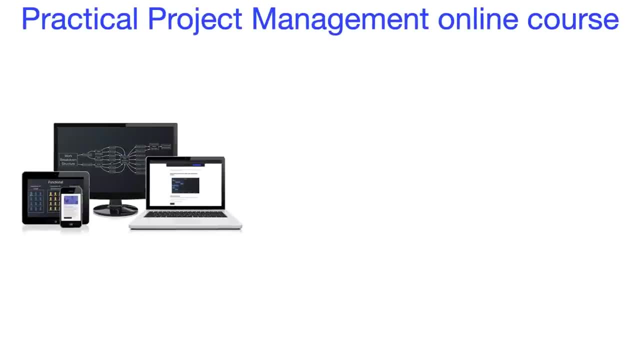 as a software project manager and created a framework that anyone can use in the real world. Hundreds of students proved that. As a result, you get a comprehensive course on project management with about 15 hours of educational videos like this one, but broken down into smaller, digestible pieces. 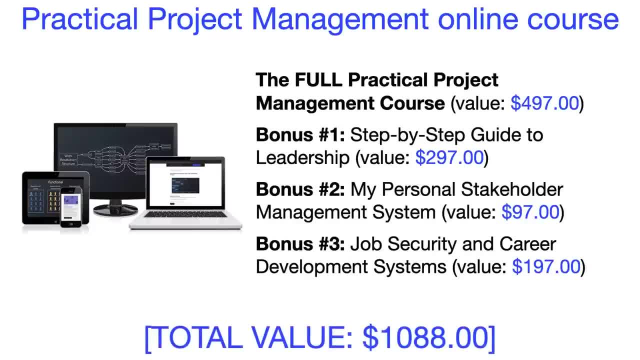 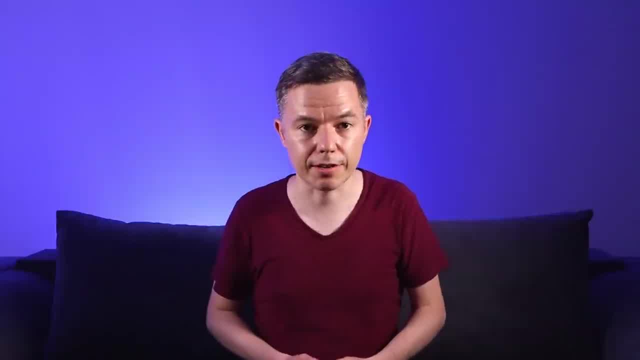 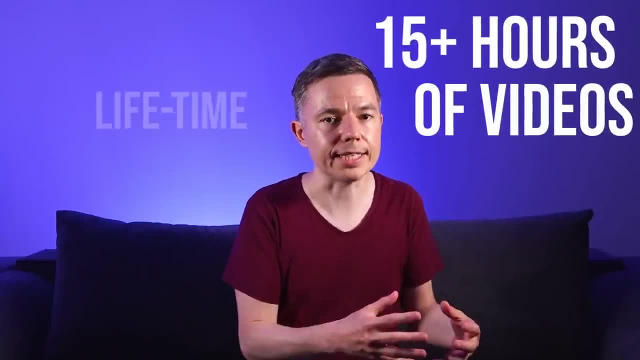 And all these videos cover all the details that we outlined today. It literally contains everything you need to know about project management for the rest of your career, And the best thing about this course is that you get lifetime access. It means you can learn at your own pace. 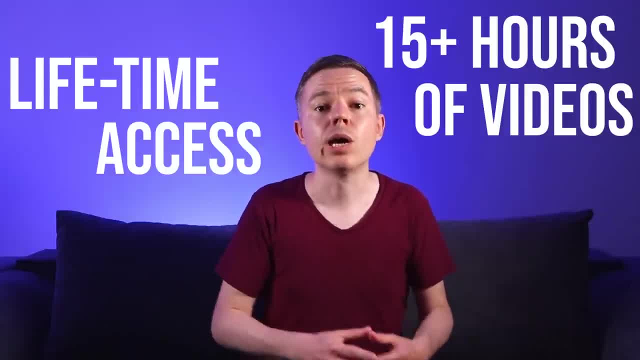 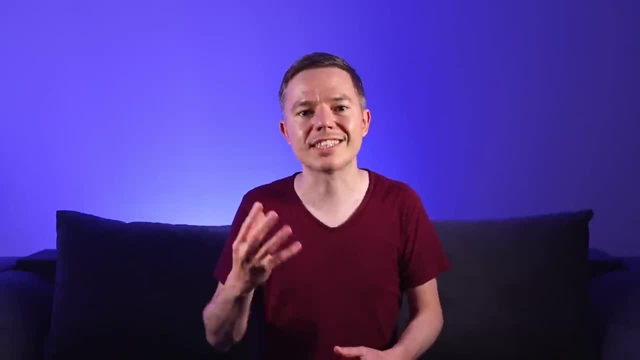 but also it means you can get back to the course whenever you need to refresh your knowledge, Because your career will get a serious boost. You will start running more significantly and you will be able to do more things, And I know you might be thinking right now. 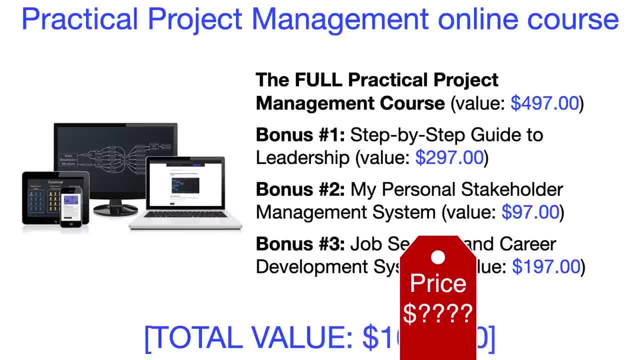 okay, Dmytro, that's a unique and profound course. Show me what I need to pay for it, And actually I might have charged you $1,000.. The program is that good. There is a lot of value that you don't get. 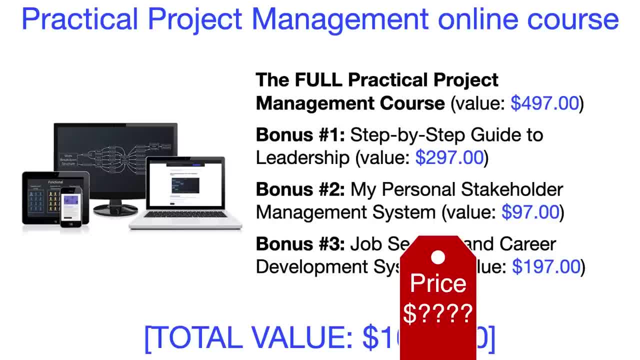 from any other online course because this one comes from my practical experience, not from theory. But I am really passionate about my profession. I believe that if I train myself, there will be one more great leader in the world, So I made the course as affordable as possible.